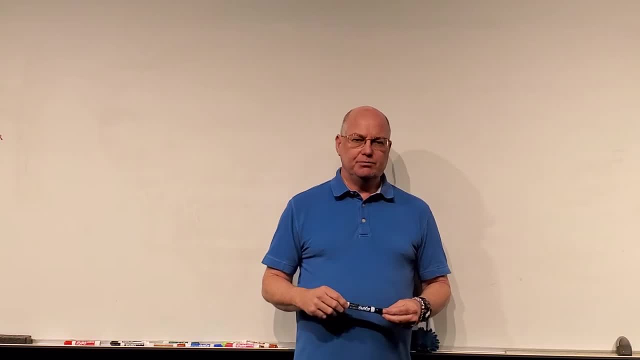 wants you to know more detail or cover some different things, then please know what your instructor wants you to know. Finally, these videos are done pretty crudely. It's just me, a camera and a board and I do them pretty rapidly, usually under a lot of duress, because 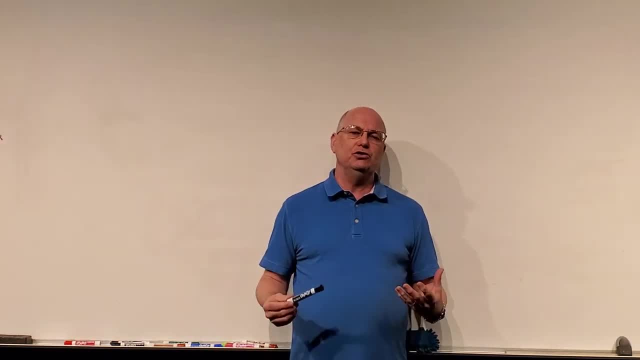 I'm trying to get them out under these circumstances for my students to use under this COVID protocol. Hopefully soon we'll go back to face-to-face classes and then I'll reshoot these videos for use by my students, Thank you, But they'll be much neater and more professionally done. So bear with me if I stumble or mutter while 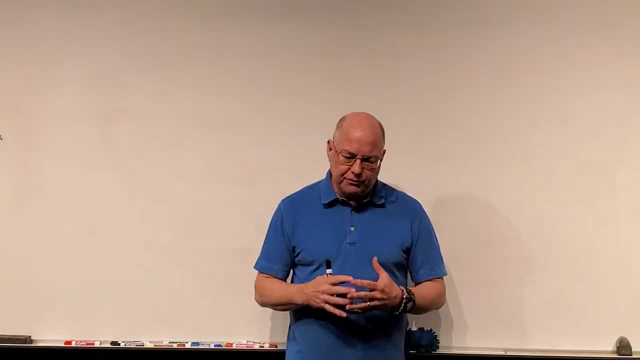 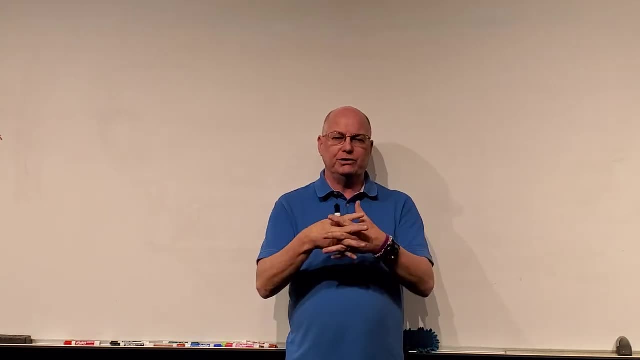 I'm thinking my way through what I want you to know Now, what we've been covering in class. this video really is intended to tie some things from our lecture course and our laboratory course together. There's a lot of information in microbiology and it's really hard to teach all. 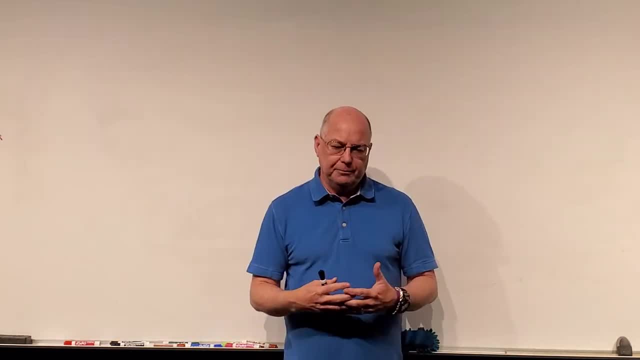 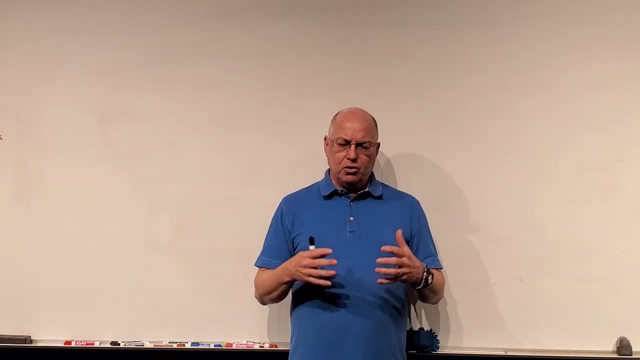 this stuff in 16 weeks with any great depth. There's just so much to know, which makes the class really really hard. Now my goal is to try to tie some things together in this lecture to make sense of why do we need to know certain things. One of the topics we covered was microbial metabolism. How do microbes convert? 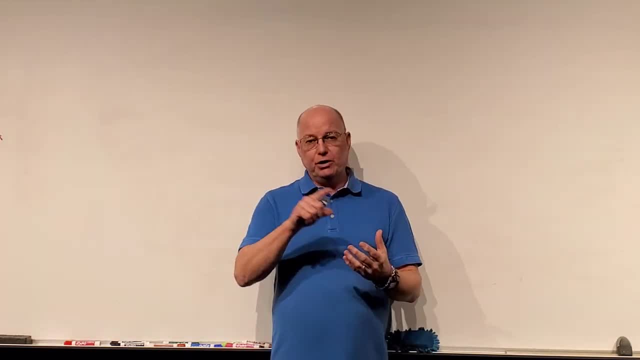 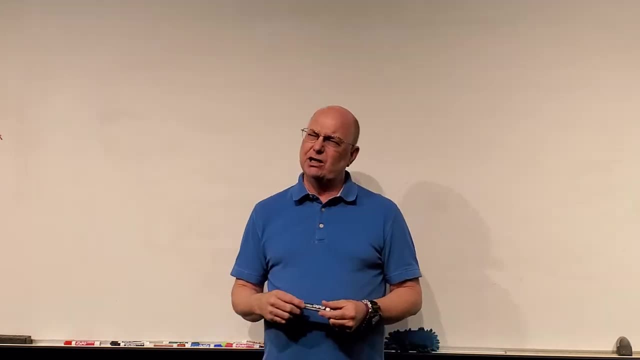 sugars into energy, and do they do it aerobically or anaerobically? And we've covered all the details of that, or some of the details of that, in a previous lecture, I think, when we did chapter five- I don't know exactly which chapter it is, I don't have the chapters memorized- But we talked 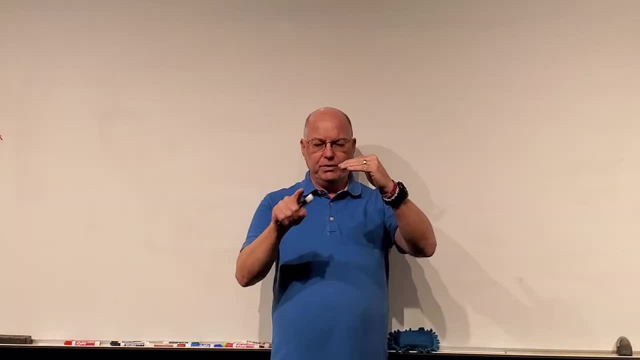 about how we go from glucose to pyruvate and then from pyruvate we could go through the Krebs cycle, make more ATP and then electron transport. We're going to review some of that. Our goal is not to follow the energy, though. It's to understand. why do we do some of the biochemical tests? 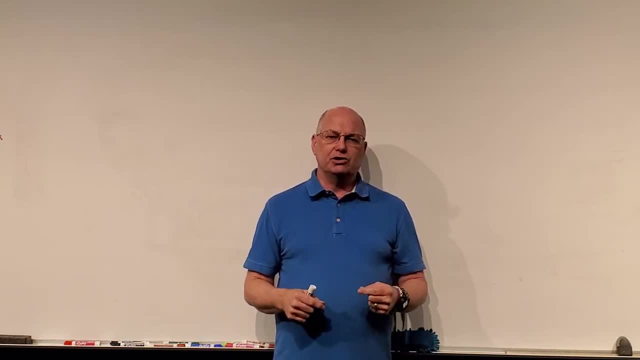 that we do in the laboratory. Biochemical tests use some chemistry and our knowledge of microbial metabolism to help us design some tests to detect which bacterium is present, based on what we know about their biochemistry. So I'm going to go into some more detail into this. But what we do know is that almost all living organisms can take glucose and turn it into pyruvate for energy. Since bacteria don't need a lot of energy, they could stop there. Some do have the enzymes to continue with the Krebs cycle and electron transport. Some do not. 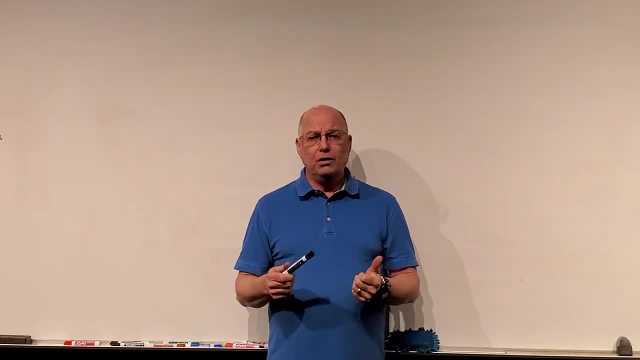 have those enzymes and don't have the capability, or if we deprive them of oxygen, they can go through another pathway and do what we call fermentation. Fermentation will produce some acid byproducts in most instances And of course we can use some pH indicators to see color change when the pH 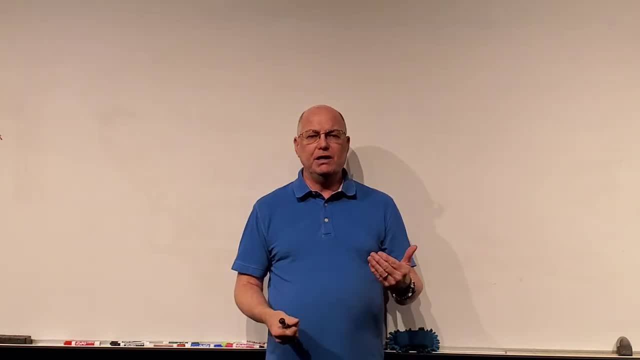 changes. So if a lot of acid is produced, then a certain pH indicator will turn yellow or red and tell us acid is being produced. Therefore we can deduce that that bacterium has done fermentation under anaerobic conditions We can take advantage of. 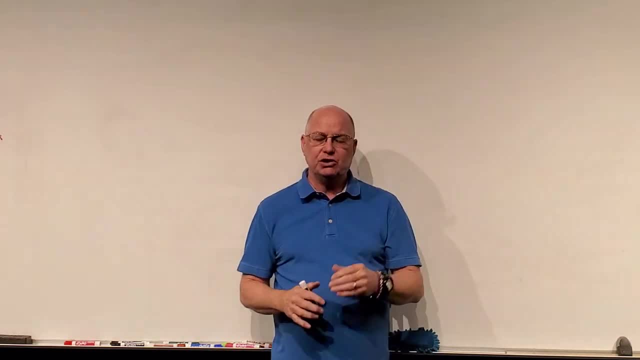 this and create a battery or series of tests so that when you have some unknown bacterium- you have a patient with an infection- we can run it through a series of tests and figure out which particular bacterium is causing the infection. That becomes important because, as 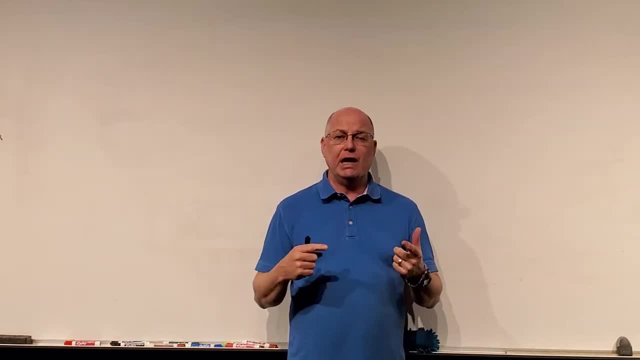 you know what we've done in lab. we've done our antimicrobial agents and antibiotic agents. Some antibiotics are more effective against certain bacteria and not others. So knowing which bacterium is present helps us to know which bacterium is present and which bacterium is not. 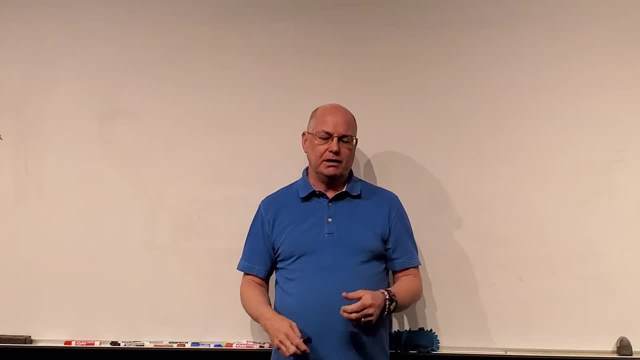 This helps you determine the path of treatment, the mode of treatment, which antibiotic agent would be used. Also in lab we did serial dilutions and microbial counts. The microbial count can give you an idea as to how severe the infection is and therefore what kind of dosages or how long to. 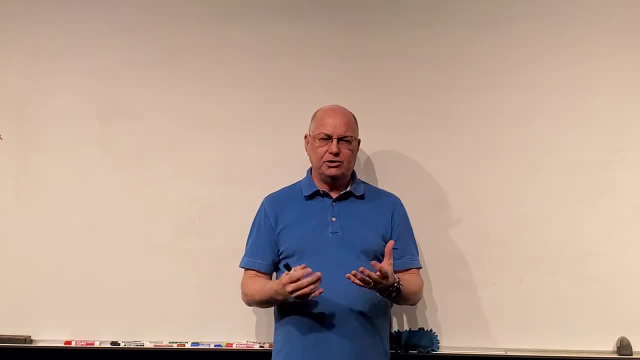 take a certain antibiotic. So we can use all of this information to figure out which microbe is causing our pathology and then determine what is the best treatment protocols in order to treat. that is why certain medications are given. Why do you get biaxin and not, you know, clindamycin or something? And why does this patient take 250 milligrams of biaxin instead of 500, or vice versa? Why do you get it for seven days one time, 10 days, another, 14 days, another? And that depends on the severity of the infection. which antibiotic is chosen based on which microbes are susceptible. 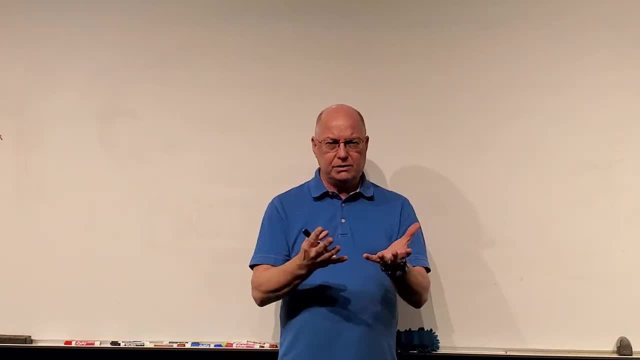 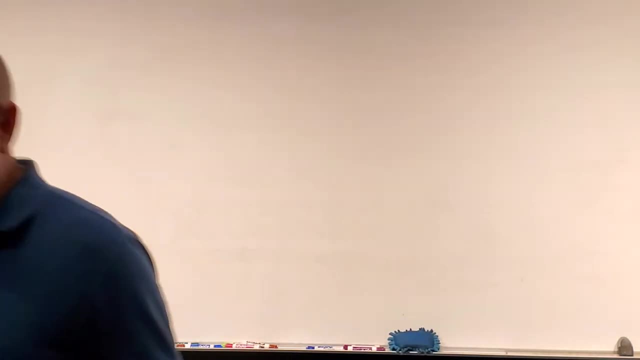 to that antibiotic. We've done a lot of that in lab. Now we're going to try to tie some things together. So let me review microbial metabolism briefly. Let me see exactly where I can see on the board. so I'm somewhat in the center of the screen. Yeah, that's about perfect, Okay, so 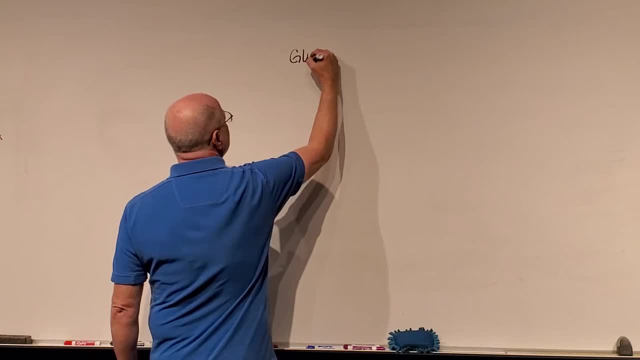 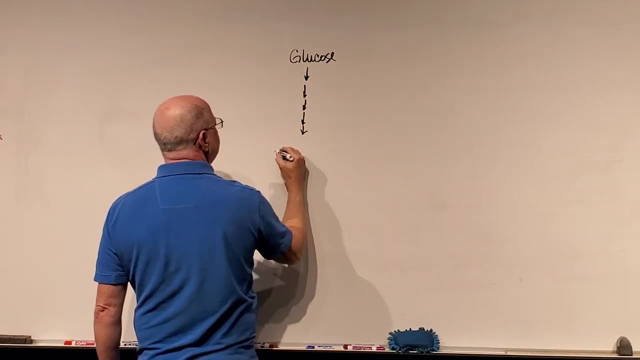 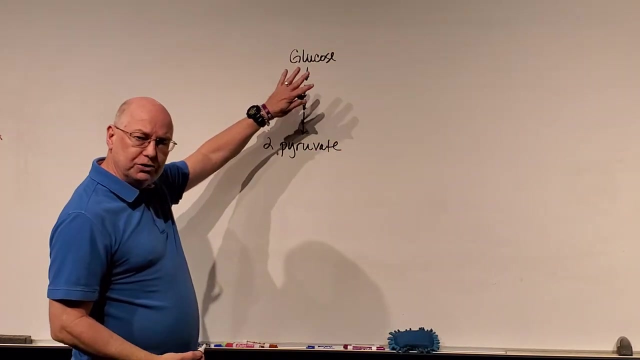 we know that almost all living organisms in their cytoplasm can take glucose, a six-carbon sugar, run it through a series of reactions and we get two molecules of what we call pyruvate or pyruvic acid. This occurs in almost all life forms. 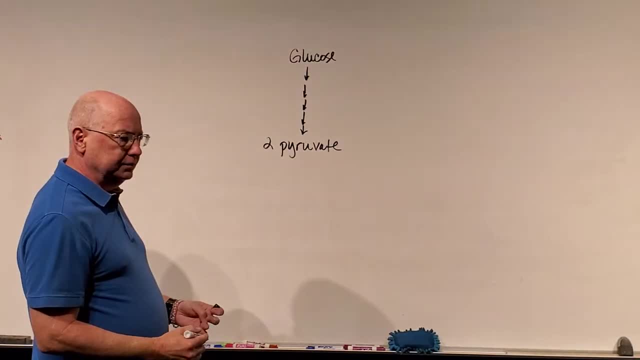 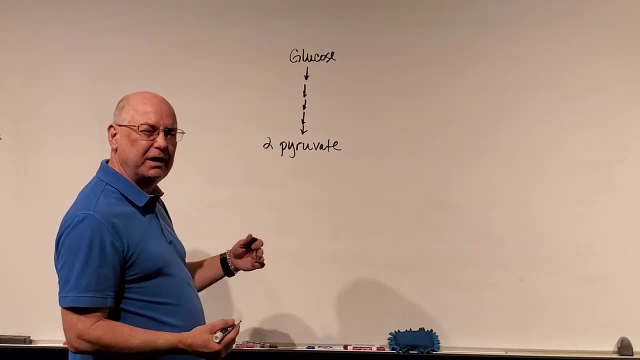 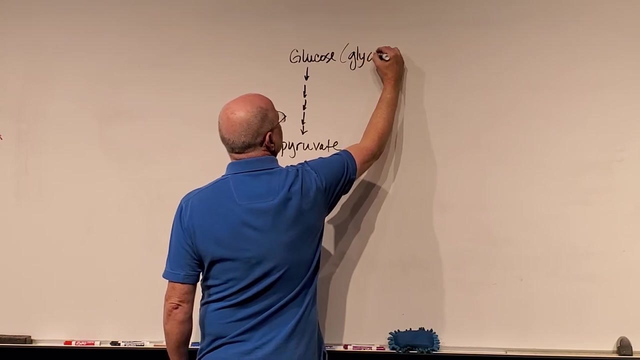 except for some that don't use glucose or you know. well, that's obvious. but chemiototrophs, So things that there's a few sulfur bacteria and things like that, but we're not going to worry about those. This process, by the way, is called glycolysis. 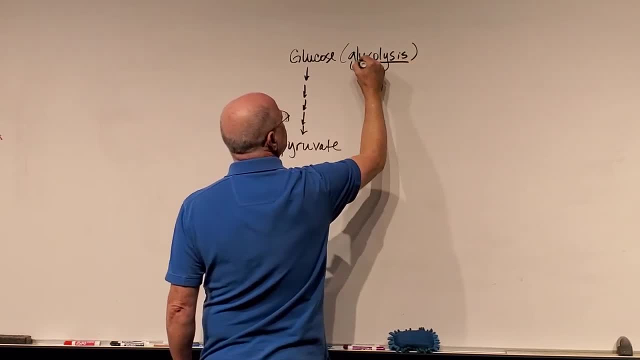 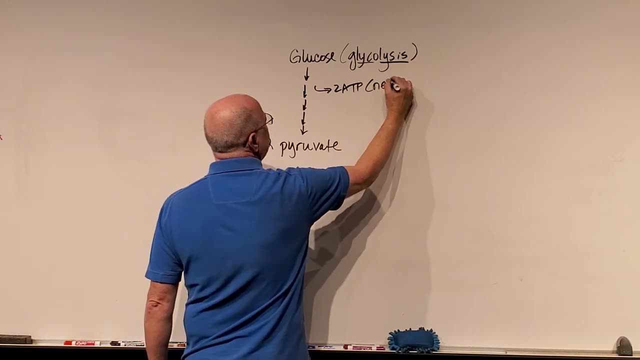 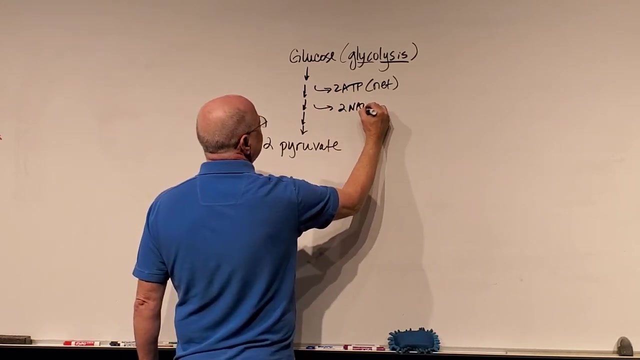 which literally means the lysis of a sugar. Now one of the things we get out of it is we get 2-ATP. That is a net gain of 2-ATP. You know, we gross 4, but it takes 2.. And then we get some molecules called NADH, which are 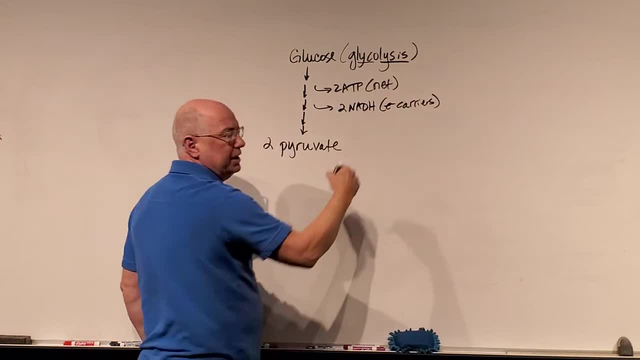 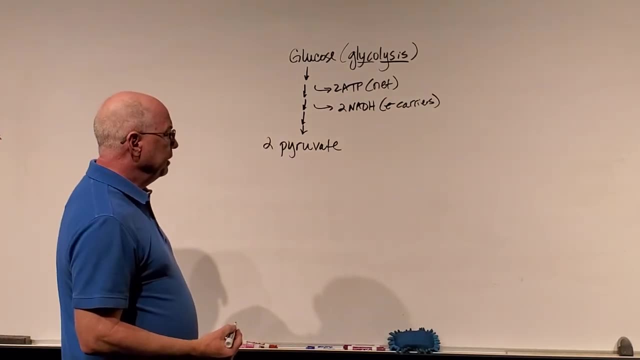 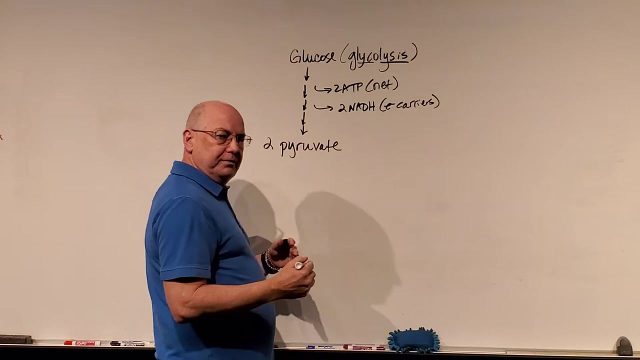 electron carriers. Now, right now I really don't care about that. We're not interested in that part, because that's, we did that with microbial metabolism. But I am interested in this next part and you'll see why in a second. okay, Now, if the bacterium does not have the enzymes to do. the next step. that's where it ends for the most part. If it does have the enzymes in its cytoplasm or associated membranes in some instances, then pyruvate gets converted to a stuff called acetyl coenzyme A, also called acetyl-CoA I. 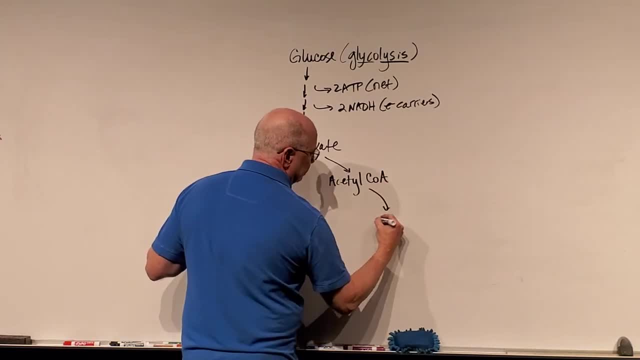 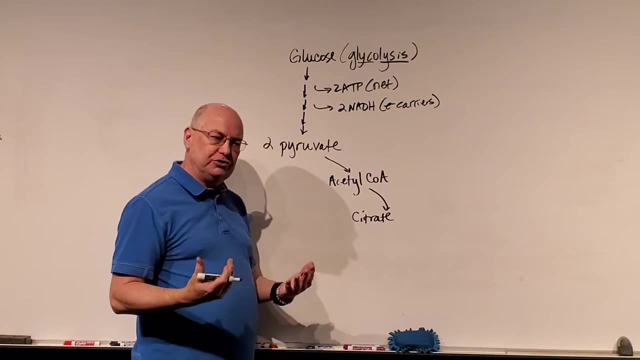 don't really care that. you know that one. The next step in the process is that can be converted to a stuff called citrate or citric acid. This is why orange juice and citrus fruits provide a lot of energy If someone has the glucose shakes and they don't have enough blood sugar. 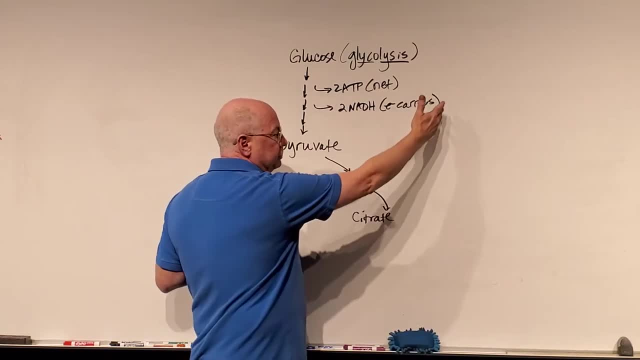 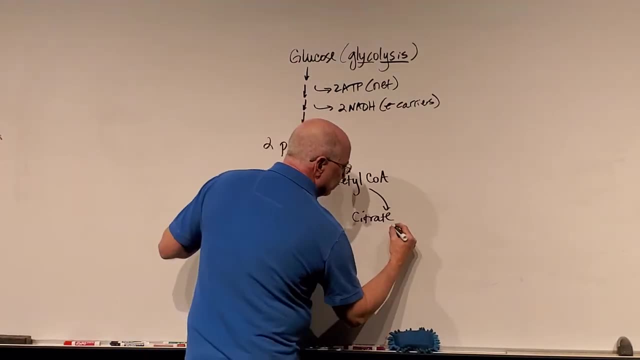 you can raise their blood sugar pretty quickly or their energy levels to prevent that, by feeding them orange juice and skipping some sit-ups, although there is glucose in orange juice as well. Okay, citrate gets converted to another stuff called isocitrate, which is just another form. 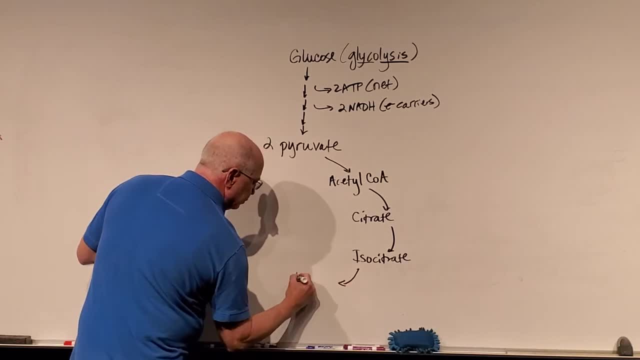 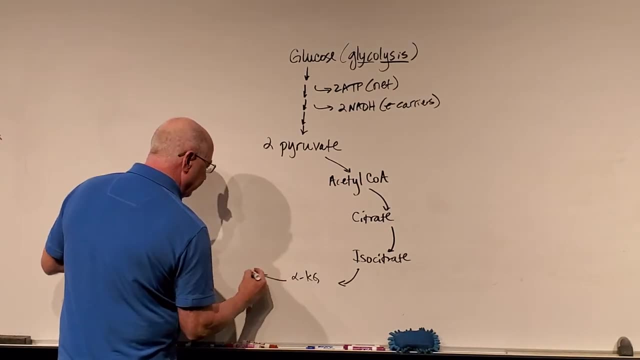 of it an isomer and then that gets converted to a stuff called alpha-ketoglutarate. I'm just- I'm not gonna write the name out, but alpha-ketoglutarate That gets converted to a stuff called succinyl-CoA, succinyl-CoA, succinyl-CoA, And the next step in the process is: that can be. 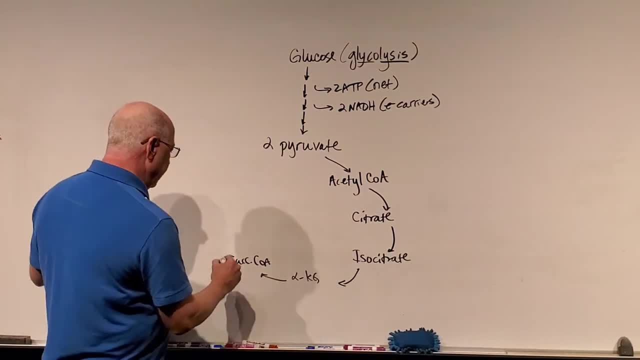 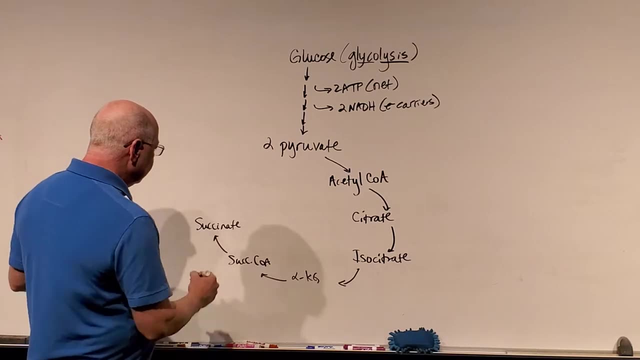 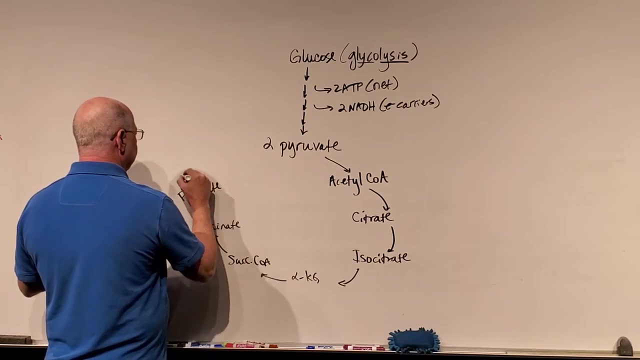 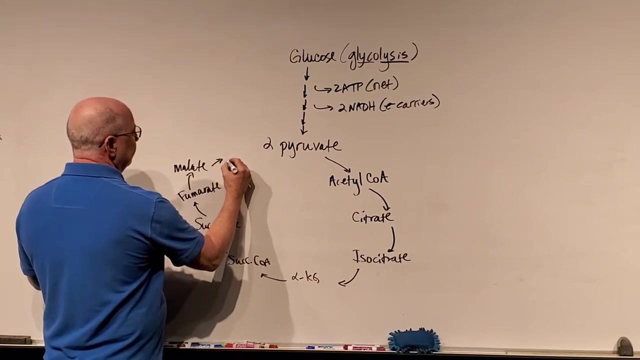 converted to a stuff called succinate or succinic acid. Succinate gets converted to fumarate. Fumarate gets converted to malate fumaric acid, malic acid. That gets converted to a stuff called oxaloacetate. I'm not going to write it out, but then oxaloacetate can be converted to oxaloacetate. 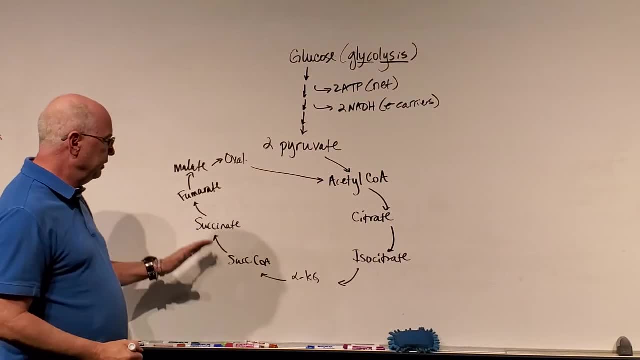 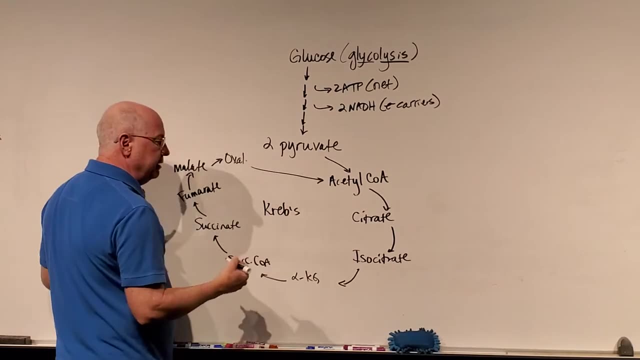 It can be converted back to acetyl-CoA and we can go back around. Now, this isn't the perfect circle, but you get the idea. This process was figured out by the guy named Hans Krebs, who became knighted Sir Hans Krebs, and we call that the Krebs cycle. Okay, it's called the Krebs cycle. 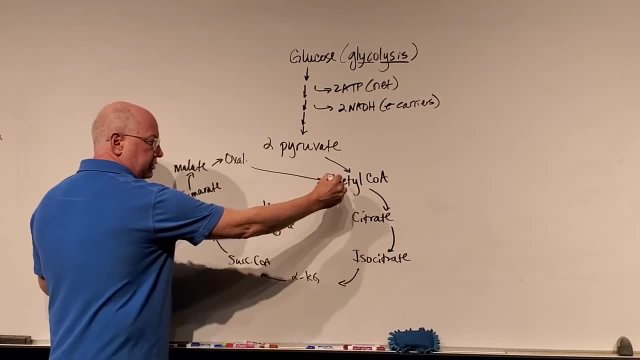 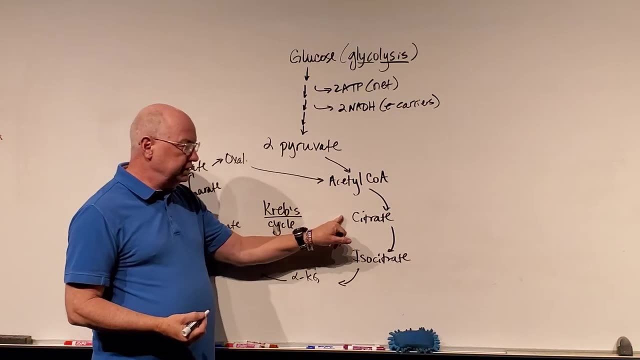 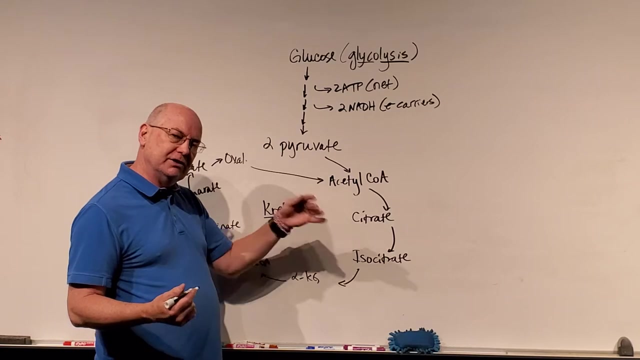 because it goes around and around and around. It starts with acetyl-CoA and it ends with acetyl-CoA and goes around again, Also called the citric acid cycle because it can be kicked off with citric acid. It's called the tricarboxylic acid or TCA cycle because citric acid has three carboxyl groups, so it goes by. 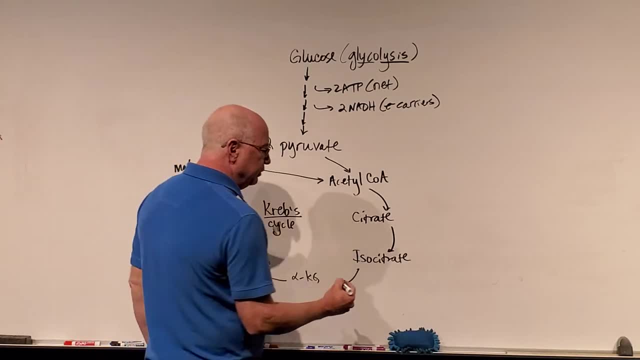 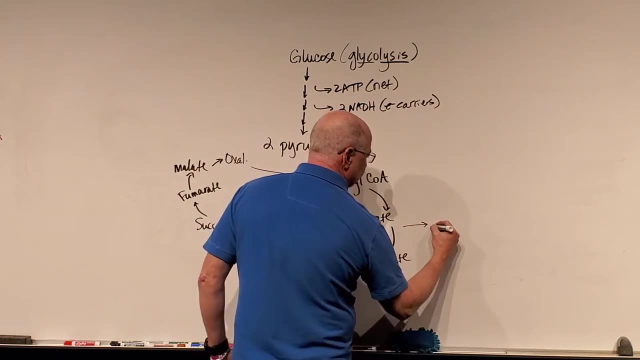 three different names. We don't care. Now, one of the things that we get from this process- although it's, I'm not going to use the exact step where these occur, but two byproducts come out of this. One is we get two more ATP gained, one for each pyruvate, and we get some carbon dioxide produced. 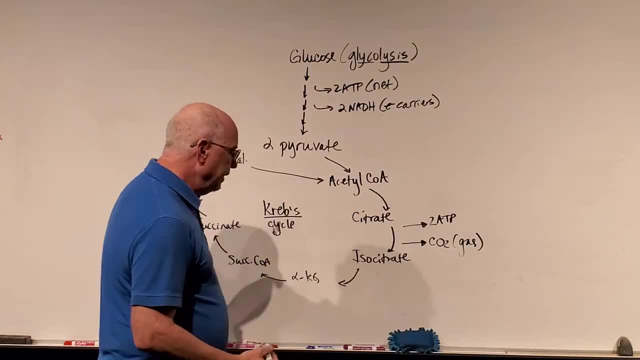 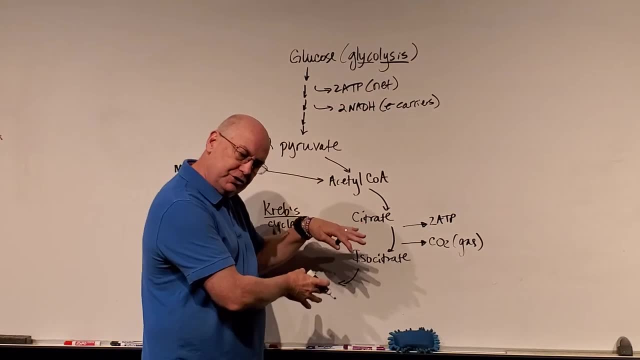 which is a gas, And then we also get some electrophoresis, which is a gas, And then we also get some electron carriers in the form of NADH and FADH2, and all the electron carriers go into electron transport. We're not going to be interested in that here, but then that would produce 32 more ATP, or sometimes even more, And so we can get a ton of ATP from one molecule of glucose. We only get two out of glycolysis, and some bacteria are happy with that. Some can produce two more and then produce even more through electron transport. As you know, electron transport is also called oxidative. 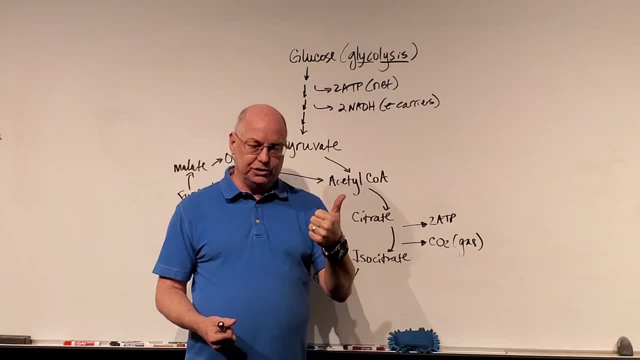 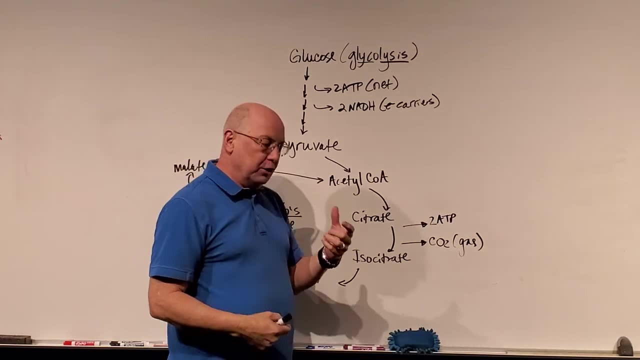 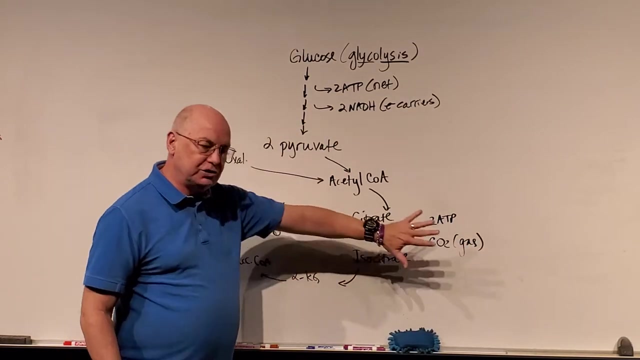 phosphorylation. It uses oxygen- that's the oxidative part- to add a phosphate group, phosphorylate ATP. So it requires oxygen for that to occur. If oxygen is not present, then all of these chemical pathways here back up and stop, And because we can produce carbon dioxide and it's 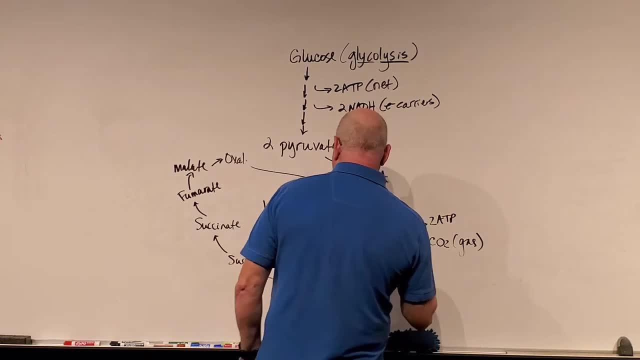 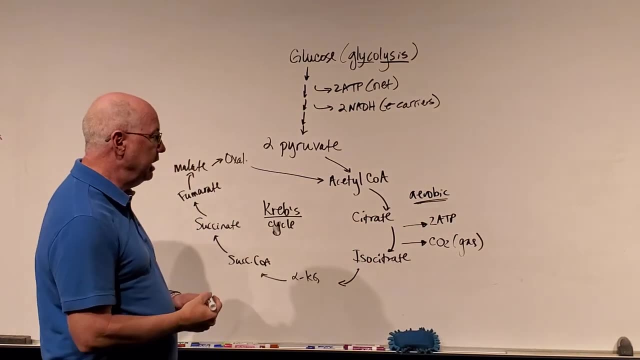 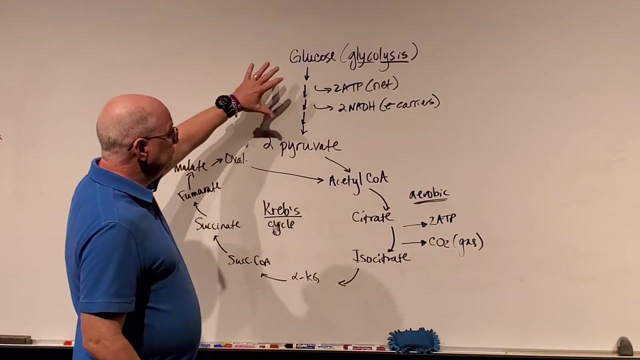 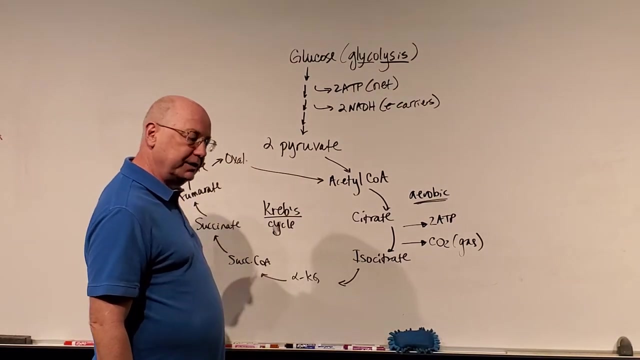 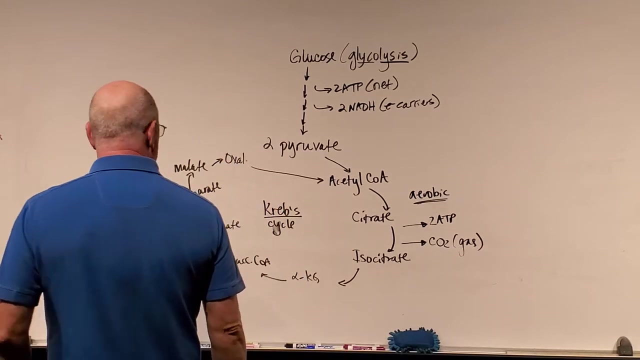 dependent, eventually, on the presence of oxygen. this part is called aerobic metabolism. We say that this process is called aerobic metabolism. We say that this process is called aerobic metabolism. This process is aerobic, requires air or oxygen and carbon dioxide is produced. Now, bacteria can do this, almost all bacteria. Some bacteria can do this and then some bacteria cannot. Now, before I go any further, I want to show you one last thing that I think is important for us, or two things I should say. 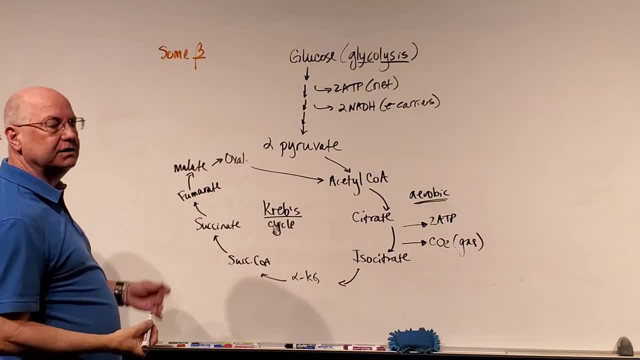 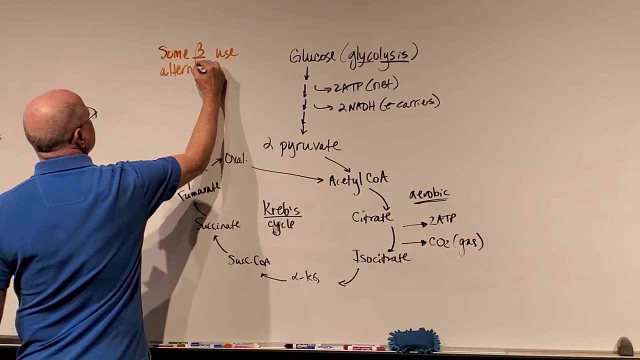 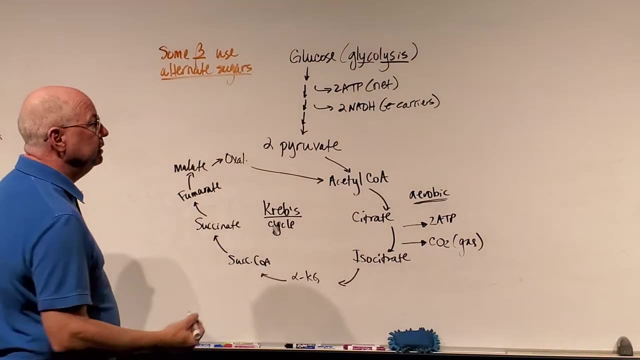 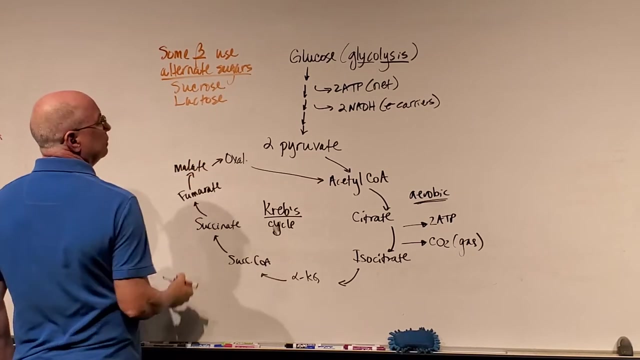 Some bacteria- this is my abbreviation for bacteria. it's the beta symbol, but that's how I don't want to write the word bacteria. Some bacteria can use alternate sugars. Not all bacteria can, but some. Some can use sucrose, some can use lactose, others can use maltose and other sugars. Now 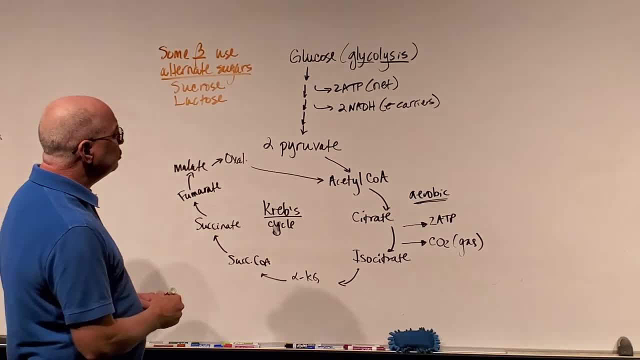 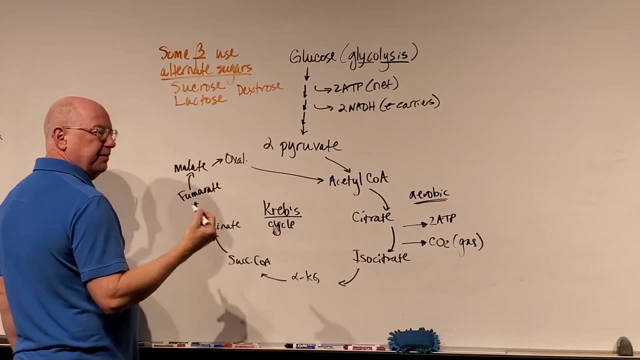 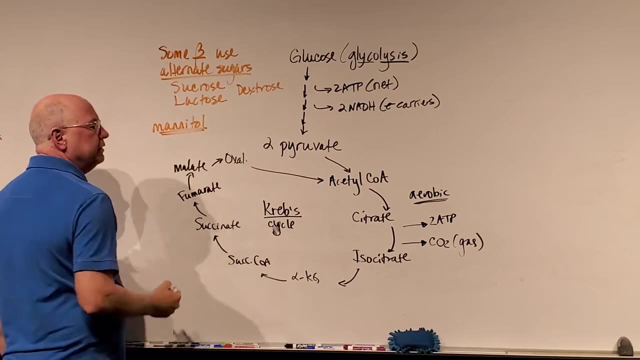 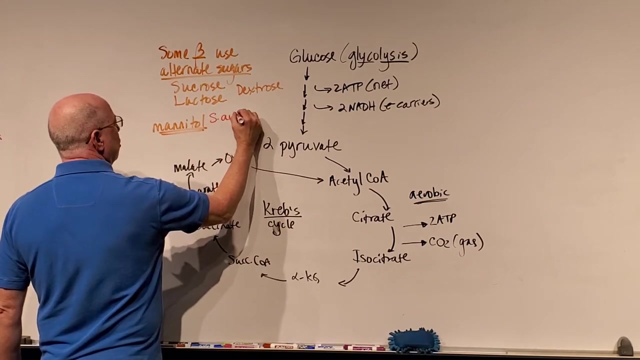 we're not going to go into all the sugars, but- and then there's an alternate form of glucose called dextrose. It's kind of a manufactured form. And then there's another sugar that some bacteria can use, called mannitol. Only a few bacteria can use mannitol. I'm going to write their names in red. One of these would be Staphylococcus aureus. 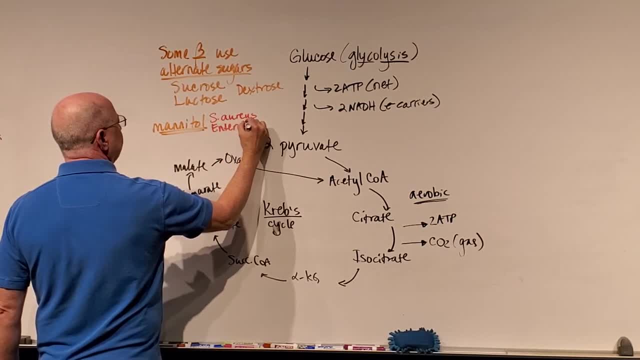 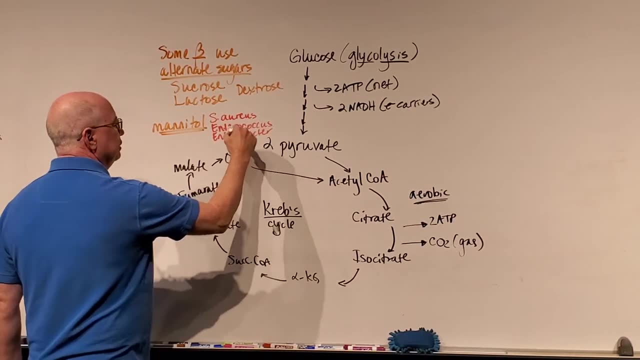 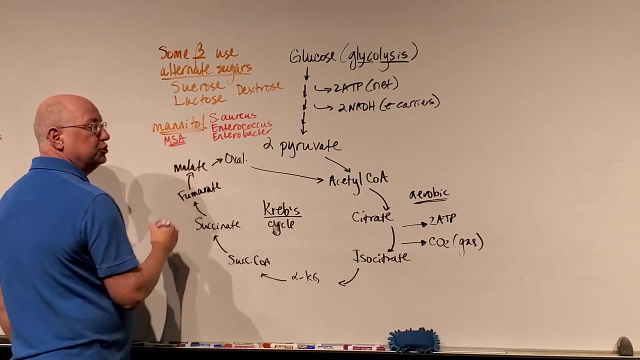 another one is a class of Enterococcus and then some Enterobacter bacteria, okay, The genus Enterococcus and Enterobacter. And so when we do what's called the MSA test, the mannitol salt auger, if it can break down the mannitol then it's going to be one of these usually. And 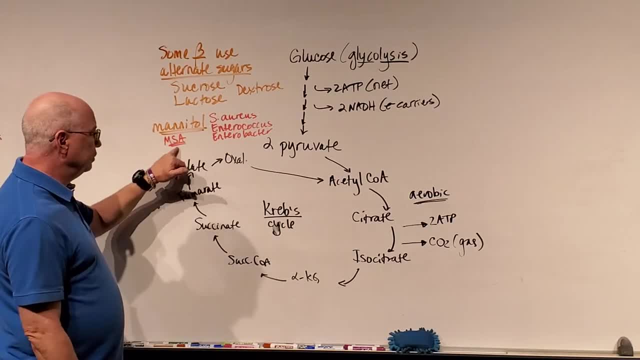 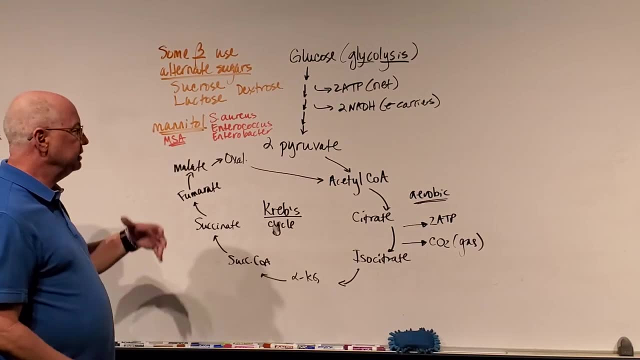 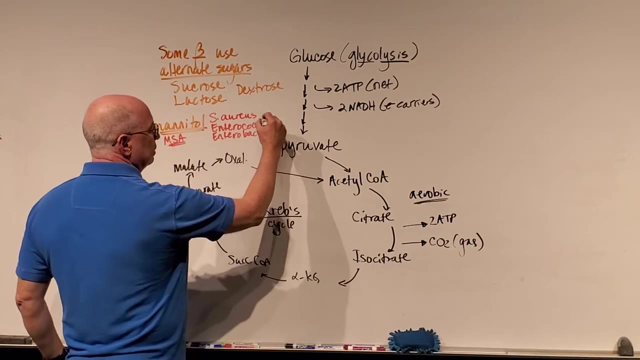 then most other bacteria won't survive in that. And then, of course, the high salt can help us differentiate between which ones or select for which ones. So we did an MSA auger test and that mannitol salt auger is simply because some bacteria can utilize mannitol to turn into pyruvate. 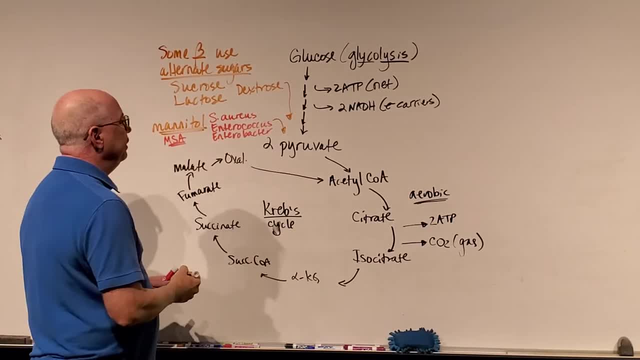 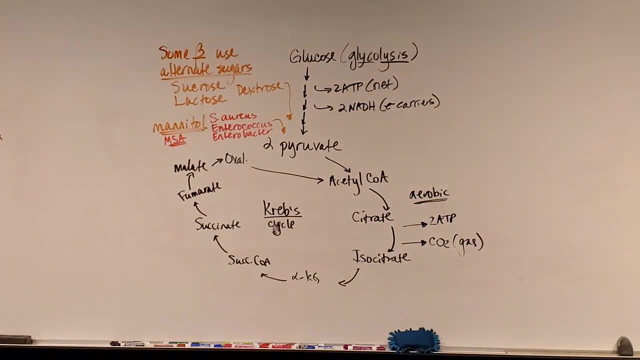 Some bacteria can use these other sugars and turn them into pyruvate. And then, finally, the last little detail. let me make sure I'm not going to run out of space on the side of the board Now. I've got plenty of room over here, Okay, good, The last little detail that I want to show you is this: 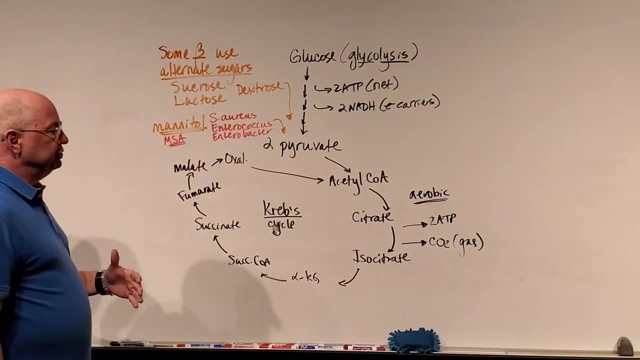 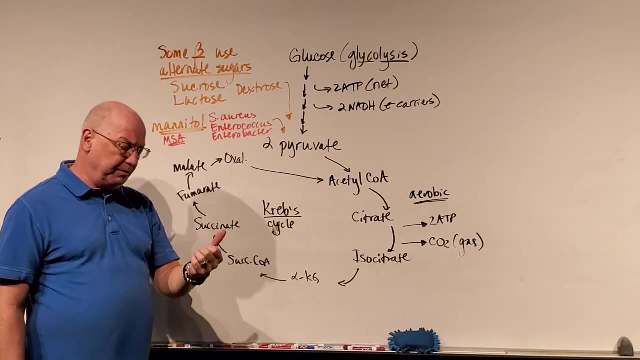 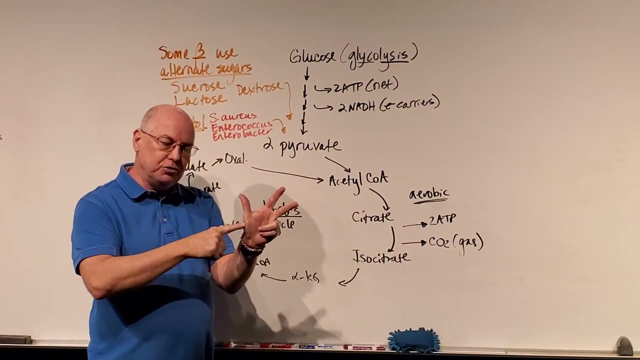 Some organisms- humans are them, are one, I should say. When we run out of sugar, we can burn proteins, convert them to amino acids. Remember, amino acids have carbon hydrogen and oxygen, just like glucose, But they have a nitrogen group called the amino group. 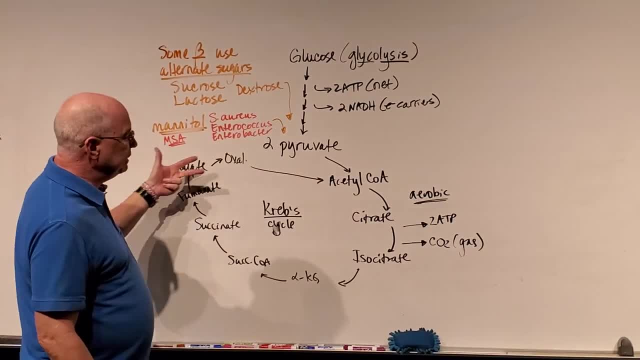 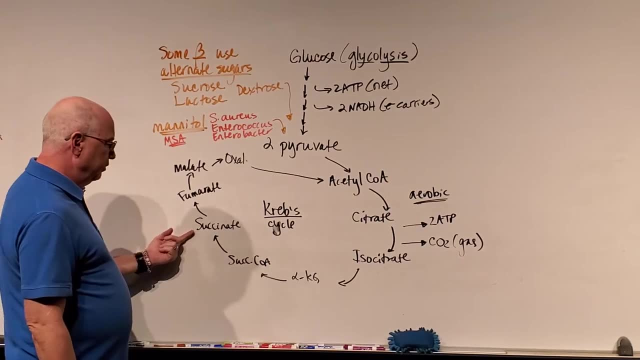 If I remove the amino group, I can convert some amino acids into energy. One amino acid I can convert into pyruvate, it's called tryptophan. Another one I can run into these chemical reactions somewhere along the way where it's not important- called cysteine. 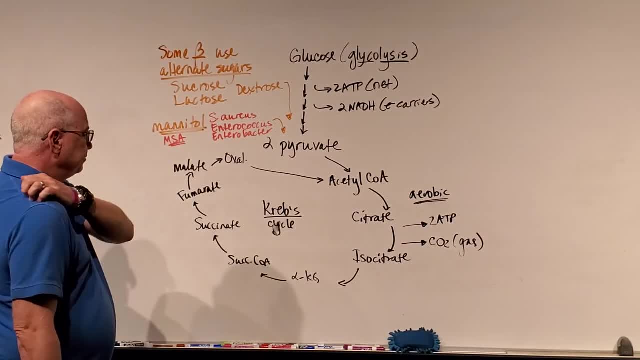 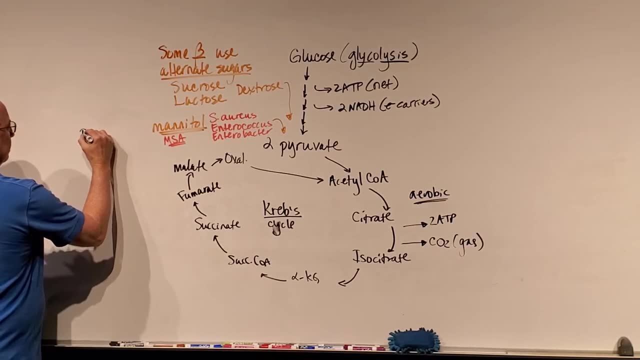 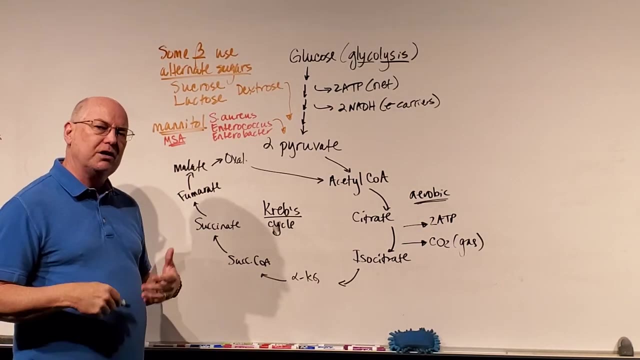 And other amino acids can also be converted into energy. So when we talk about certain media, we use a stuff called peptone. We talked about this. Peptone is in what we call an undefined media or complex media, okay, where we don't know all the products. 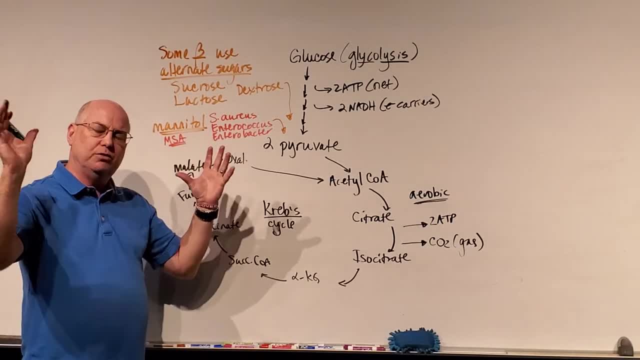 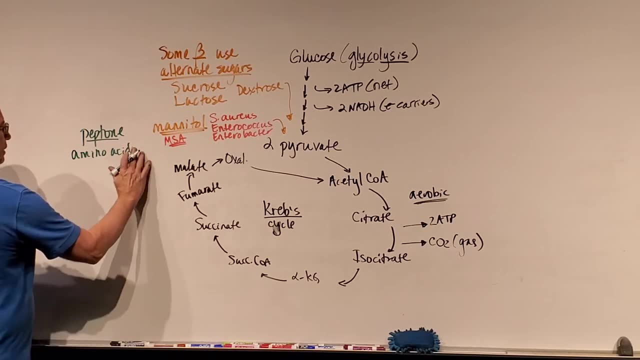 Peptone is simply, We take some proteins and we digest them to release a lot of the amino acids. So anytime there's peptone present, I think amino acids. okay, Now one particular amino acid. I'm going to try to change the colors so we can follow these along the way, all right. 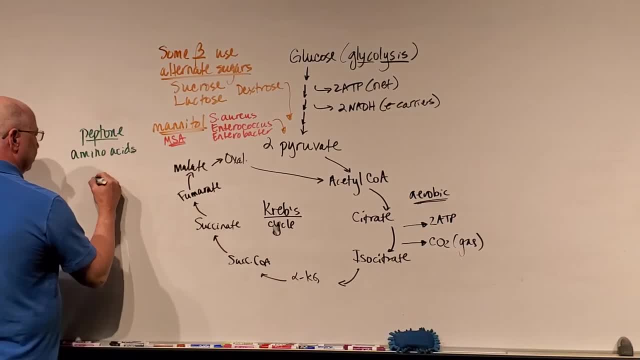 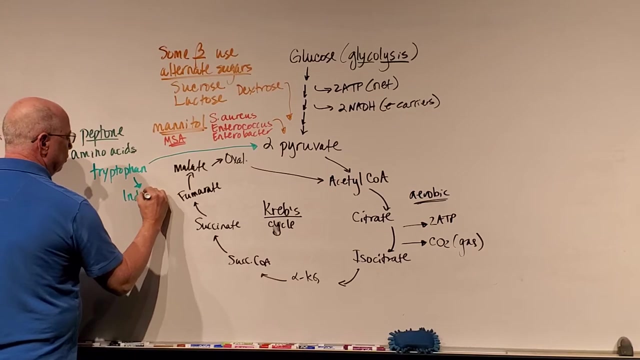 One particular amino acid that we can use is called tryptophan. okay, Tryptophan can be converted- These arrows are all going to get kind of messy- into pyruvates and then used for energy, But in the process it gives us a side product, a byproduct called indole. 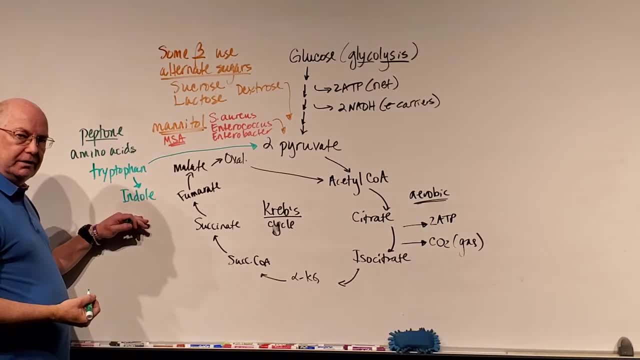 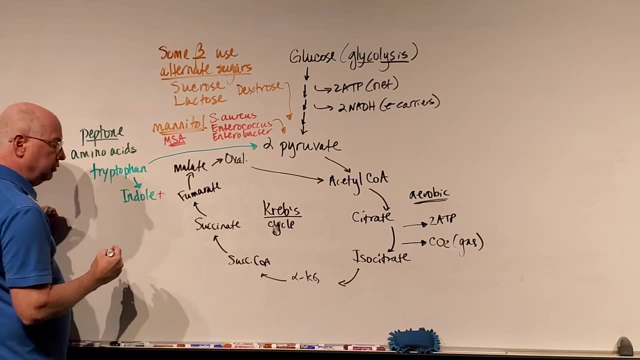 So we can do an indole test in lab. And one of the bacteria that can convert tryptophan into pyruvate and make a test that's indole positive is Proteus mirabilis. Okay, So we know that, Proteus mirabilis, can? I'm sorry, no, it's not Proteus mirabilis. It's E coli- I'm sorry I was thinking another step down, Forgive me- And some enterobacter species. okay, So if we get a positive indole test, then we know that we have E coli or some enterobacter species. 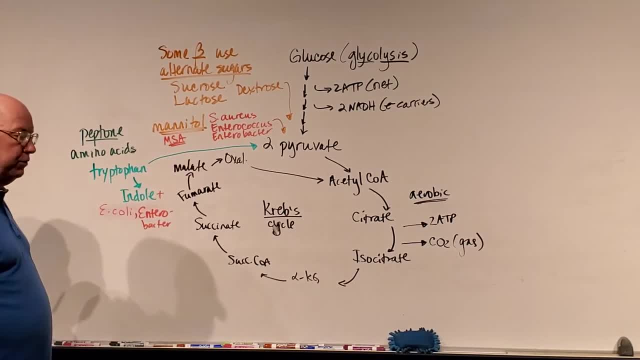 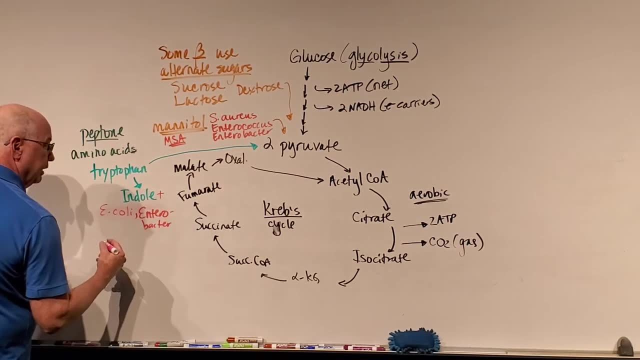 Present because they can convert tryptophan into pyruvate. Another amino acid that we can use- and I'm going to try to use a different color for this one- is- let me use blue. Maybe it'll stand out really well. 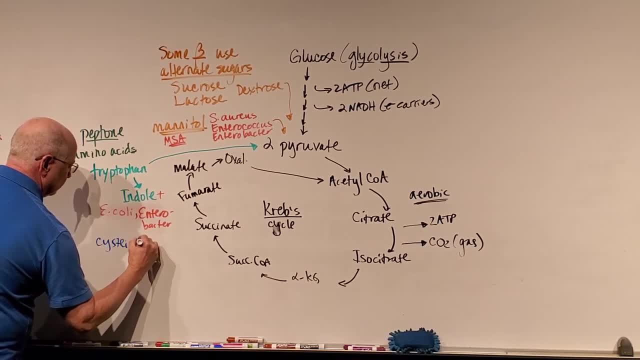 It's called cysteine. Now, cysteine can be converted into compounds that are used in the Kremp cycle, And one of the things that happens in cysteine is that we produce a lot of sulfur. Okay, And cysteine is an amino acid that has a sulfur group on it, an SH group. And so when we break down cysteine for energy, sulfur gets produced. Now one of the things that happens with the sulfur is when we test for it sulfur-positive bacteria. if we get a sulfur-positive test, that's when we know we have what's called Proteus mirabilis. 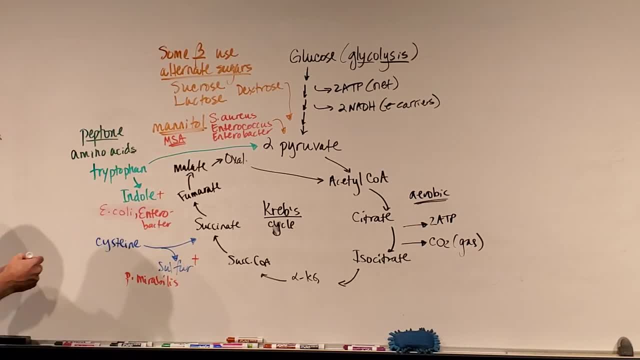 Okay, It produces a positive test for sulfur. Now, one of the last things I want to talk about when we talk about these is sometimes when we break down these amino acids. as we break down the amino acids from peptone, one of the side groups, as I said, is that the amino acids that are present in the peptone are the amino acids that are present in the peptone. 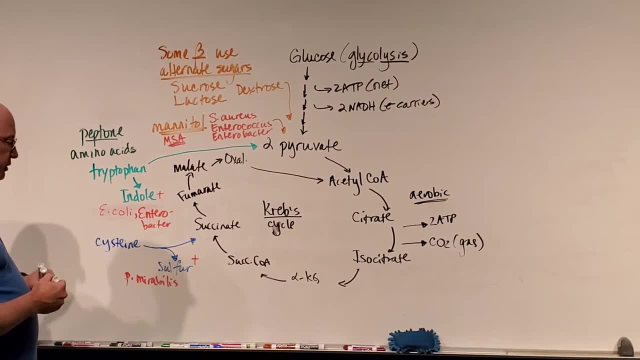 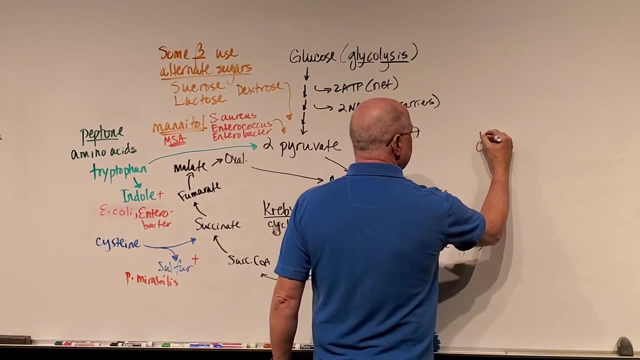 Okay, And one of the side groups, as I said, is that little NH2 group called an amino group, hence the name amino acid, And I don't know if you recall this, so I'll draw it right over here. I'm going to erase it in a second. 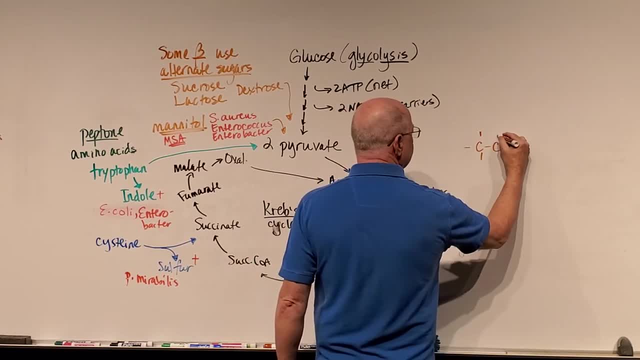 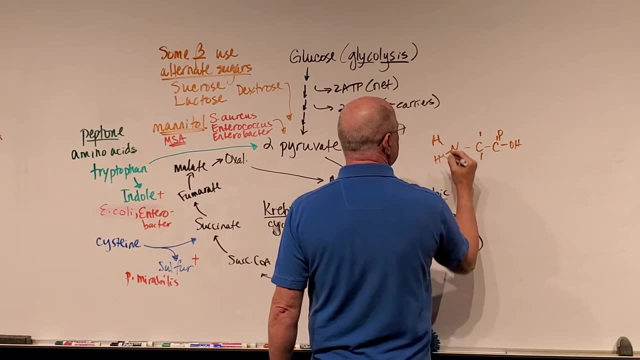 But amino acids all have a centrally located carbon. On one side they have a carboxyl group, On the other side they have a nitrogen group that has two hydrogens associated with it. This is our amino. That's our acid. 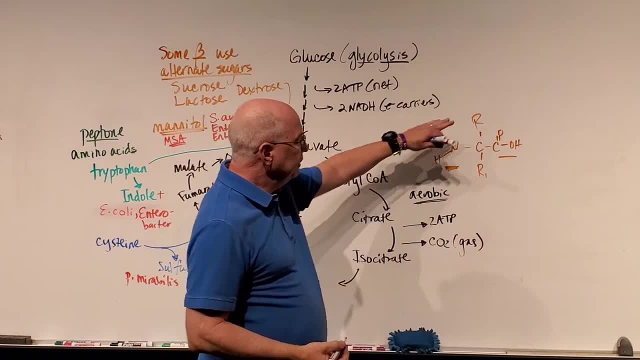 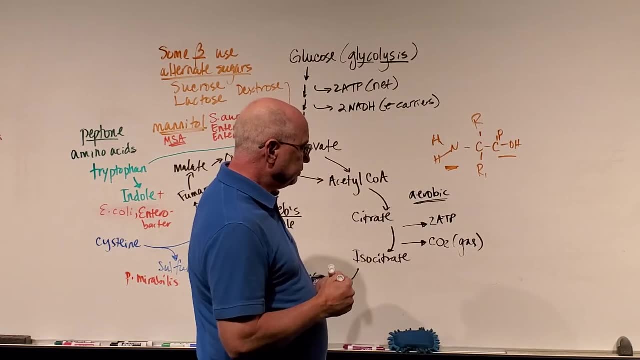 Then we have an R group, an R1 or an R prime group. These can be other things. It can be sulfur, It can be other carbons and other compounds. Okay Now, in order for me to metabolize amino acids for energy, I have to take off the amino group. 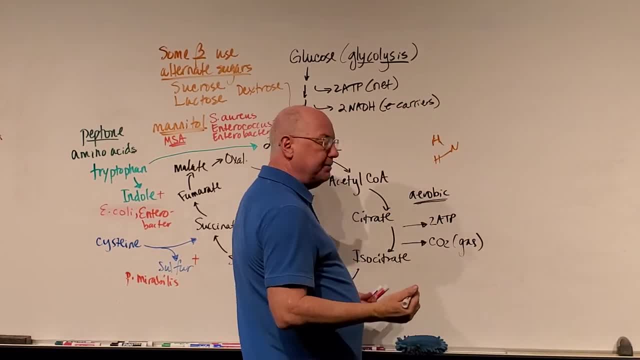 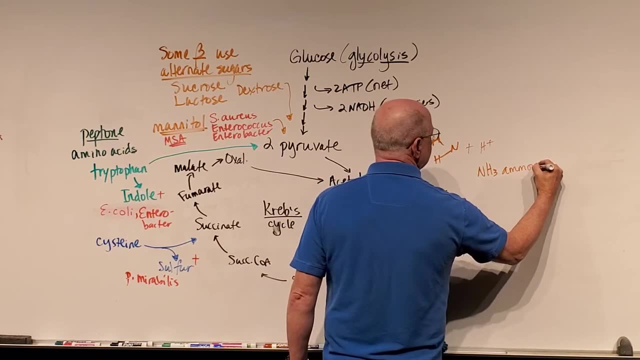 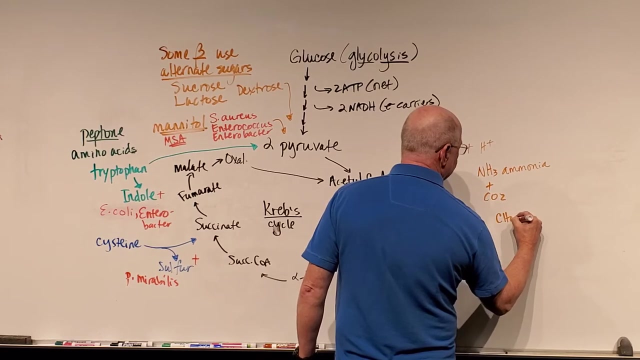 When I remove the amino group. we call that process deamination. If I combine this with a free hydrogen, then I get NH3, which is ammonia. Ammonia can be combined with some carbon dioxide And we can get a stuff called CH4ON2, which is urea. 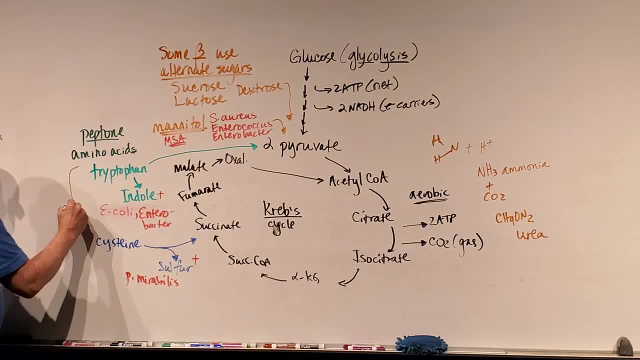 So sometimes when I break down amino acids, I'm going to get ammonia and then I can get urea. Urea can be used by a couple of bacteria for energy, And so there's a test that we can use The test for urea and the breakdown of urea for energy using an enzyme called urease. 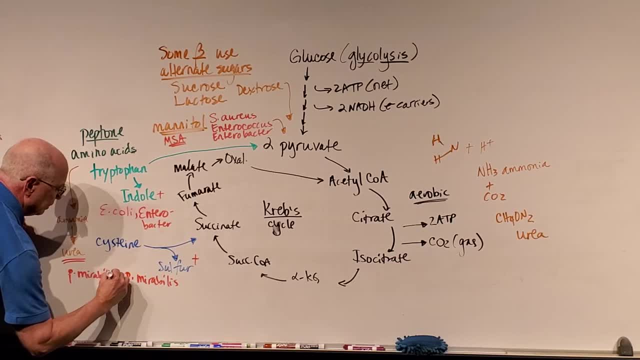 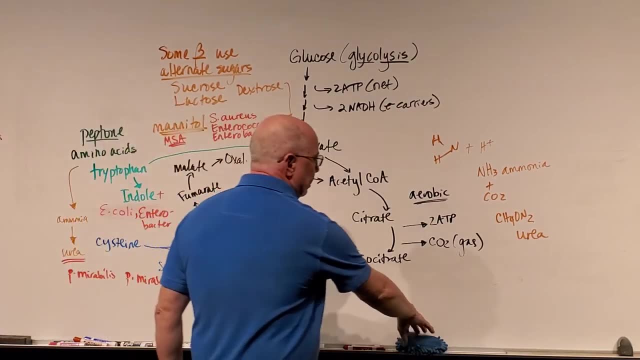 And again, Proteus mirabilis is a bacterium that can do that. So I want to write something. I'm going to erase this now because we don't need this part, But I want to point out a few things so far. 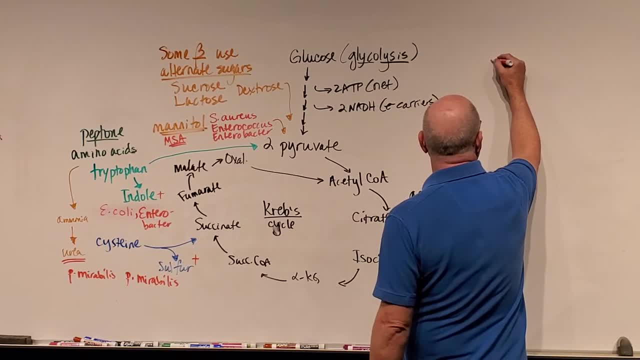 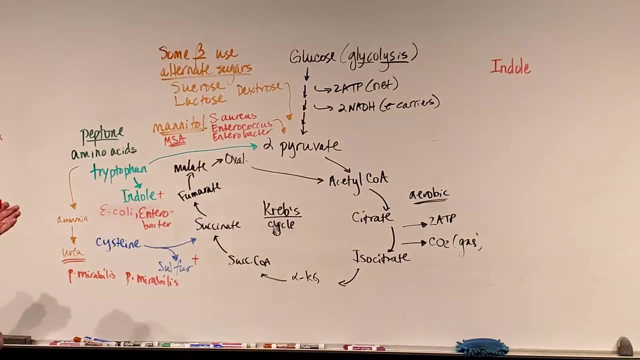 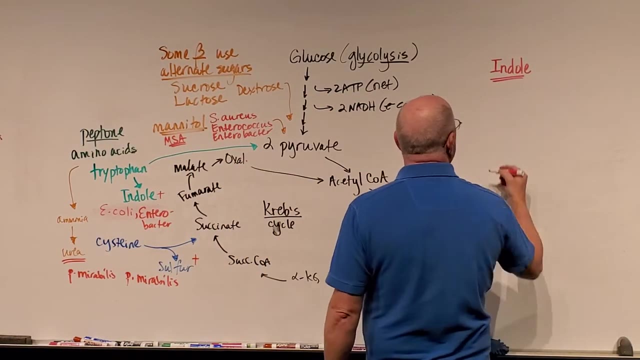 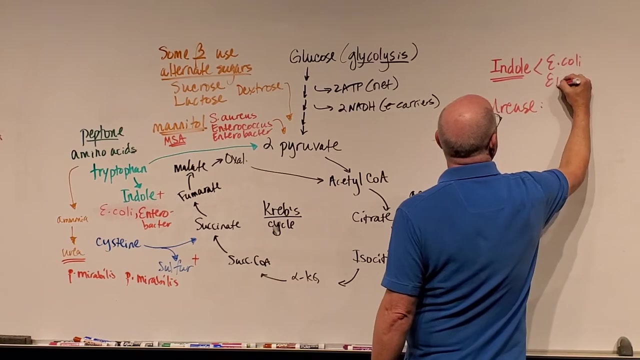 First of all, if you do an indole test, the indole test will tell you if we have E coli or Enterobacter. If we do the urease test or the urea test, so this gives us E coli or Enterobacter. 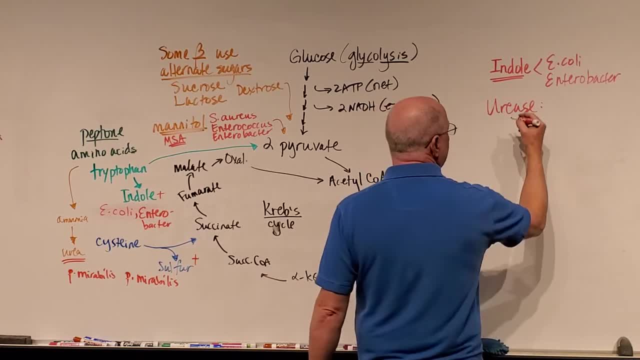 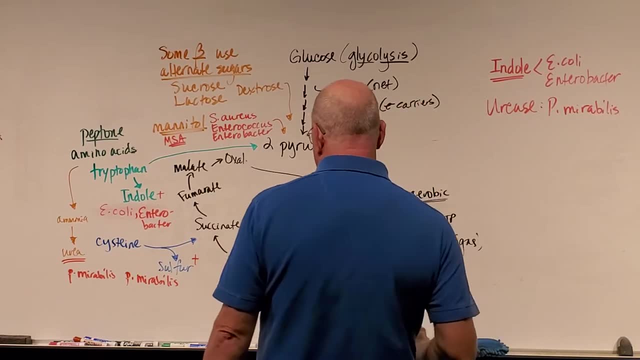 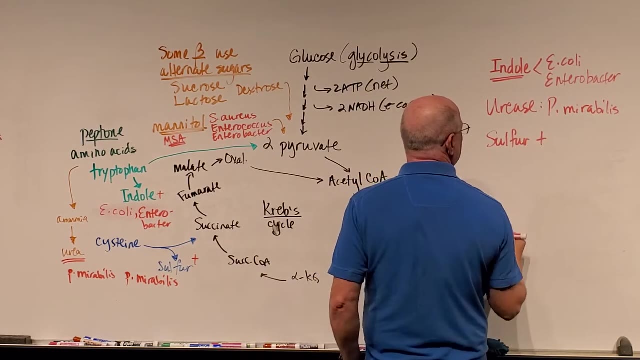 as long as the test is positive. If we do the urease test, then we can tell if we have Proteus mirabilis. Now, if I do a sulfur test and it's sulfur positive, then I know I have Proteus mirabilis. 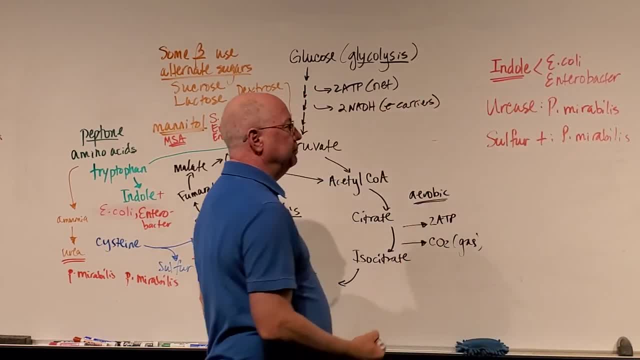 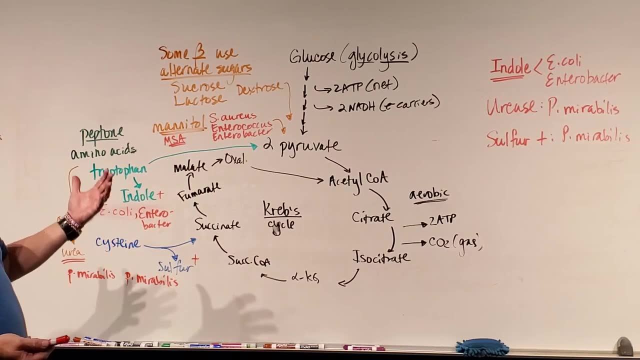 So if I get these two tests to be positive for me, then I can pretty much identify my culprit as Proteus mirabilis. If I get a positive test for indole, then I know I either have E coli or some other Enterobacter causing the issue. 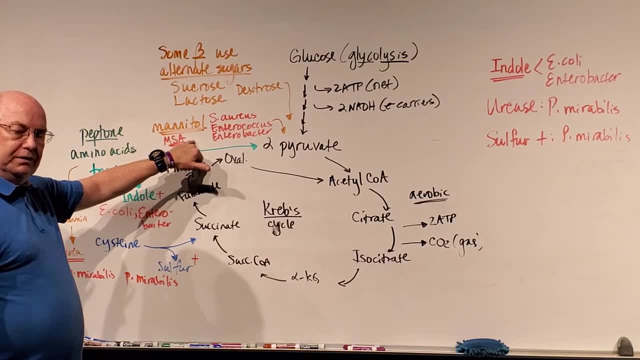 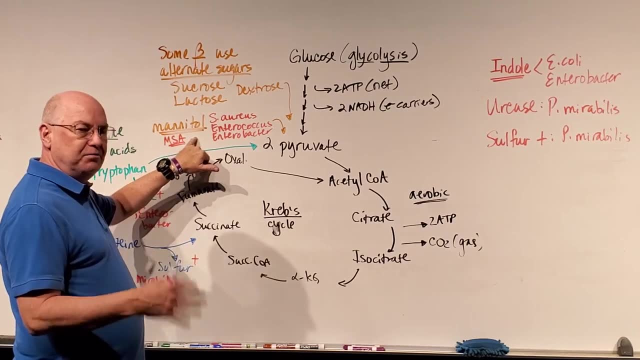 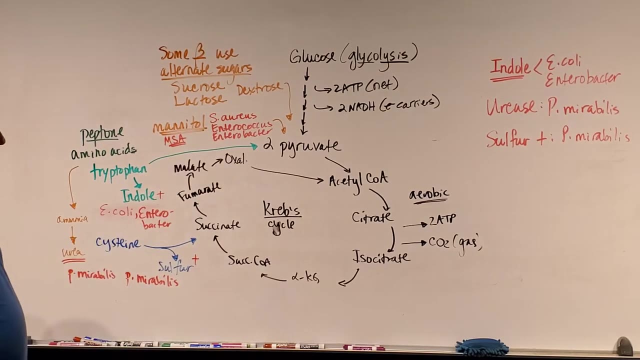 If MSA gives me the results, if the bacterium or pathogen can break down mannitol, then I know it's either Staphylococcus aureus causing an infection, Enterococcus or an Enterobacter species. So several of the tests that we run will tell us this information. 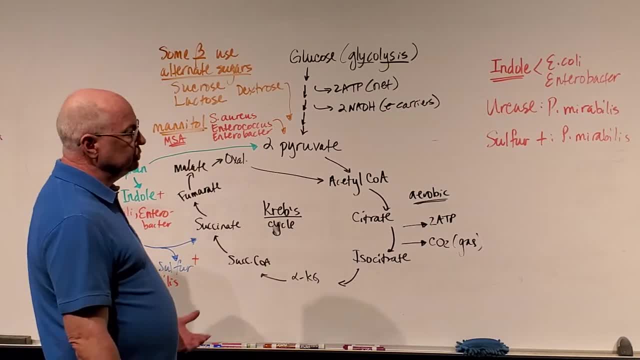 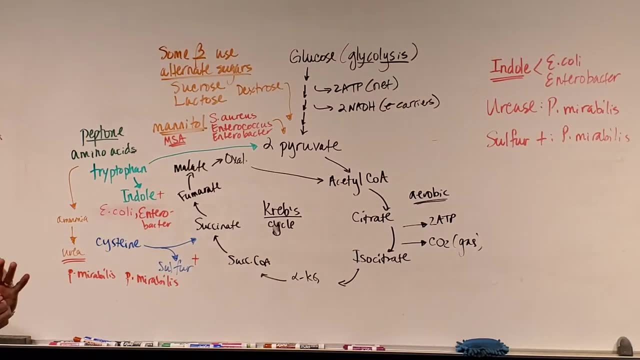 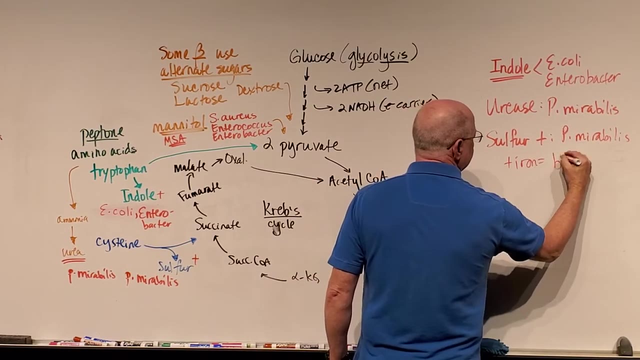 One of the tests we run is called the triple sugar iron test and any time that iron reacts we know that we have Proteus mirabilis, because sulfur plus iron gives us a black precipitate And we're going to see that in some of our tubes. 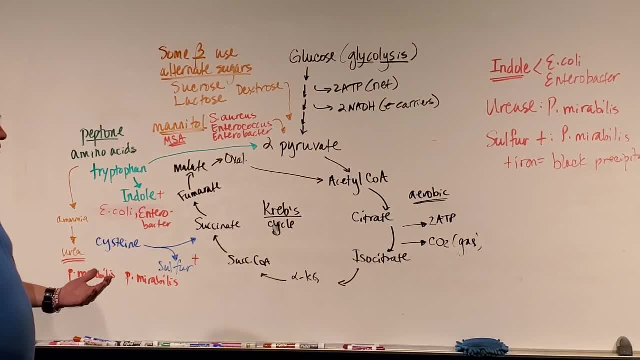 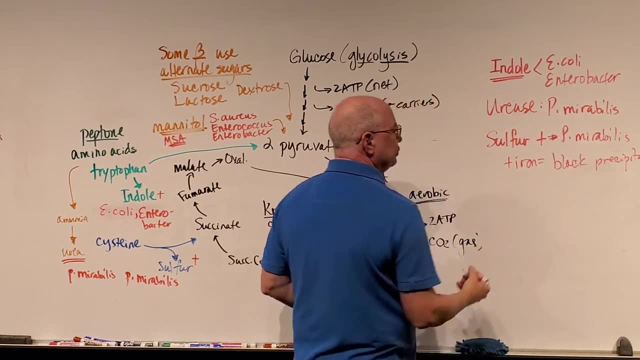 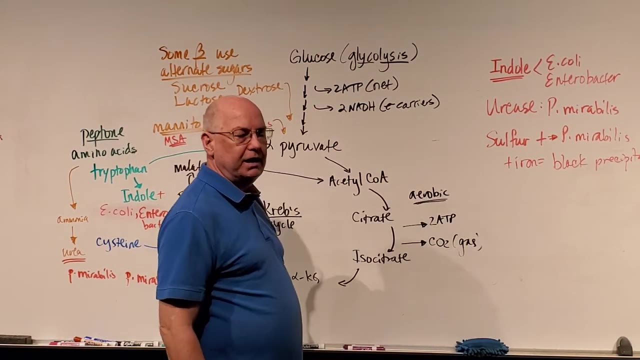 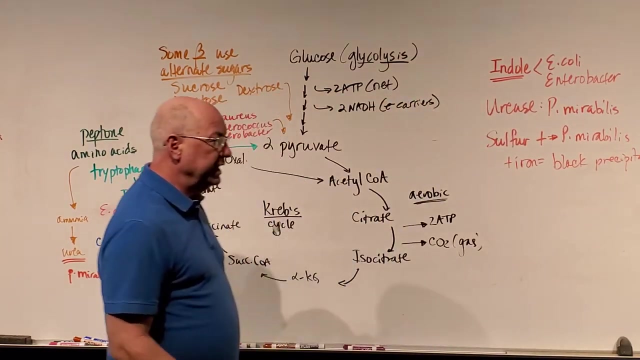 If Proteus mirabilis is present, then the positive sulfur test. when iron reacts with sulfur and it makes this black precipitate, then I know I probably have Proteus mirabilis present. Also the urea test. One of the tests we do in lab simply is a tube. 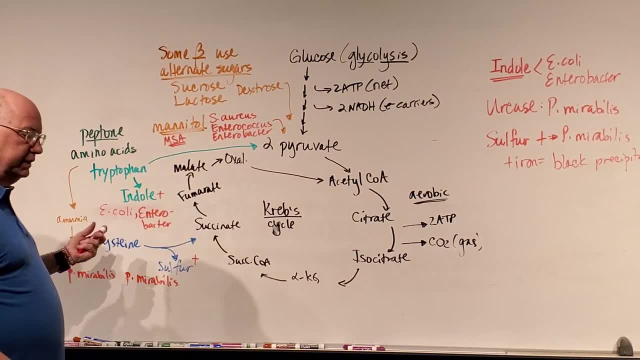 that has the ability to test for the metabolism of urea, and if the urea is present, if the urea test gives us a positive result, then we know Proteus mirabilis is present. If we were to start listing the tests that we do, 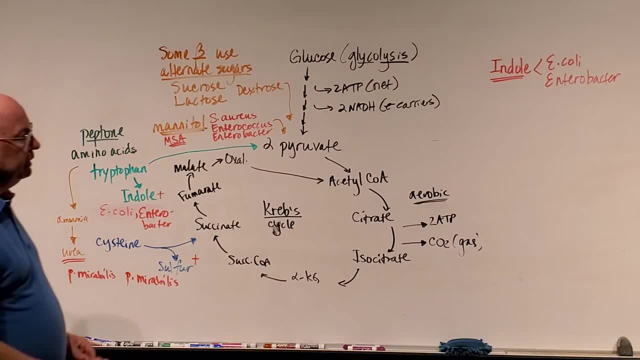 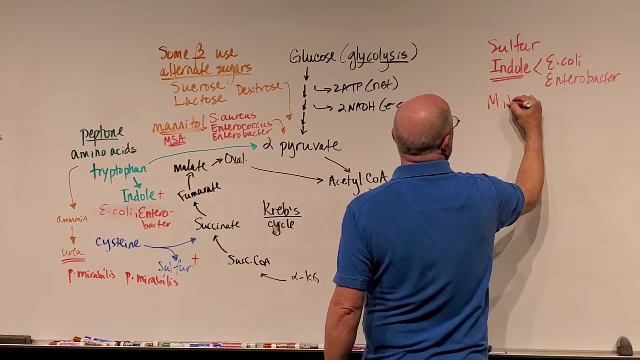 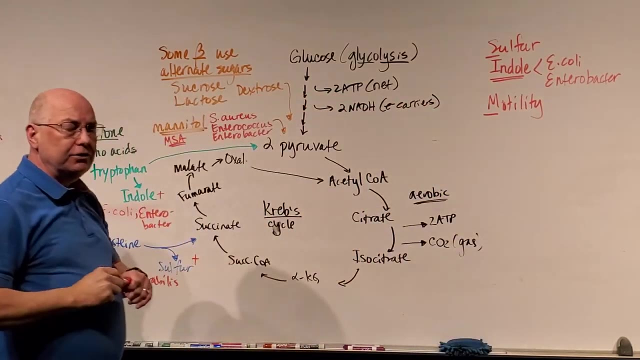 one of them is the indole test. The indole test is part of what we call the sulfur-indole motility test or the SIM test. If we get an indole-positive reaction, it's E? coli or enterobacter. 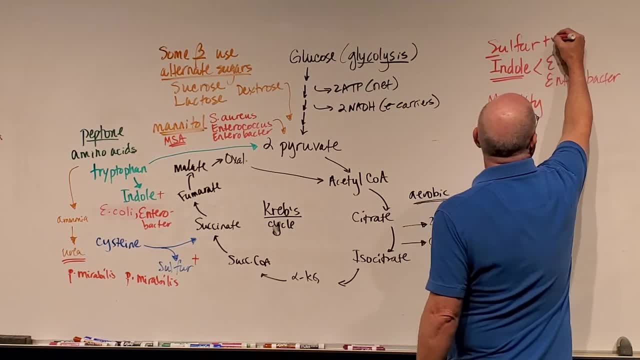 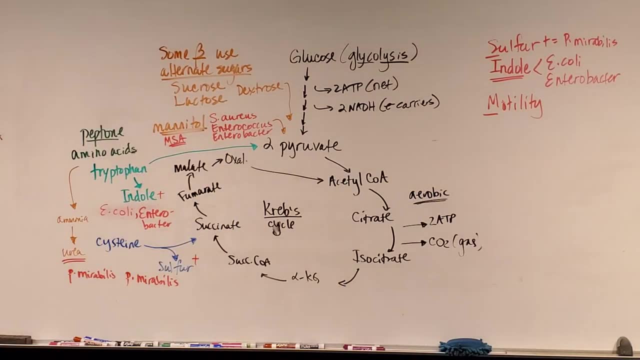 If we get a positive sulfur reaction, then we know it's probably Proteus mirabilis. So when we look at the SIMS test, the sulfur-indole-motility test- excuse me while I take a drink- essentially it's testing if can our bacteria reduce sulfur. 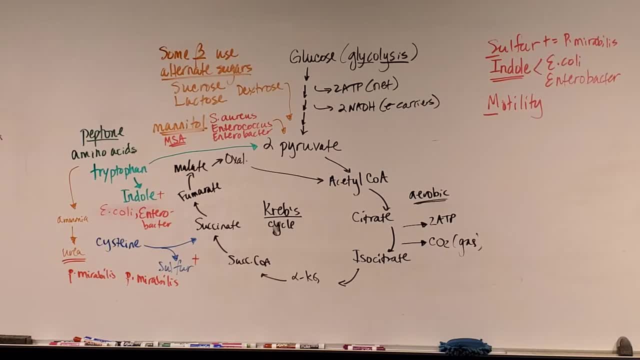 does it produce indole, and are they multiple? Can they move around? Okay, I think that's all I want to tell you on that one. Now again, the urea test will tell us that Proteus mirabilis is around. 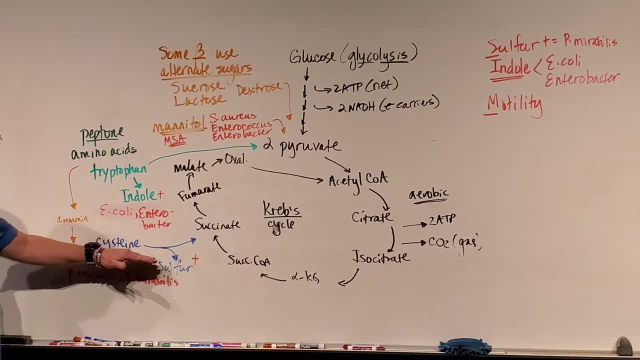 because Proteus mirabilis can break down cysteine, producing the sulfur. so both the sulfur test and the urea test can back each other up and confirm that we're getting Proteus mirabilis. So one test we did was SIM. 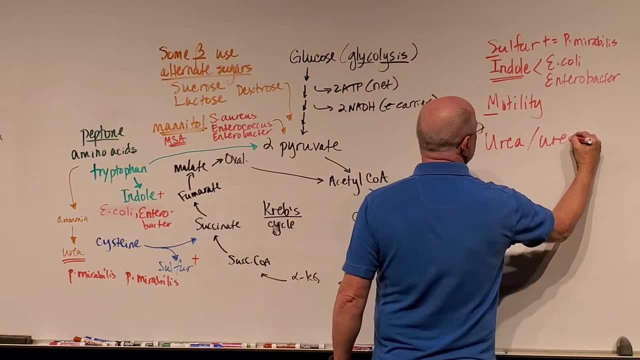 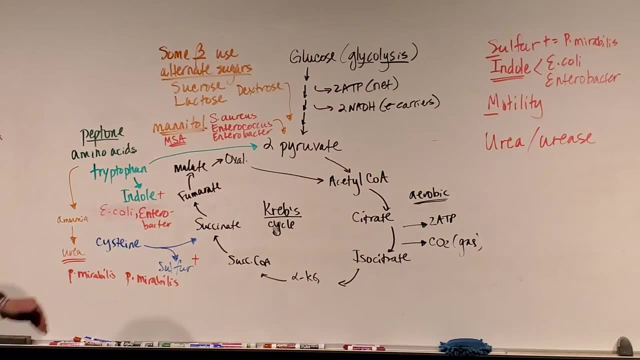 one was called the urea, or some people call it the ureaase test, and then, of course, mannitol salt. auger- which we're not doing at this point in lab, we did it before with plating- will tell us if these bacteria are present. 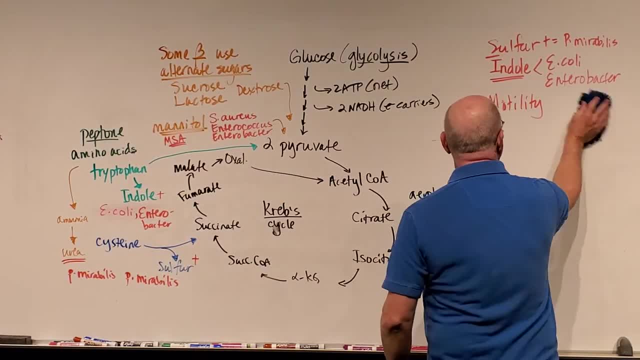 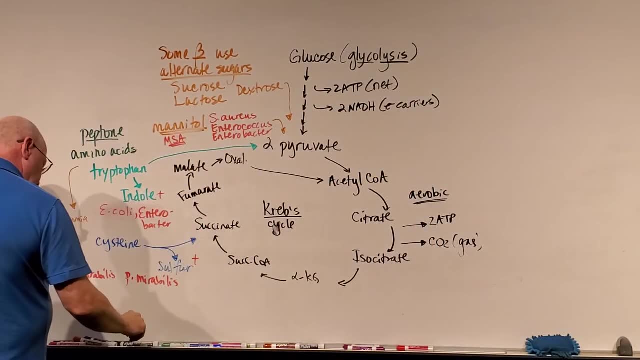 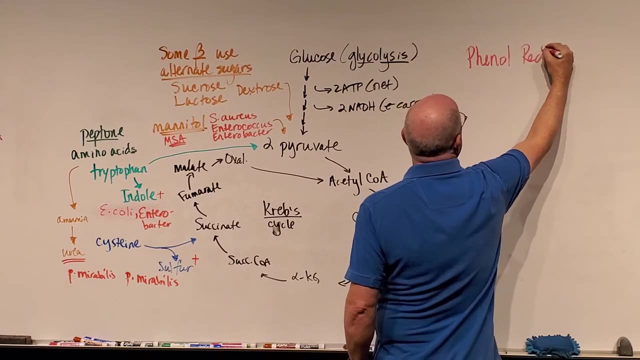 Now I'm going to erase this, because there are still some other tests that we've used in lab that can help us identify certain bacteria. So one of the tests that we talked about is called the phenol red tests, which are usually abbreviated PR. 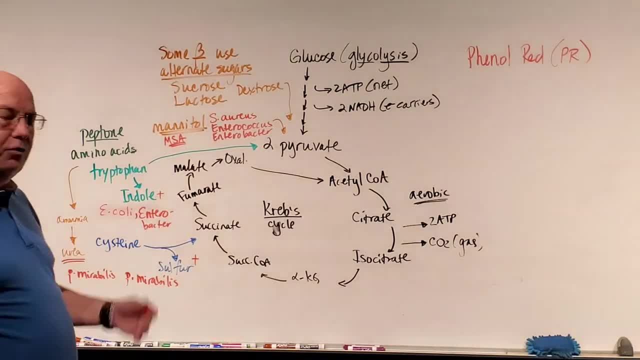 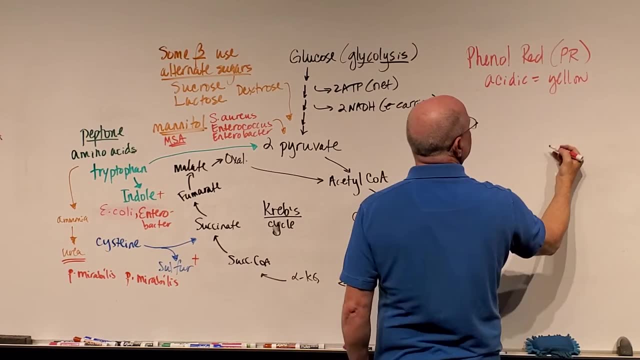 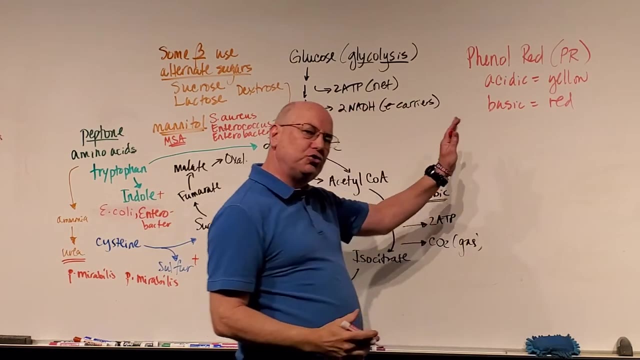 Now one of the things I want you to know is that when we add phenol red to a tube, if it's acidic it's going to convert to yellow. If it's basic, then it's going to be red. So if it's kind of neutral to basic, 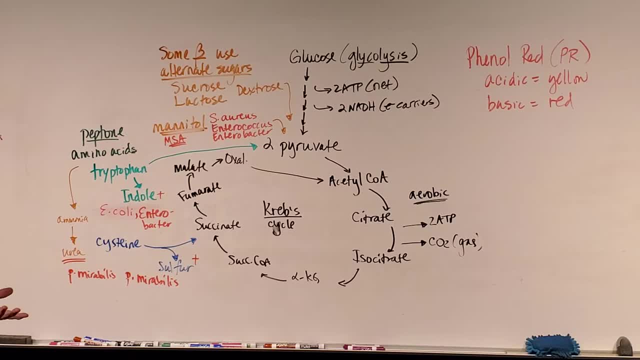 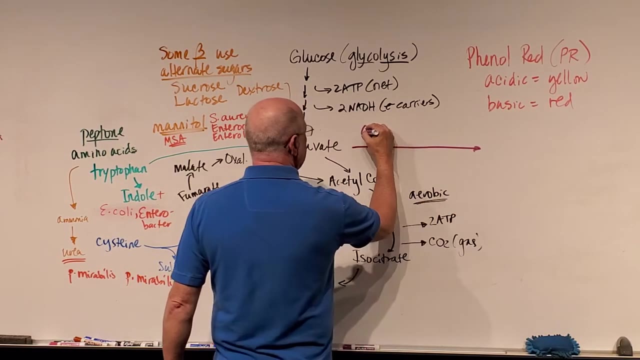 then we get a red coloration. If it's acidic, then the media will appear yellow. Well, why is that important? Well, it's important because of this: Some bacteria have the ability. if it's anaerobic, under anaerobic conditions. we get the fermentation of pyruvate And there's a whole bunch of bacteria that can do this, And we can get four products. I'm going to list them here, So the four products that come from fermentation. the first one is lactic acid. 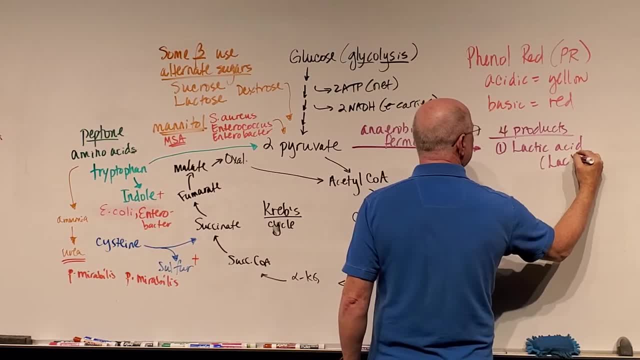 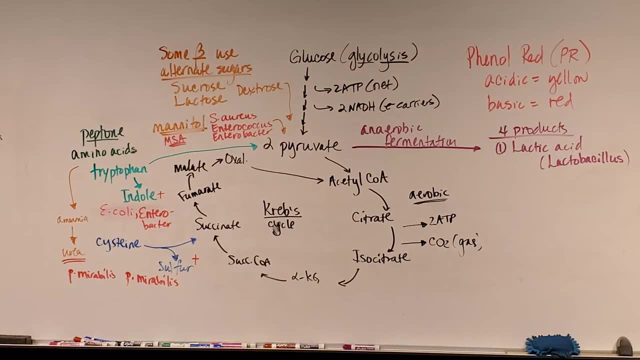 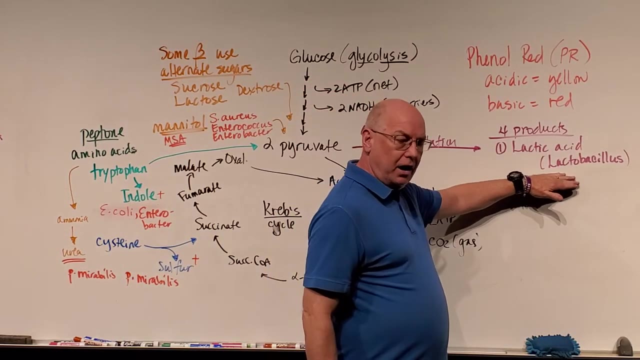 One bacterium that can do this is called lactobacillus. Now, lactobacillus. let me make sure everything's fitting on the board and I'm not writing on the screen. yes, I'm just on the edge. Lactobacillus is a probiotic. 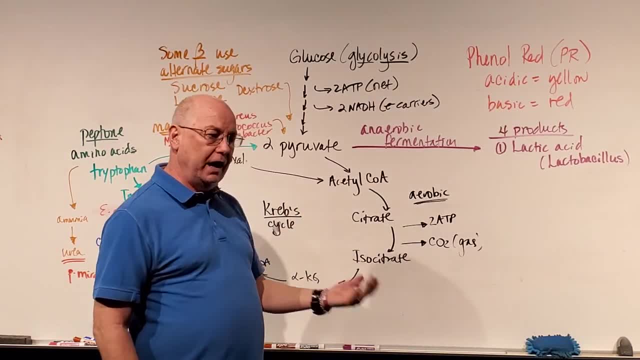 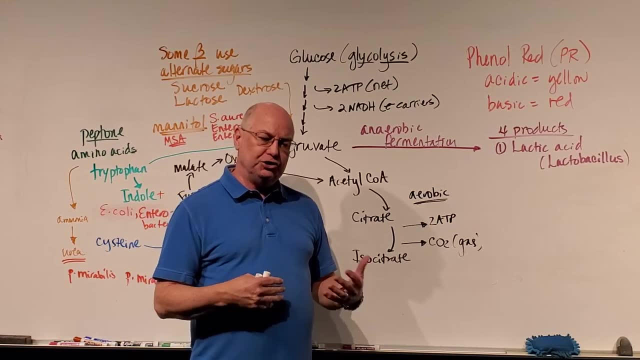 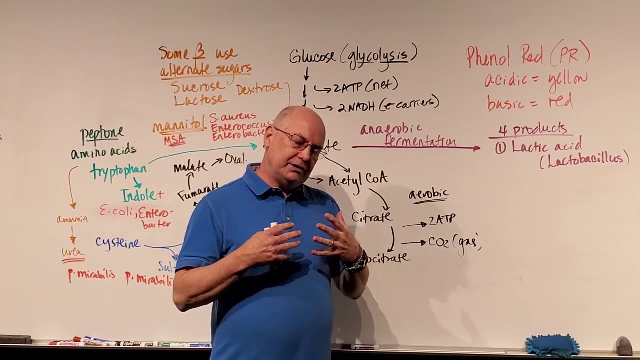 It's one of the bacteria that inhabits part of our gut and the vaginal canal, And it does what we call microbial competition or microbial inhibition, where the presence of lactobacillus, a beneficial bacterium, creates a somewhat acidic environment to prevent other bacteria. 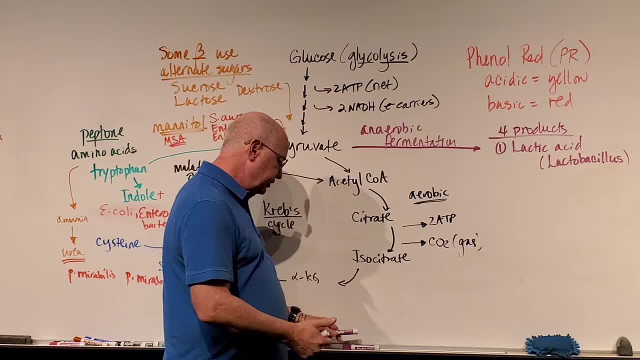 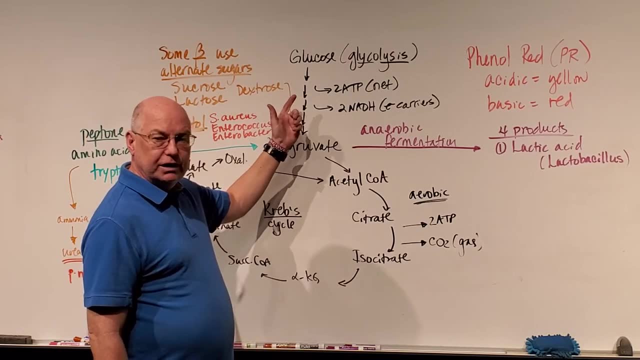 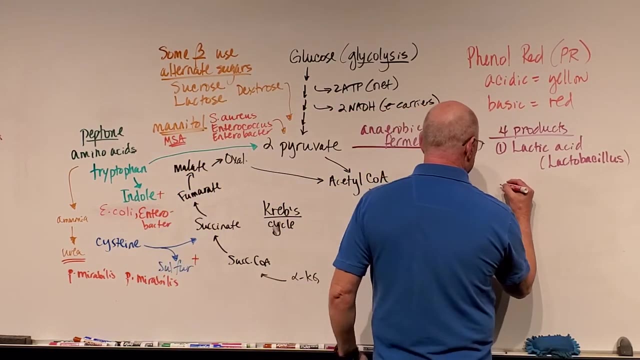 from seeding in that area and from causing an infection, And so lactic acid fermentation from things like glucose and some sugars is an indication that lactobacillus is there Now. a second byproduct that we can get from this is alcohol. 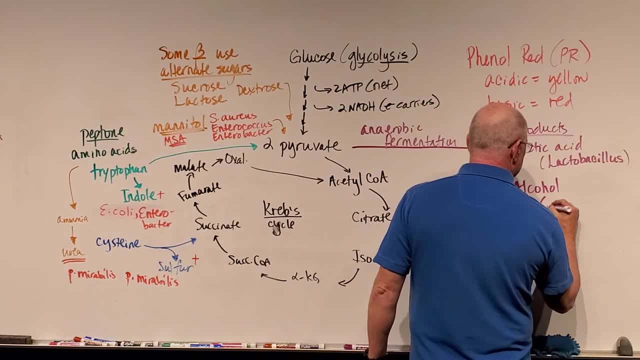 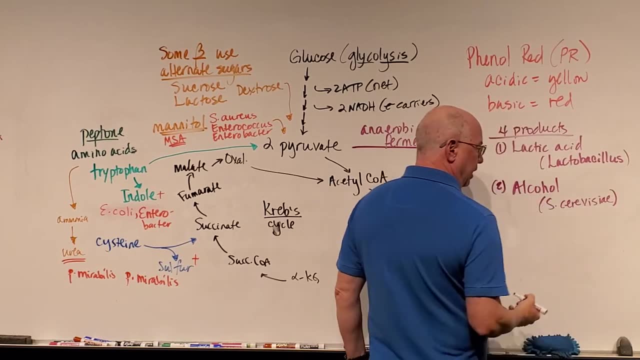 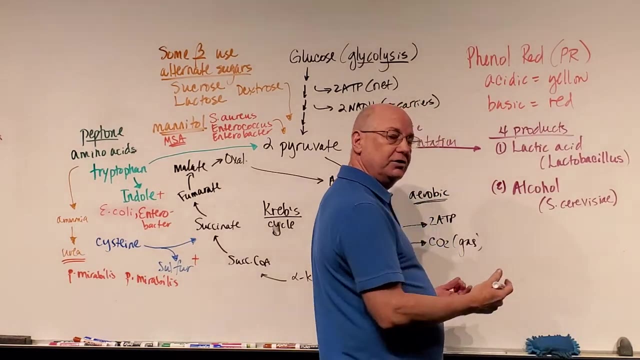 Ethyl alcohol. One bacterium that does this is Saccharomyces cerevisiae, And that does beer and wine. We're not interested in that for health science reasons, but we are interested in it, for after a long shift you might need a drink if you partake. 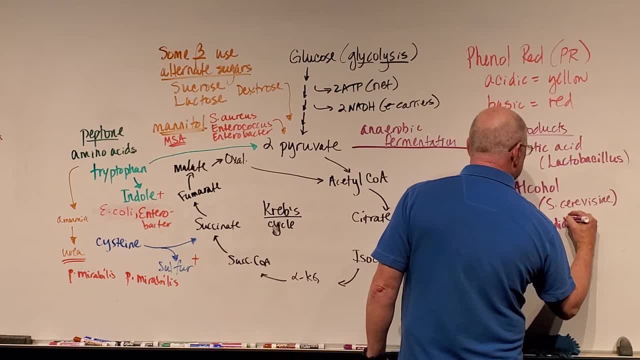 But another one. another microbe that can do this is called Candida albicanis, So let me just erase Saccharomyces cerevisiae. There is a yeast called Candida albicanis that causes yeast infections- That's my abbreviation for infections. INFXNS. Now in some cases it's reported that yeast infections can be so severe that if someone has one but they don't get it addressed, then if the yeast infection gets worse and worse and worse, you can actually detect an aroma of alcohol. 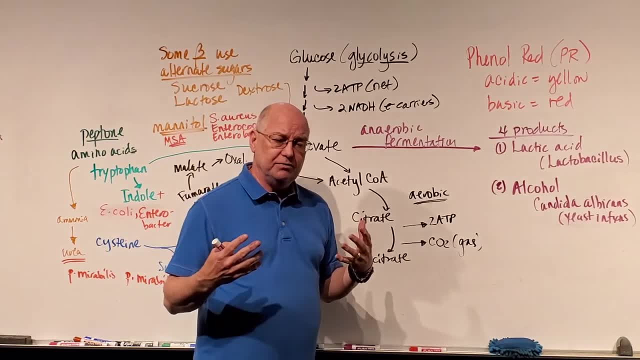 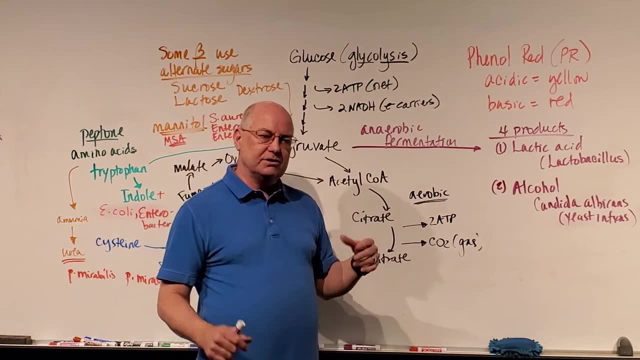 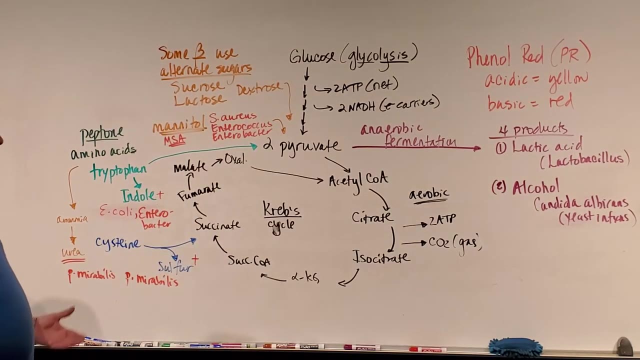 and in very severe cases. some patients have been described as having the symptoms of being drunk, Kind of a loss of balance and sort of a disorientation in things, So anyway, so if an organism ferments alcohol, it could be Candida albicanis. 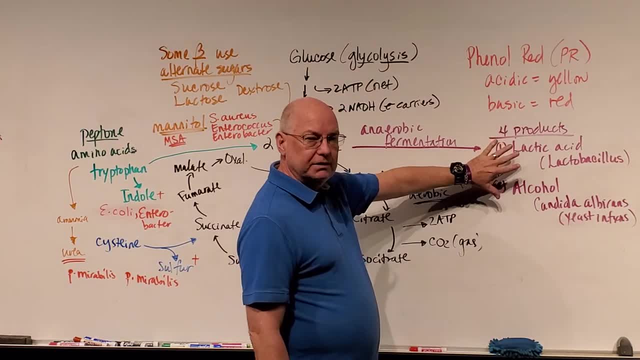 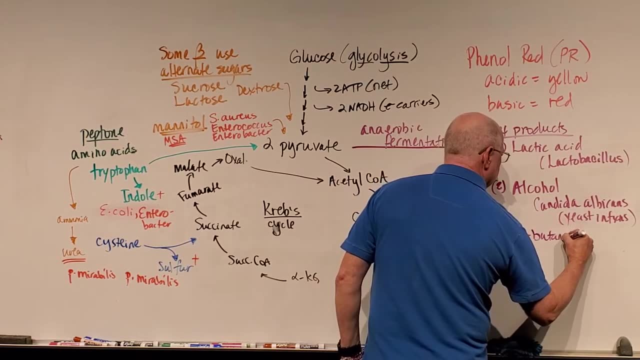 if someone you suspect a yeast infection. We're not going to talk about the tests for these two, but there's another product called 2,3-butane butane diol. This is not an acid, but it's an alcohol. 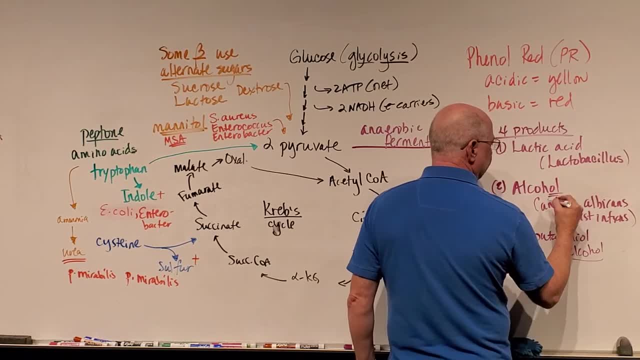 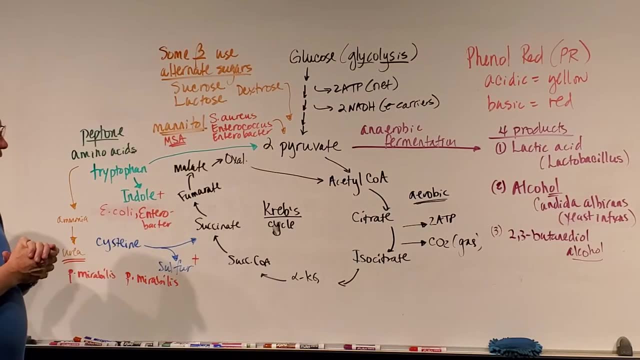 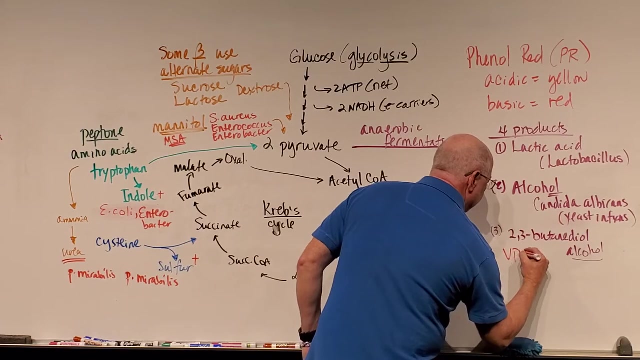 Okay, Alcohol is always and in all OL. Now there's one microorganism that can convert certain sugars into 2,3-butane diol, And when we get this, there's a test that we can run, called the Vogt's-Proskauer test. 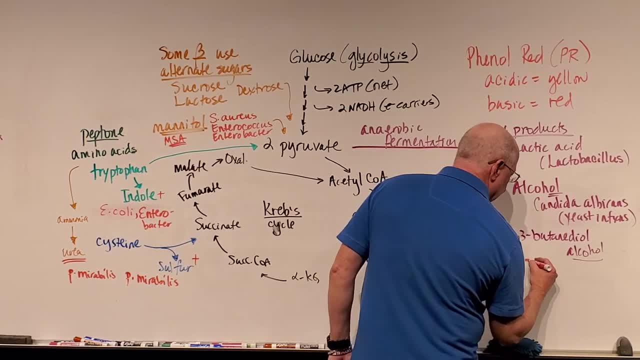 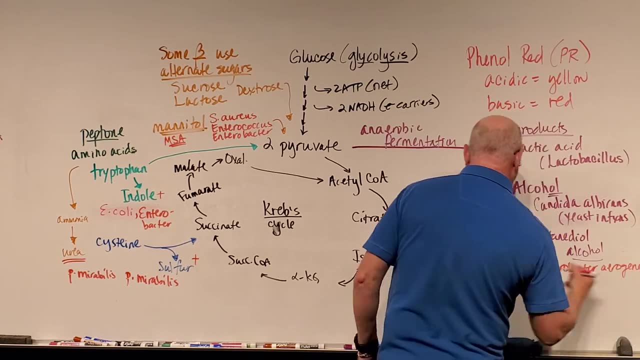 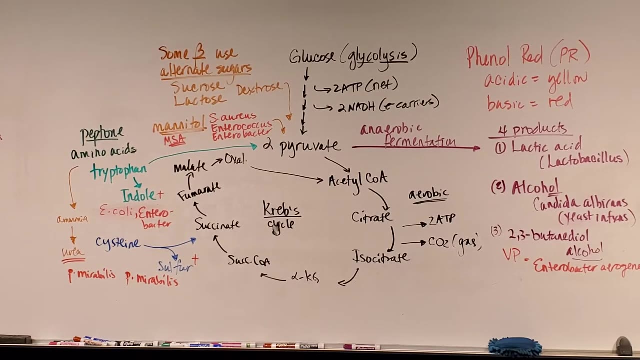 the VP test and it will tell us if there's enterobacter orogenes. So if you run the VP test or the Vogt's-Proskauer test, it can tell us that if we have enterobacter orogenes present. okay, 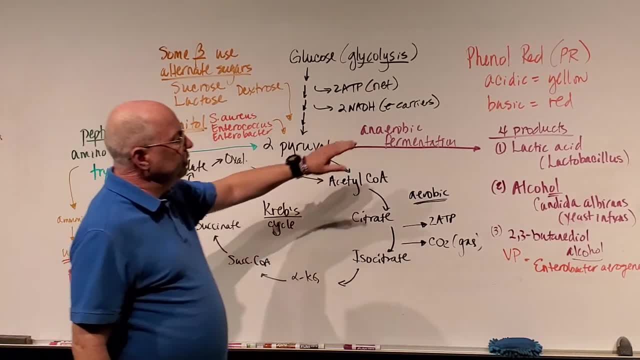 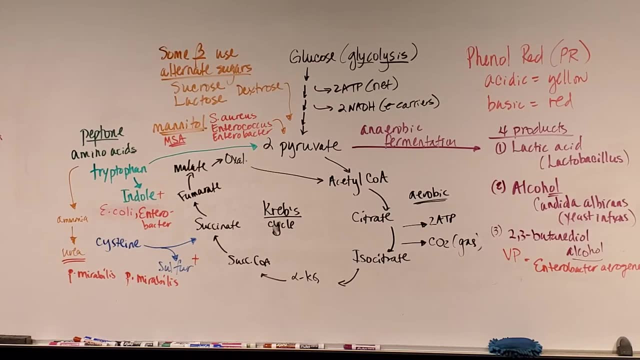 and the VP test uses phenol red. so when we run the VP test, we use a medium that has phenol red in it as our indicator, and if the bacteria produces this 2,3-butane diol, then it will definitely tell us. 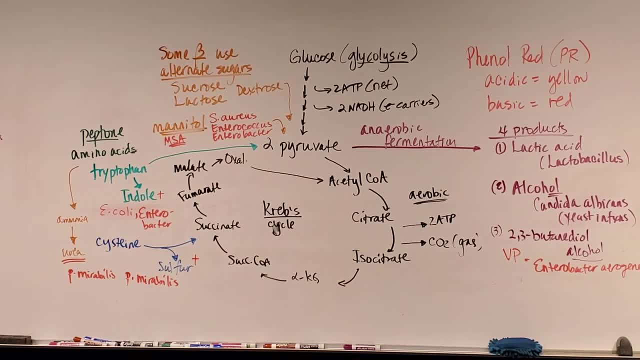 if we have some enterobacter orogenes present. okay, Now it can also be indicative of serratia marcescens and certain tests, and we'll talk about how the test works in a little bit. I don't want to go too far down that road. 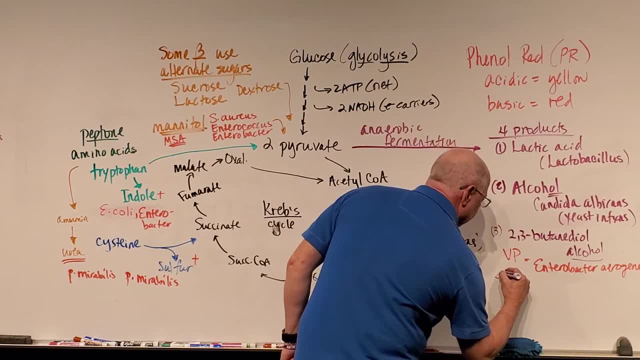 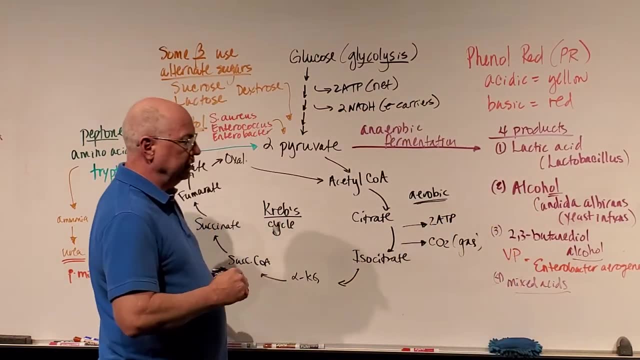 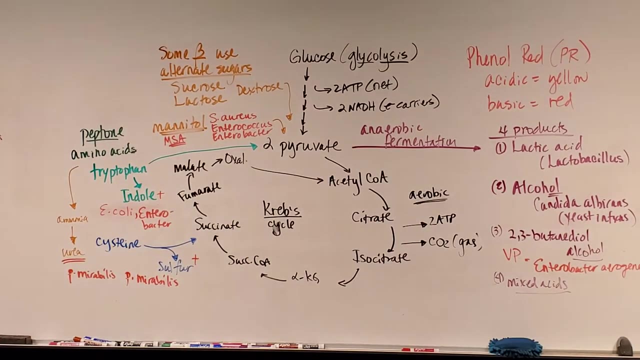 because then it's a whole other lecture, But nonetheless, one of the last products is called mixed acids. We get a mixture of some lactic acids, some other acids and sometimes a little bit of alcohol produced and some bacteria that produce a lot of mixed acids. 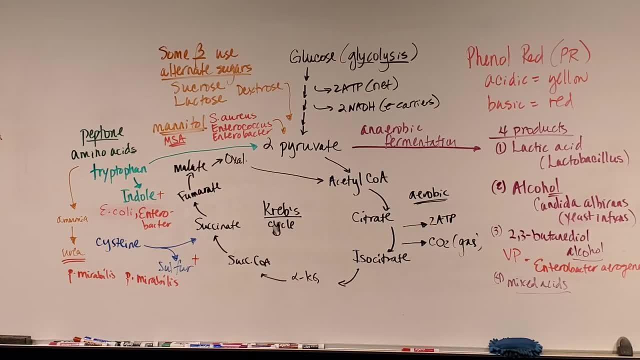 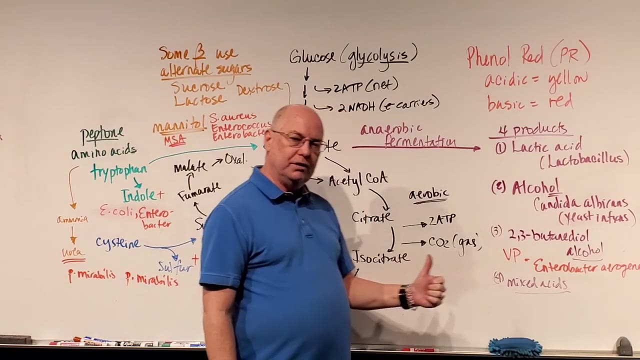 Those acids really have a strong effect in that they're pretty stable acids and they will turn the medium acidic. And a couple of those bacteria that produce mixed acids would be some real bad guys that can cause a lot of infections. E coli is one of them. 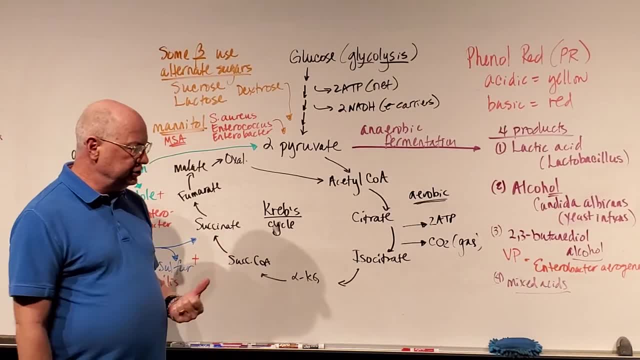 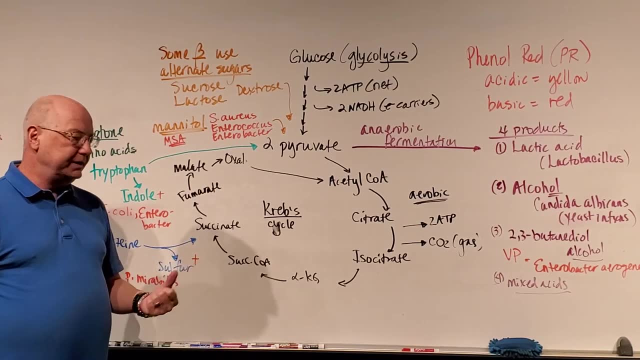 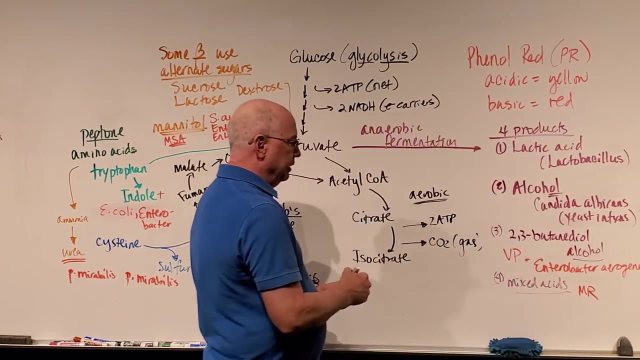 If E coli is in the urinary tract, it can cause a UTI, and so we could run the methyl red test. So the MR test uses methyl red. Now, methyl red is different than phenol red. They are kind of the opposite in how they work. 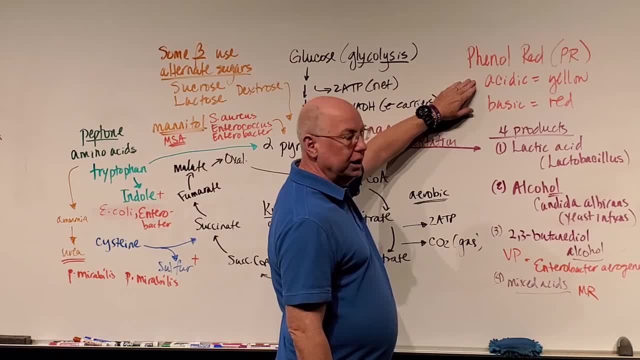 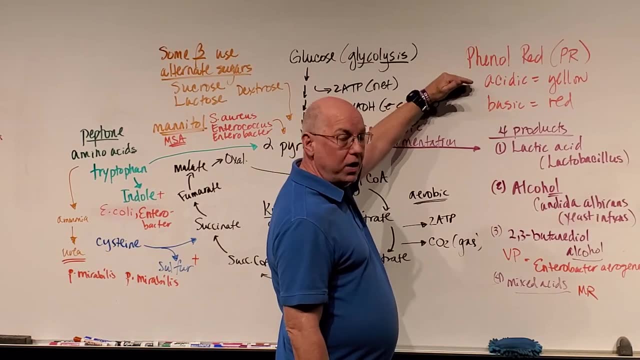 If you look at phenol red, phenol red is yellow when it's acidic and red when it's basic or neutral. essentially, Methyl red turns red when it's acidic and yellow when it's basic. So in the methyl red test, 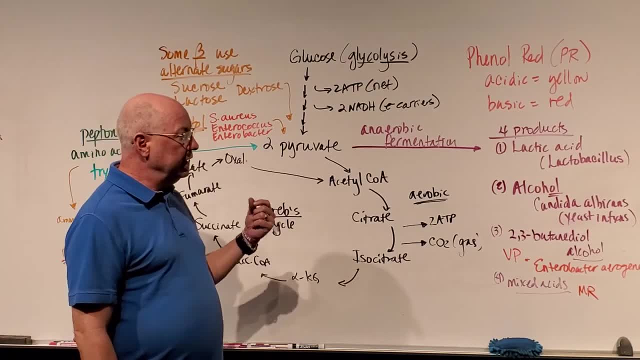 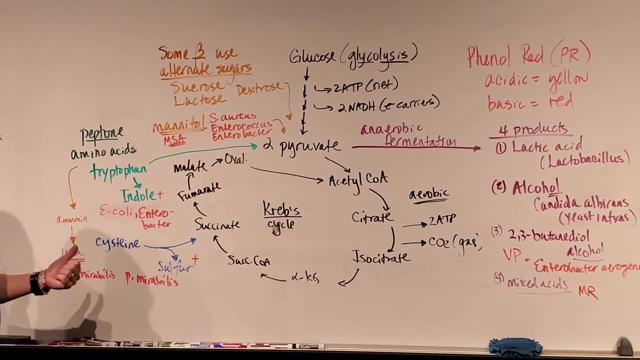 if you add it to the solution and it turns red, then you know that you have an acid fermenter, something that's fermenting mixed acids. E coli is really really good at that. A couple of others that are good acid fermenters. would include Shigella, Salmonella and Proteus species. Okay, And I'm going to stop there because it gets to be too much. So if I get a positive methyl red test, if it turns red and there's acid produced. 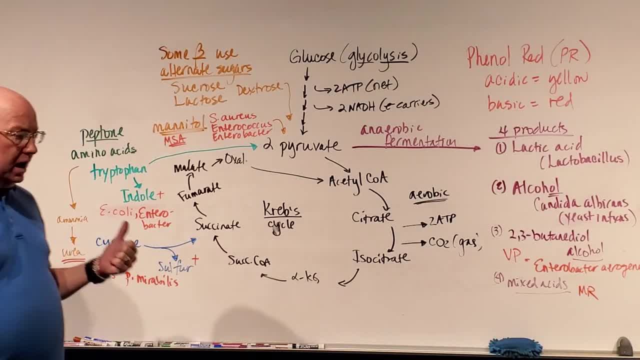 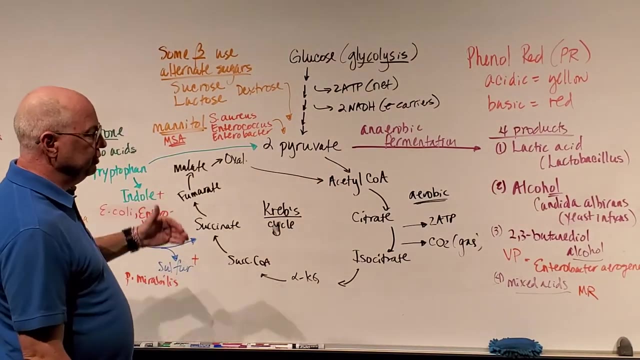 then it's indicative that I could have E coli, I could have some Shigella, I could have some Proteus presence or even some Salmonella. They can all produce positive tests there. So you can see how our knowledge of the fermentation of certain bacteria. 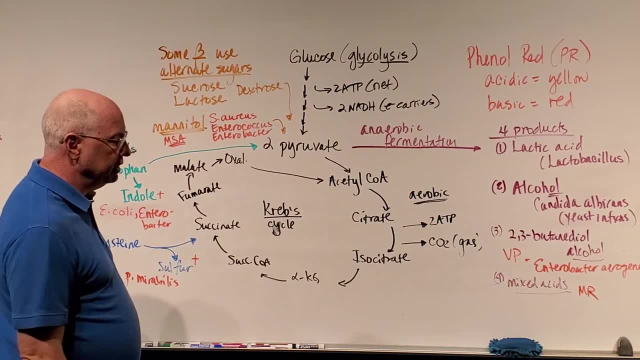 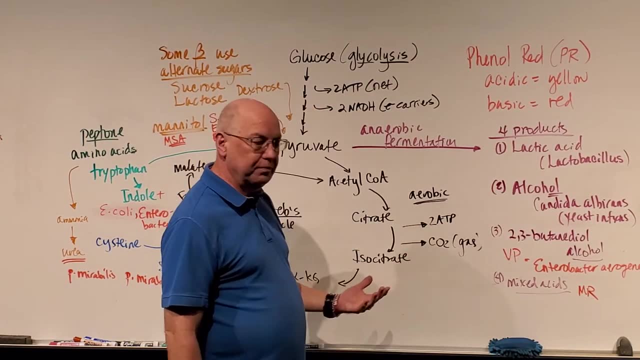 allows us to detect them, setting up some certain tests. The methyl red test will tell us if we have E coli, Shigella, Salmonella, Proteus. The VP test will tell us if it's Enterobacteriogenes. 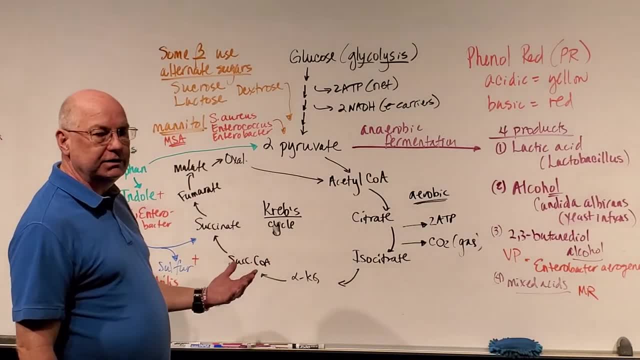 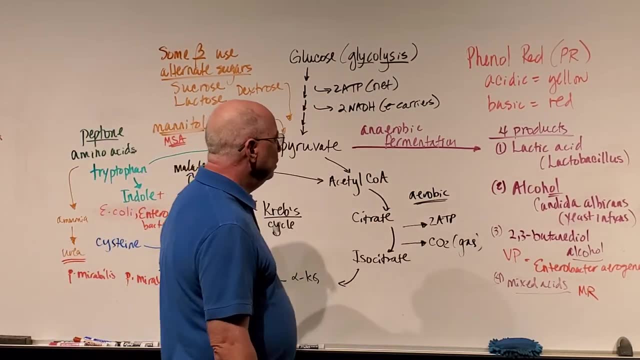 And there are some other phenol red tests that we can talk about in just a moment. Okay, We haven't talked about the phenol red test, but I wanted to knock these out. So if we have some anaerobic fermentation going on, 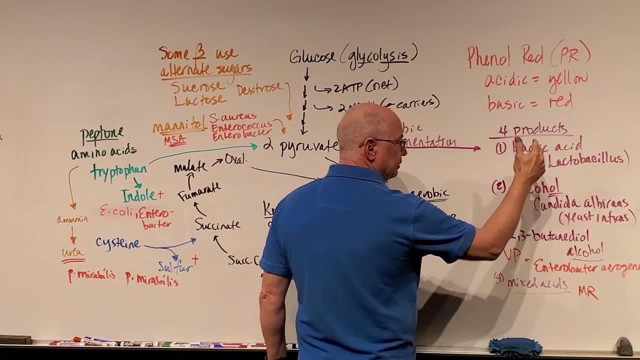 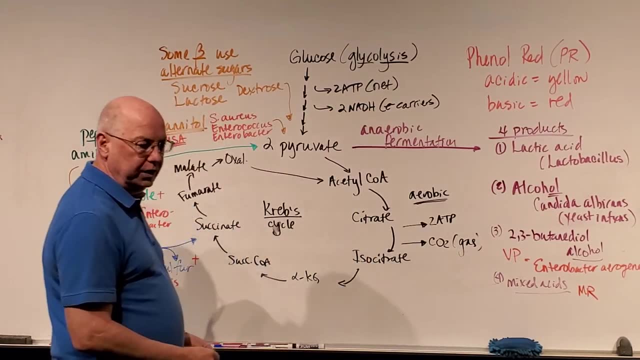 and we're going to produce some acids, then it'll tell us which bacteria are present if we run certain tests. If we produce some non-acids, then we can run another test- Volksproskauer- and add some reagent to it. 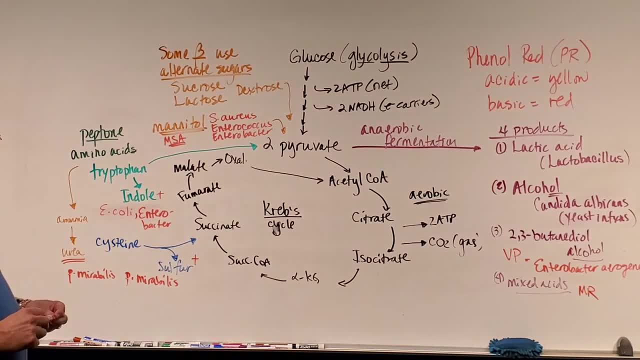 and we get a copper color or get some color change and it'll tell us if Enterobacter is present or not Now. so so far we've talked about mannitol salt, auger If we grow something on mannitol salt. 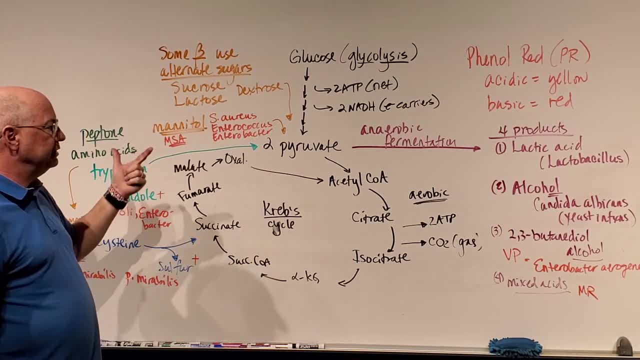 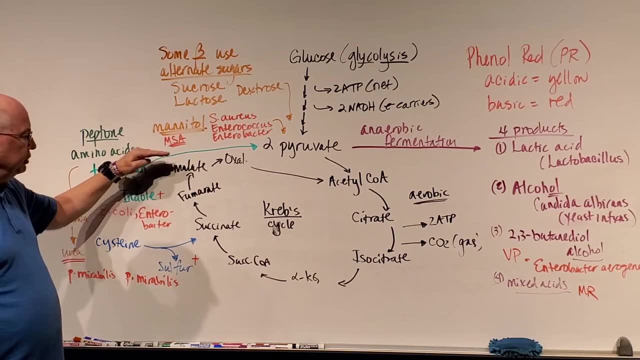 and it grows. it's probably one of these three SRAS, Enterococcus or Enterobacter, If we know. something can break down peptone and particularly the tryptophan in peptone, to produce indole. 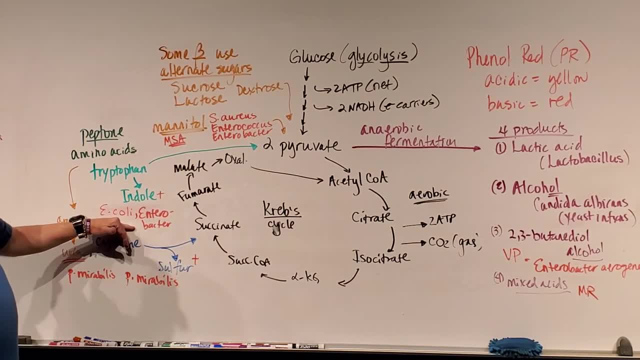 then we know we have E coli and Enterobacter present. So these two tests can kind of confirm and double up, because you don't always just want to rely on one test. What if you've got a bad result? So sometimes we have a lot of overlap in these tests. 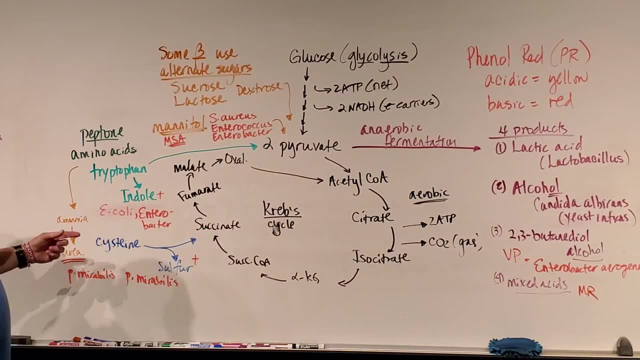 to confirm our results. If we're going to break down cysteine and get some ammonia, some urea or some sulfur, then Proteus Mirabilis. these tests- a positive sulfur test or a positive urea test- will tell us if Proteus Mirabilis is present as well. 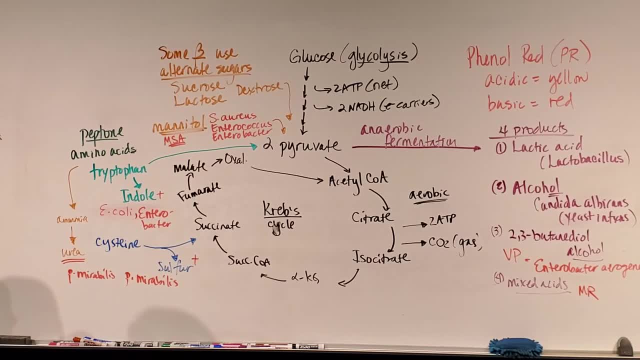 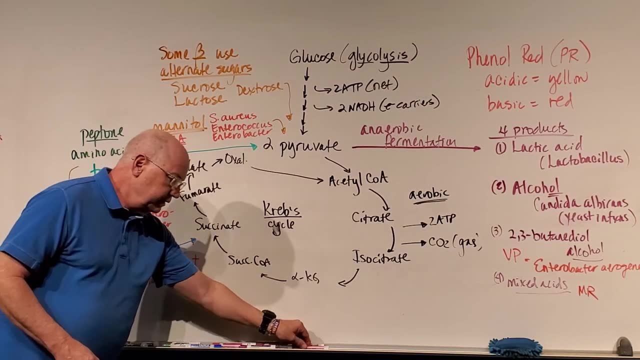 All right, Now I want to get to the phenol red, but I'm going to have to probably erase a few things. Well, maybe not So when we did the phenol red test, there are different sugars that you can add. 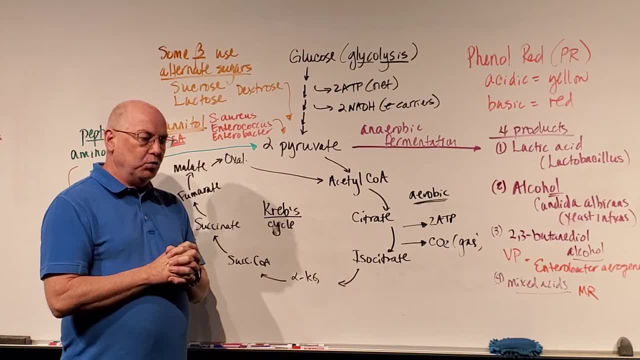 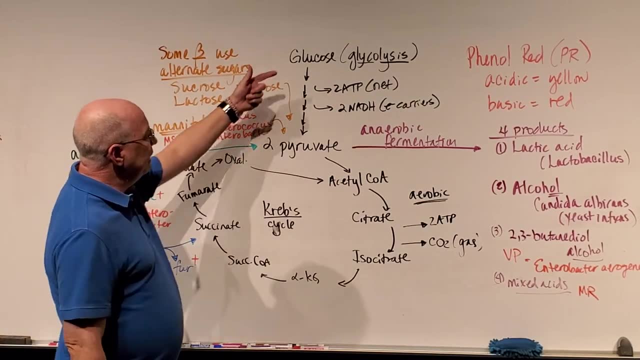 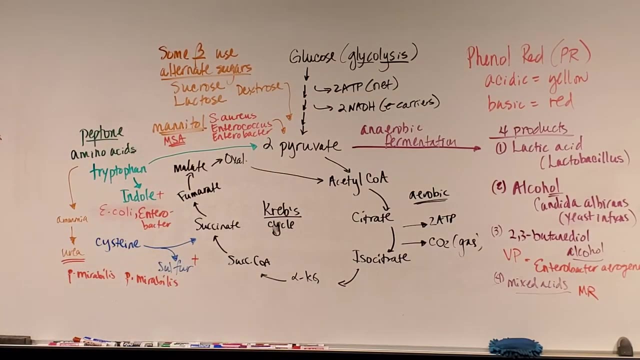 to the phenol red medium. One of them is glucose. So one of the phenol red tests we did was called PRG- phenol red glucose test- And if glucose is broken down and fermented to some acid byproducts then we'll get a positive phenol red test. 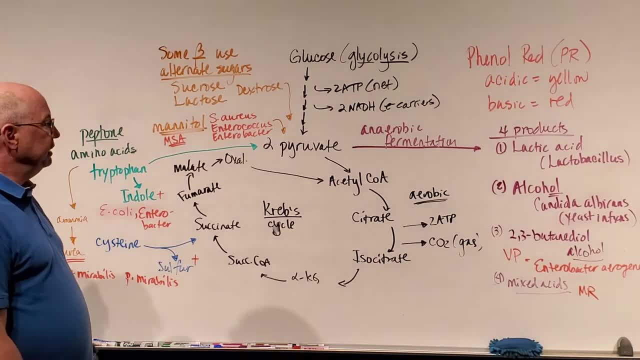 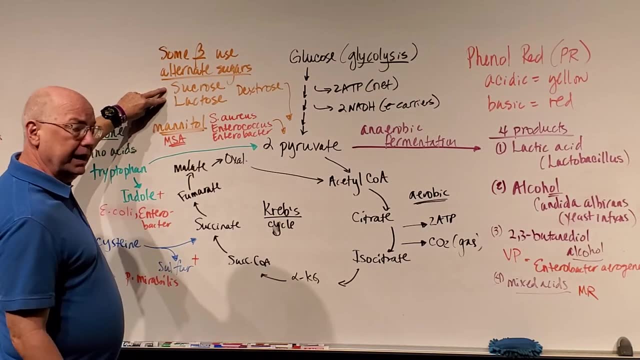 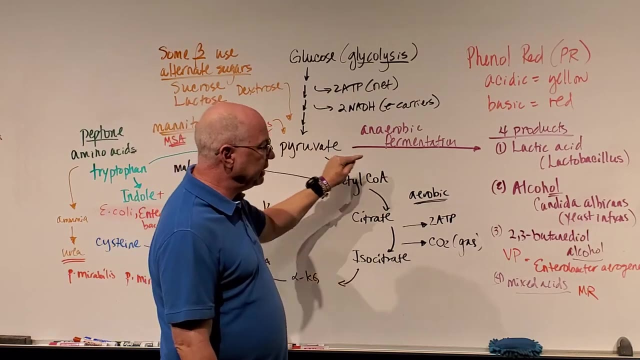 It'll turn yellow if it's acidic. But some bacteria can also break down sucrose or lactose. So in our lab we did a phenol red glucose test and we did a phenol red lactose test And if it can ferment lactose, 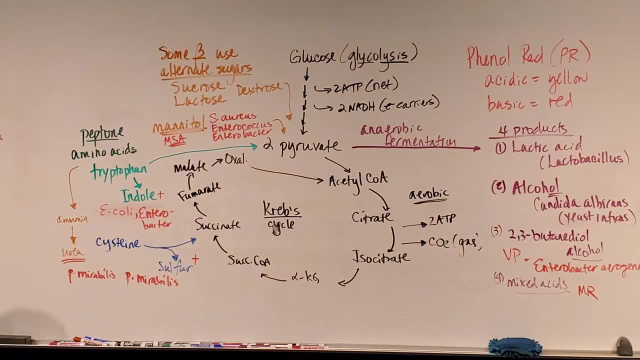 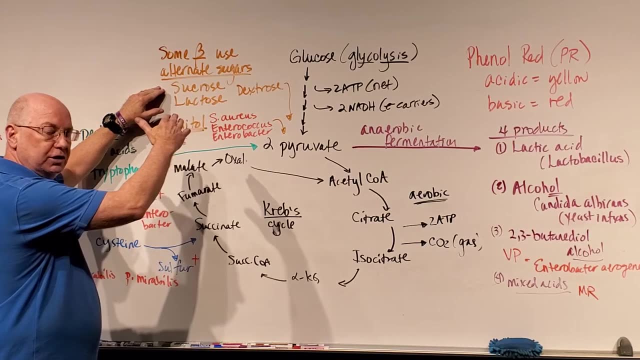 then we'll get the positive test for phenol red, And you can even do a phenol red with sucrose, because some microorganisms can break down sucrose as well. Now I'm not going to go into all the ifs and thens. 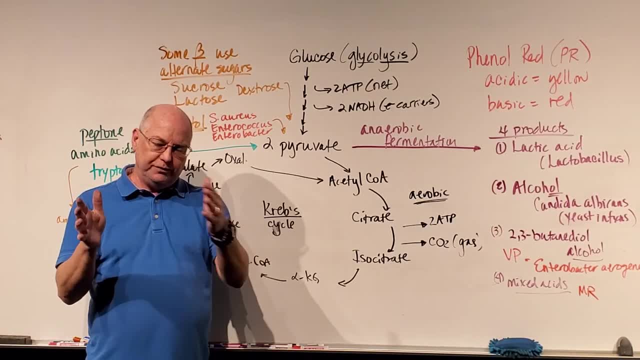 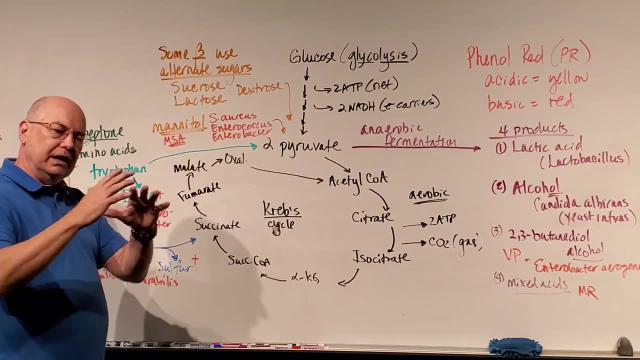 but if it breaks down glucose but not these two, or if it ferments lactose but not the other two, or if it ferments sucrose and glucose but not lactose, it could be All these different ifs and thens can tell us which bacteria is present. 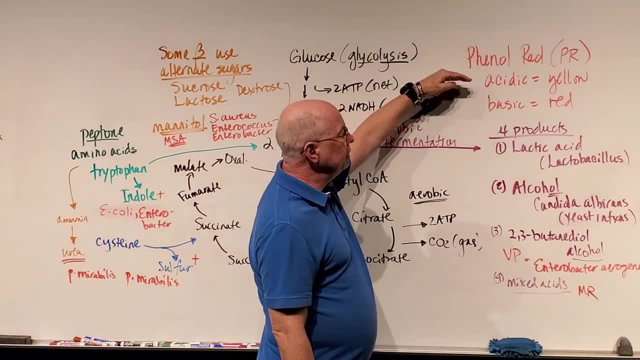 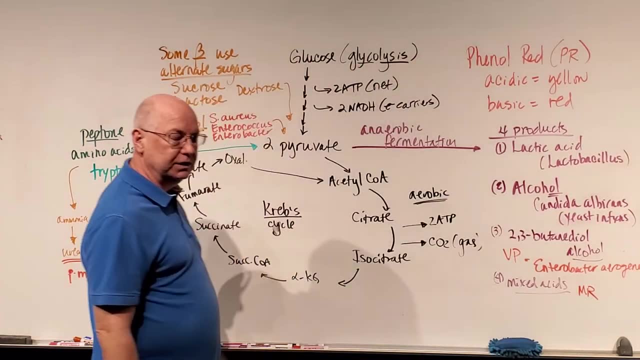 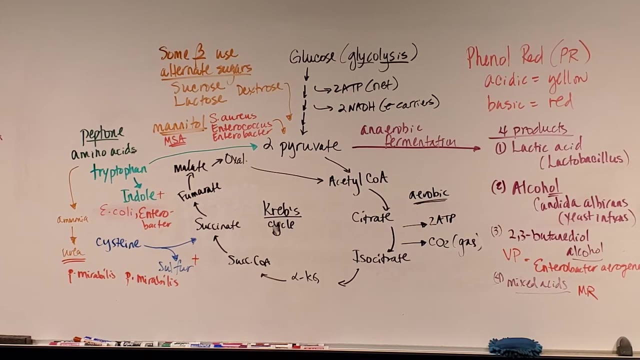 So that's why we do the phenol red test. We're looking for fermentation of sugars into acids. If they're stable acids, then we know these particular microbes are present. Okay, So I'll give you a couple of examples. Okay, 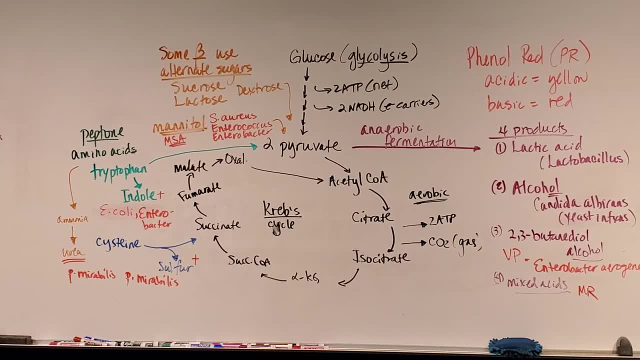 So if we do the phenol red test, Give me a second. I need to take a drink, And no, it's not a drink of ethyl alcohol, Ethanol, It's a drink of coffee. So if we do the phenol red test with glucose, 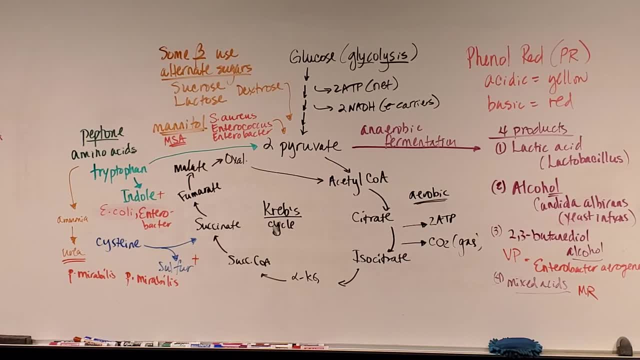 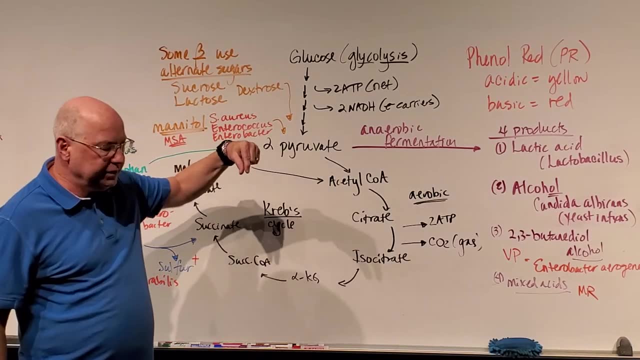 and the bacteria can ferment glucose and produce gas, then it'll tell us some information as to which bacteria are present And some will produce gas. That's why we have the little Durham tube. It'll track the gas in there And if it can ferment lactose and produce gas or not. 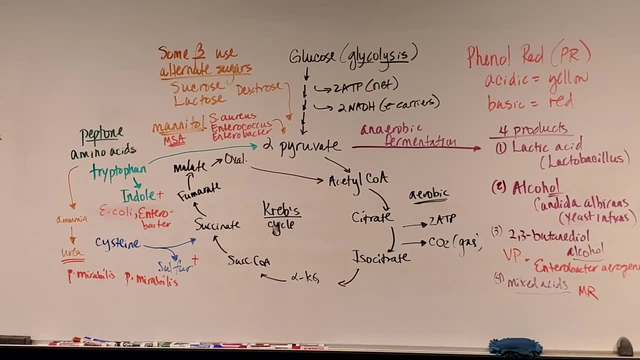 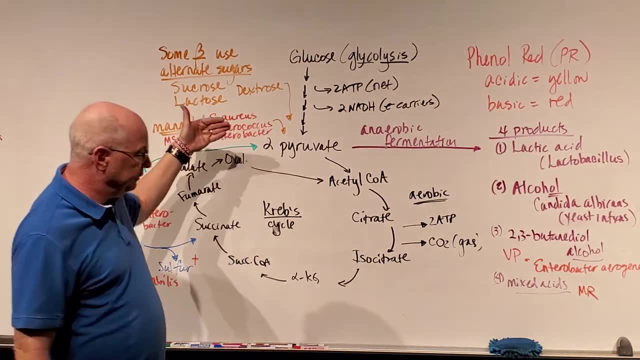 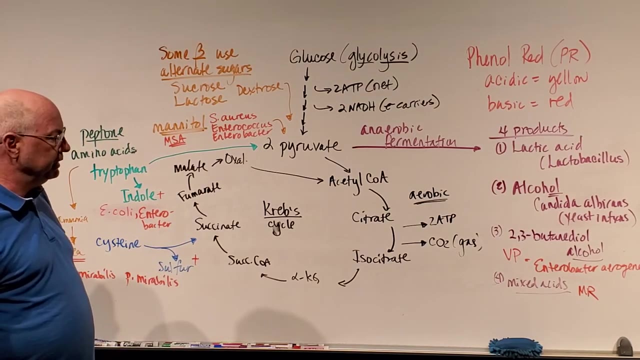 it will then be indicative of certain bacteria. So now we've discussed the phenol red glucose test, the phenol red lactose test, and if we get fermentation and we'll get a yellow color with the phenol red, we know that it's going to be certain bacteria. 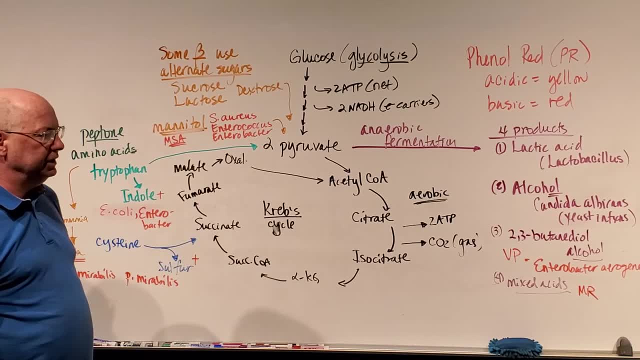 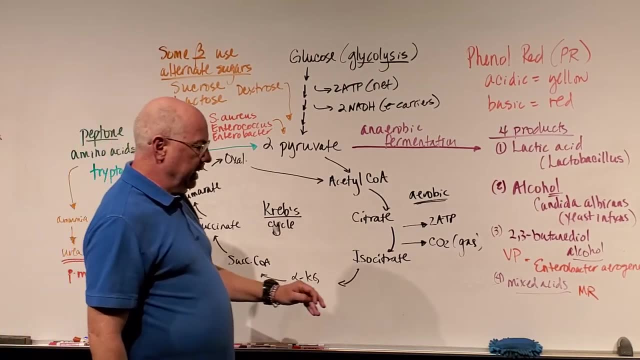 And I'm going to have a whole checklist of this, that and the other, because it's really hard to keep track of all of this stuff. Okay, If we run the MRVP test and the methyl red gives us a result, 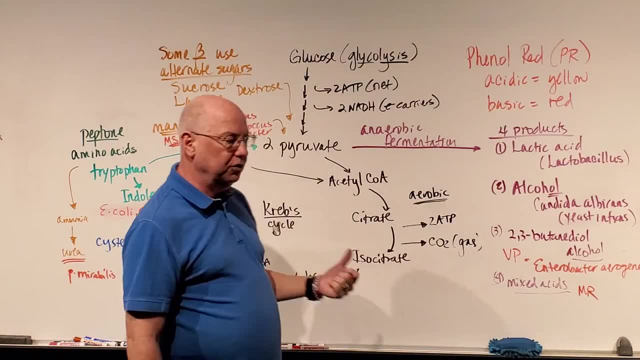 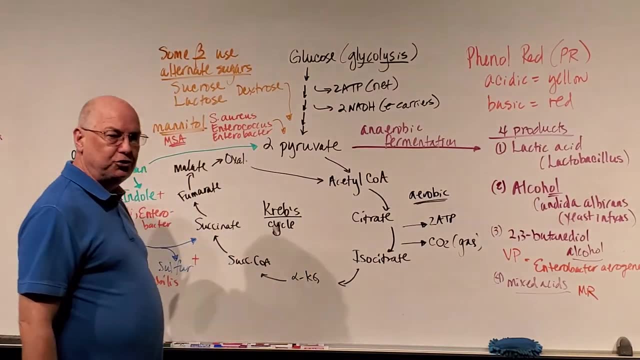 and turns red under acidic conditions, then we know that we have some E coli and enterobacter or maybe a proteus. If the VP test gives us a positive result, then we know we have some. we have enterobacter, orogenes. 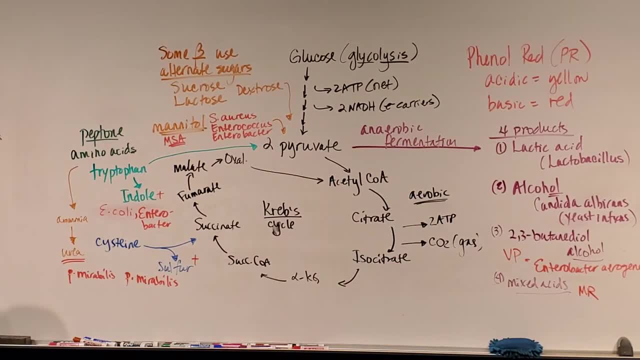 So again, we can figure out which bacteria are based on the results of the test. Now I'm not going to repeat the indole or the sulfur and urea tests, because we all have. we have all those up here. Phenom: 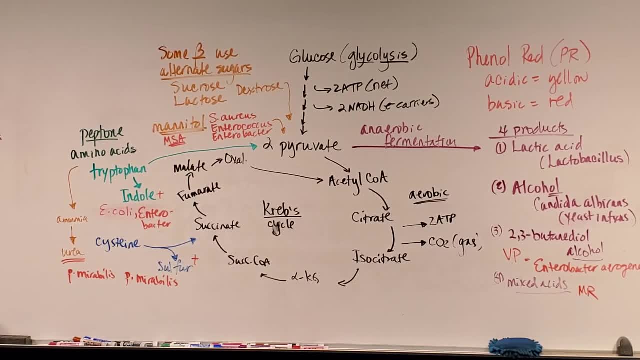 Okay. One of the very last tests that I want to talk about is called the TSI test. Okay, The triple sugar indole test: Okay. So in our triple sugar indole test, one of the things I want you to know about this: 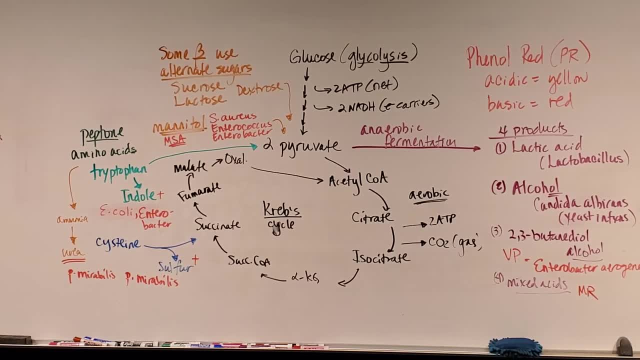 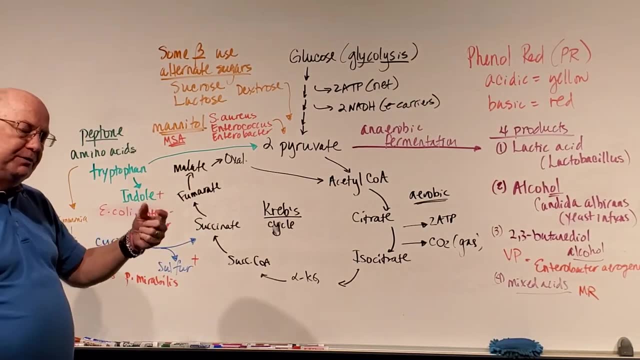 is that? I'm sorry, triple sugar indole. I'm looking here Triple sugar iron test. In the triple sugar iron test, the triple sugar simply means there's three sugars present, And those three sugars happen to be lactose sucrose. 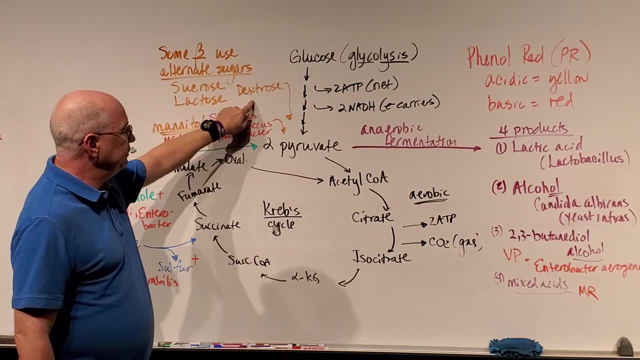 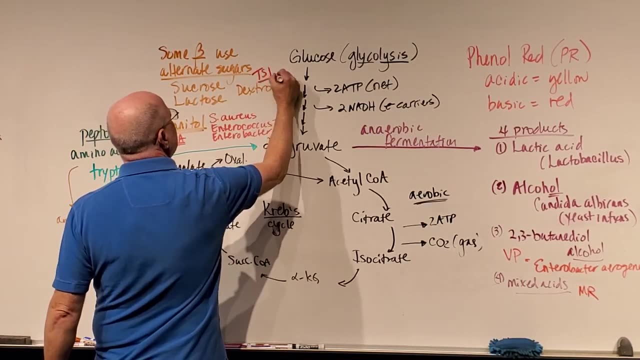 So we have sucrose and lactose and we have a stuff called dextrose. Dextrose is sort of a cousin to glucose. So this is our TSI test: Triple sugar, iron- If these sugars can be converted into acidic byproducts. 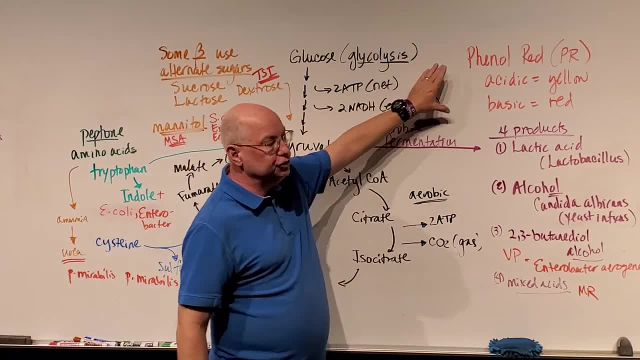 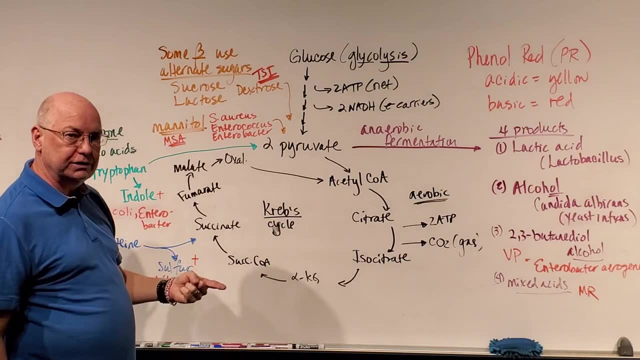 by the way, the TSI test also uses phenol red. That's why I'm talking about it now. So we did three tests that utilize phenol red: Phenol red glucose test, the PRG, the phenol red lactose test. 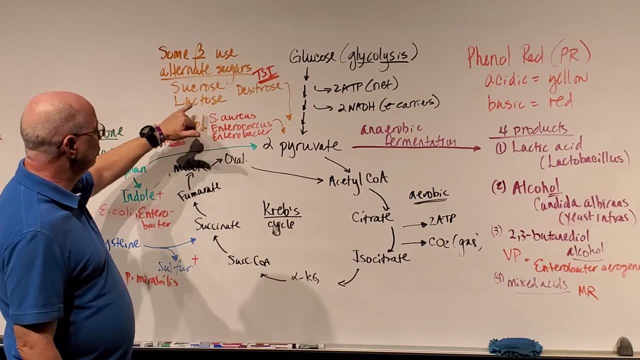 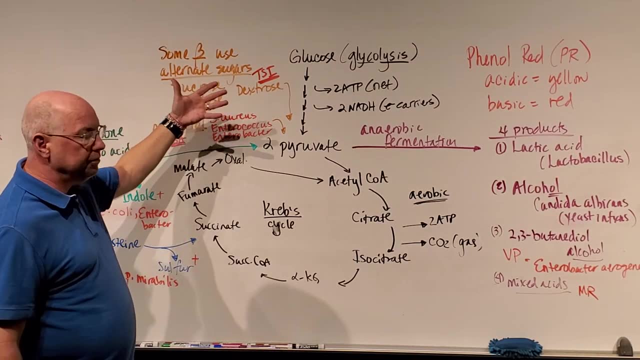 PRL, and then the TSI test which is going to check glucose or its cousin, dextrose, lactose and sucrose, And if those can be fermented then we'll get the phenol. red will turn yellow. 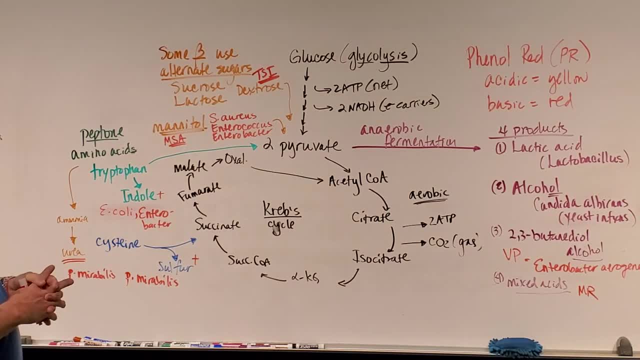 and it will tell us which particular sugars are fermented, based on some other results. okay, Now in this test we can also get gas production, and if there's gas present or not, we'll give us some information. but I'll go over that in just a second. 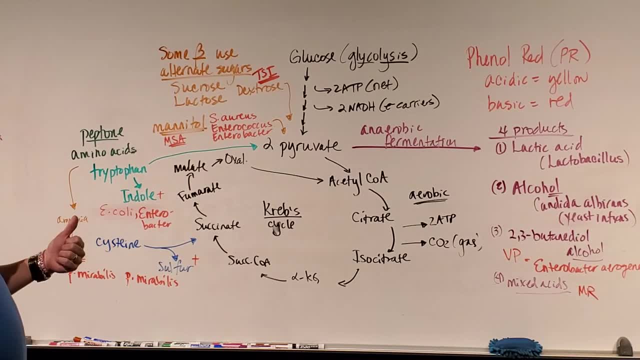 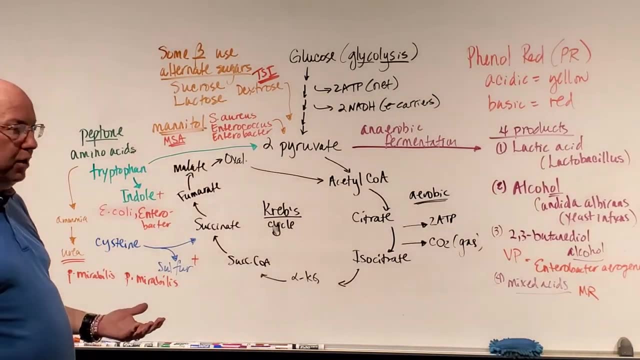 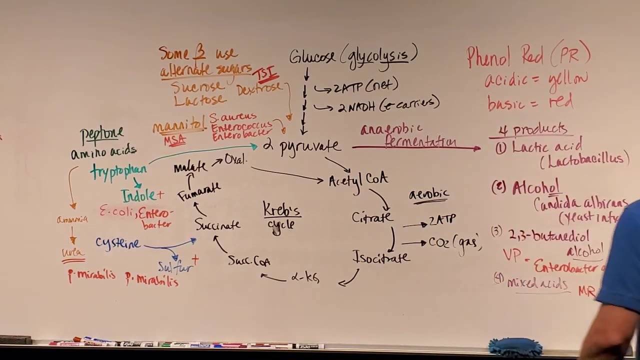 The iron part of the test is this: If you have something that produces sulfur and sulfur interacts with the iron, then it can tell us if we have proteus mirabilis present or not. okay, So now when we do the triple sugar iron test, 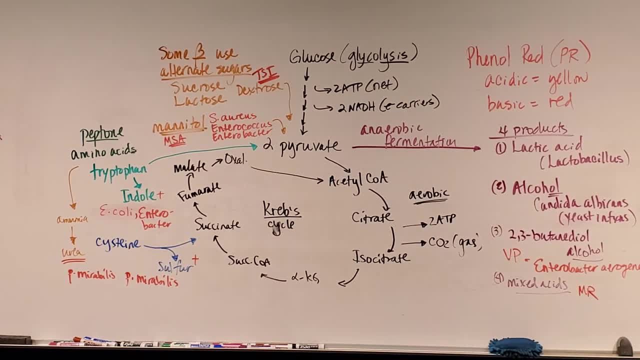 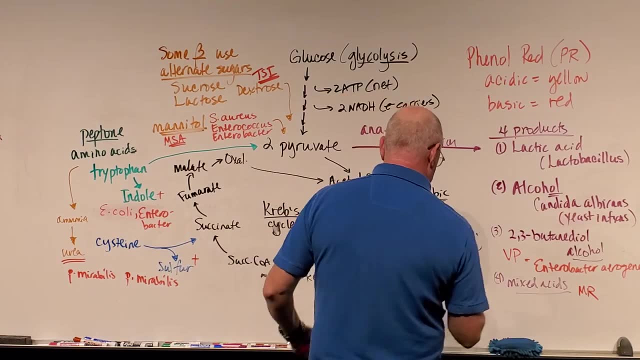 one of the things that you'll see- and I may step off screen here for a second, but one of the things that you see in the triple sugar iron test is that in this particular test we used a tube that was a slant. 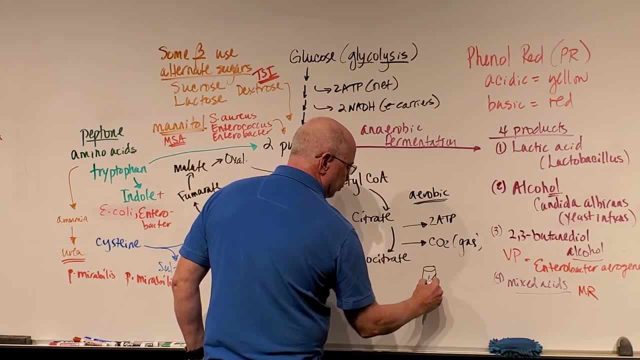 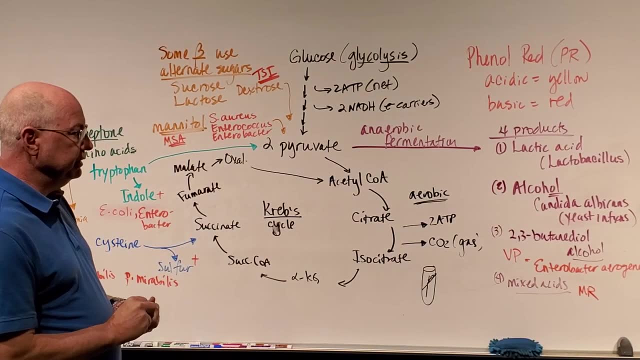 but what we did was we stabbed the tube and then, as we withdrew the needle, we dragged it on the surface. We're checking for aerobic and anaerobic metabolism, okay, And so in the TSI test, what we can do is: we can see. 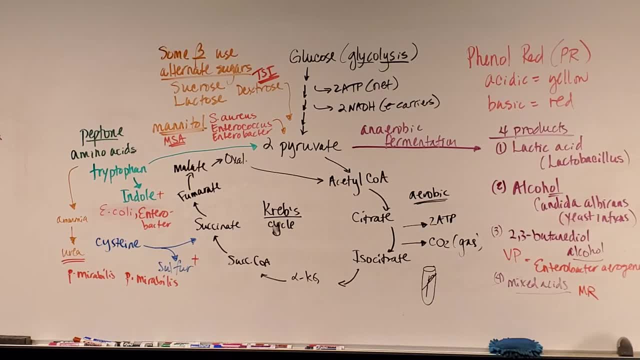 if the phenol red turns yellow, we know that the sugars were fermented into acid. Now what happens is this: If we ferment dextrose, the way that the tube is set up is that there's a little bit of dextrose. 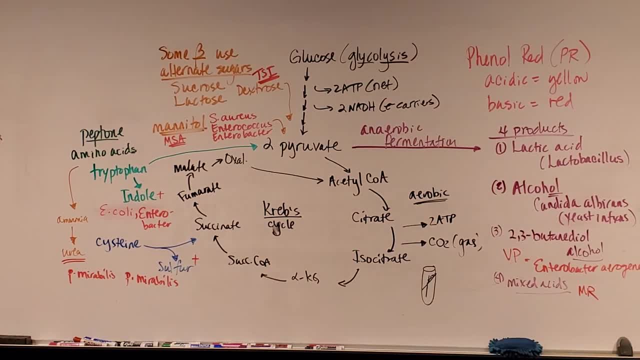 but not a lot, and after a while the dextrose will be exhausted and as it's broken down in air, then the tube will revert back to sort of a negative result, and so we'll get red on the surface but the bottom of the tube. 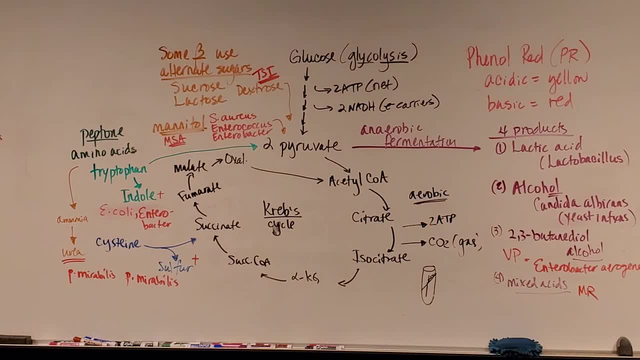 or what we call, the butt of the tube will remain yellow. So if it ferments, dextrose only, we get red on the surface, but yellow in the butt. If it ferments the other sugars, lactose or sucrose. 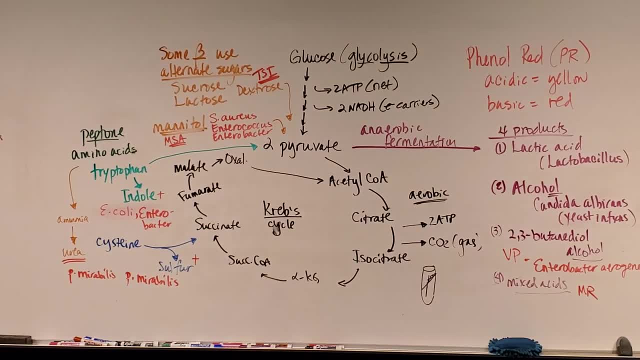 the whole thing will turn yellow, okay. If nothing turns yellow and the whole thing stays red- both the slant and the butt are red- then no fermentation occurred, okay. So finally, if the organism produces hydrogen sulfide and that interacts with the iron, 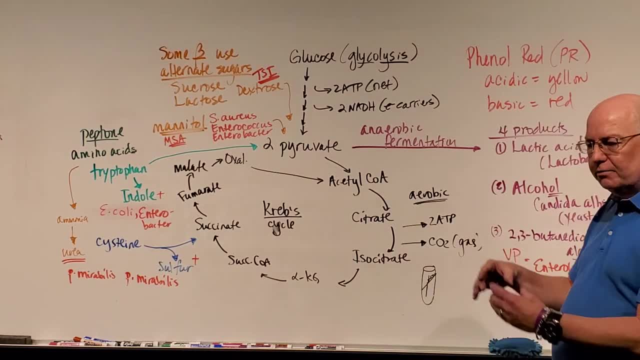 then we'll get a black precipitate in here and when you look at the medium you'll see whether you get. the whole thing is red, no fermentation. you get yellow and yellow, the yellow slant and yellow butt. then fermentation of lactose and sucrose occurred. 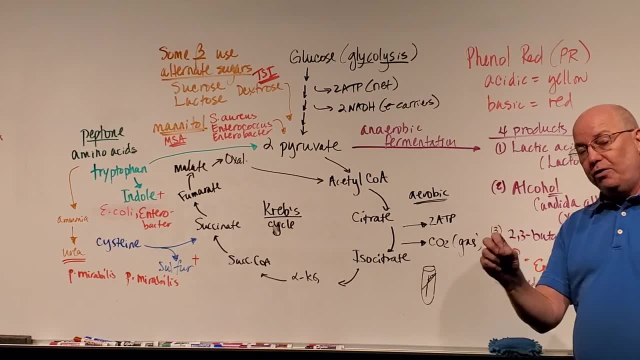 If I get red slant and yellow butt, then we fermented dextrose, and if we get the fermentation of dextrose and hydrogen gas produced, then what we're going to get is a black precipitate. okay, So anytime the hydrogen sulfide is produced. 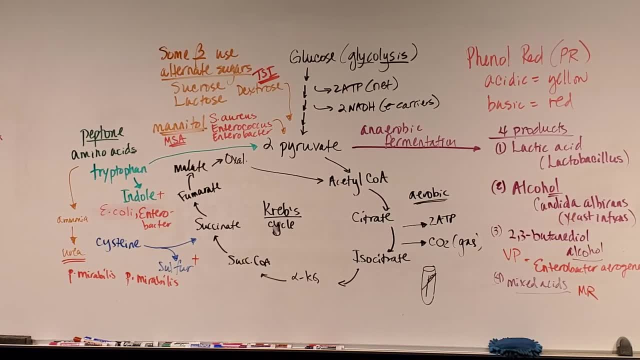 we get a black precipitate. okay, I think that's what I want to tell you, and that's about it. So I guess I could tell you this: a couple of bacteria that are culprits here: If we get yellow and yellow. 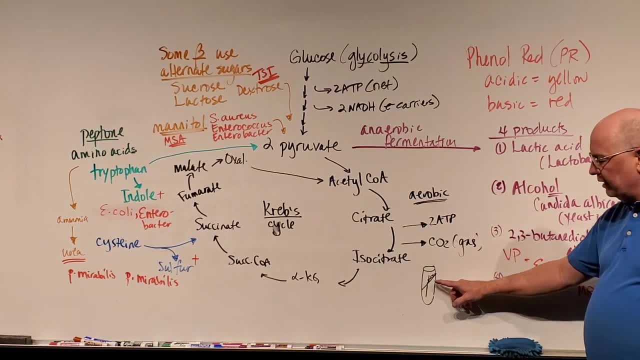 okay, you might want to try to take note of this. I don't have any room to write it down and I'm going to have this printed in some notes for my students. but if I get a yellow and a yellow and some gas is produced. 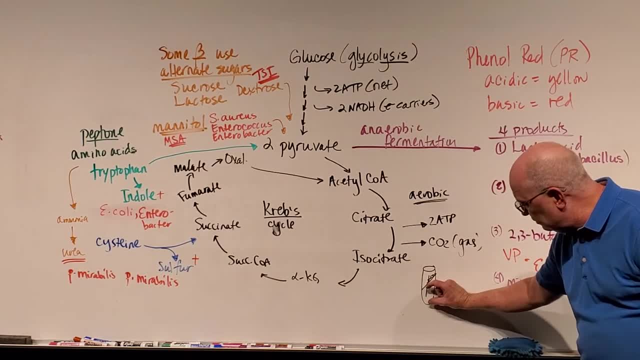 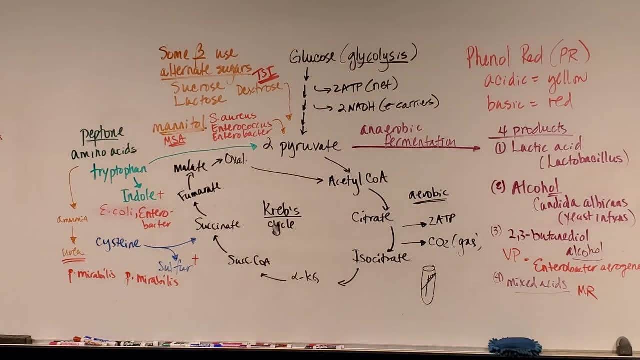 so the two. if we produce gas at the bottom of the tube, the media can be lifted or have cracks running through it. If we get yellow and yellow with gas, then it's going to be like E coli. the three main culprits would be E coli. 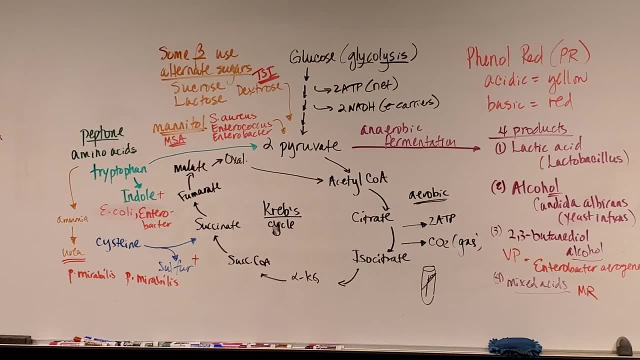 Klebsiella pneumoniae, which can cause pneumonia or Enterobacter. If I get red up here on the slant and yellow in the butt, then I have a glucose or dextrose fermenter and if I don't, get any gas produced. 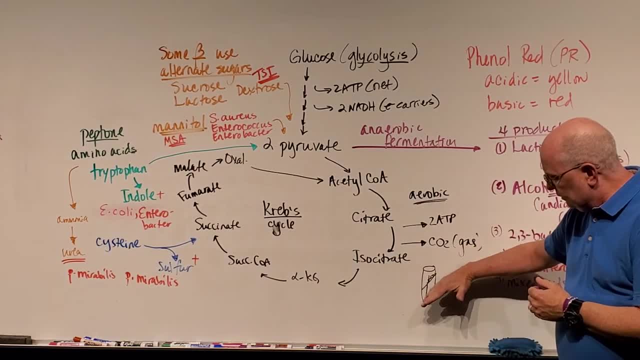 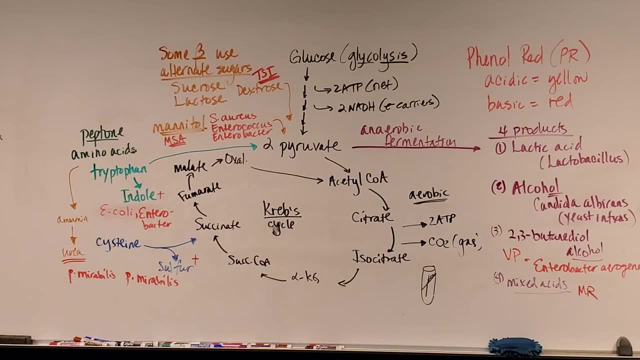 so if I get red, red slant, yellow butt with no gas produced, then the culprit is probably going to be Shigella or Serratia marcescens. okay, If I get red, and yellow, red slant. 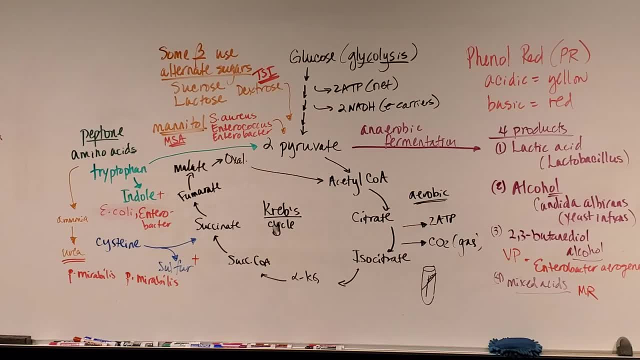 yellow butt, but I do get gas produced and it's lifted or cracked in the media. then I know I have Proteus, some kind of Proteus like Proteus vulgaris or Proteus mirabilis, and or I could have Salmonella present. 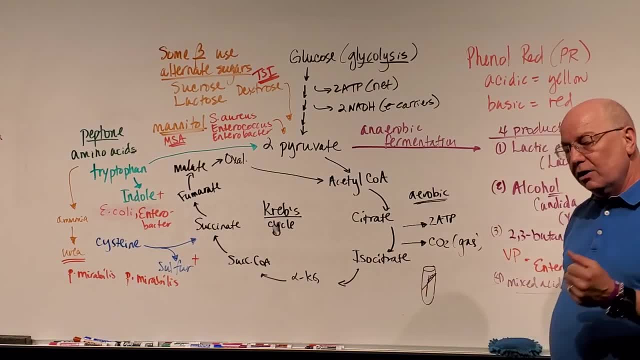 and if I get nothing but all red, usually the culprit is a stuff called Pseudomonas aeruginosa, or we know it's not any of the others. So the triple sugar iron test tells us a lot. Number one: it tells us which bacteria are present. 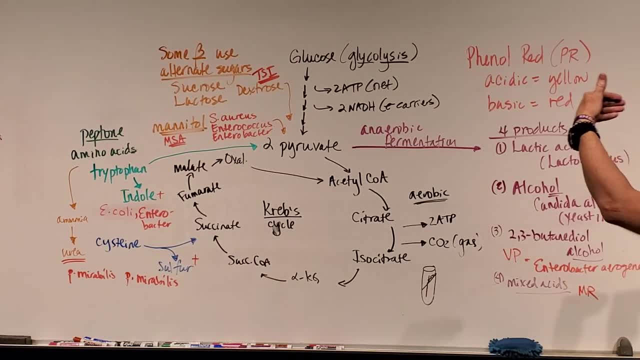 based on this whole grid, that we can do. is it yellow? yellow with gas yellow yellow, no gas red. yellow with gas, red- okay, If it's all red, there's no fermentation. we got Pseudomonas aeruginosa. 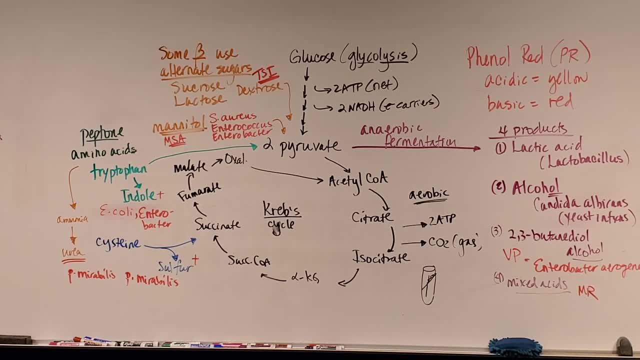 If we have yellow, yellow with no gas, then it broke down to lactose or sucrose, and we have, I'm sorry. if we have yellow yellow with gas, then it broke down lactose or sucrose. it's E coli. 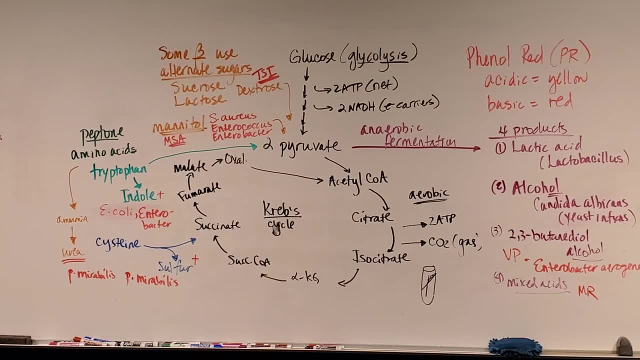 Klebsiella, pneumoniae or Enterobacter. If it's red, yellow and no gas, then we get the fermentation of dextrose, and and that would be Shigella or Serratia, and if it's red and yellow with gas, 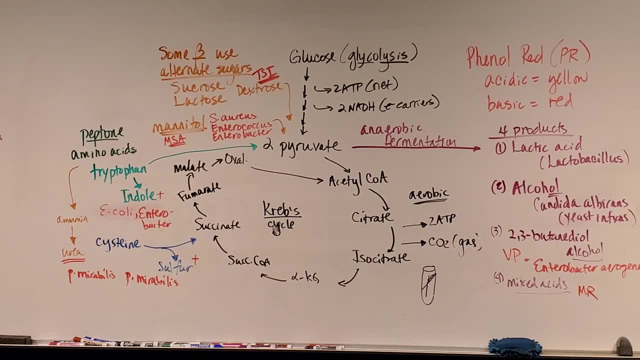 then it's Proteus or Salmonella and I think that's all the ones I want to cover. And of course, if we get hydrogen sulfide and it produces a black precipitate, then we know hydrogen sulfide was was produced. 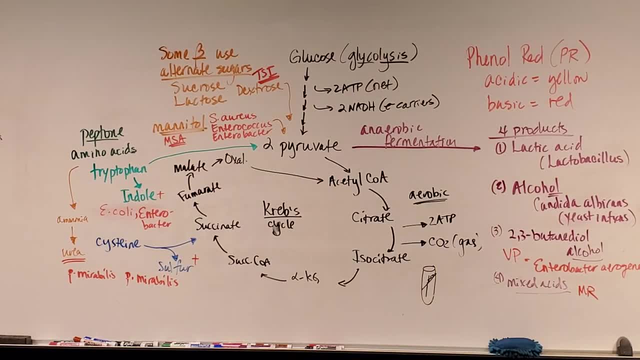 and it could be Proteus mirabilis. okay, And that's a lot, and it's a lot to keep track of and a lot to memorize, but I think I've gone over all the tests. So we have phenol red with glucose. 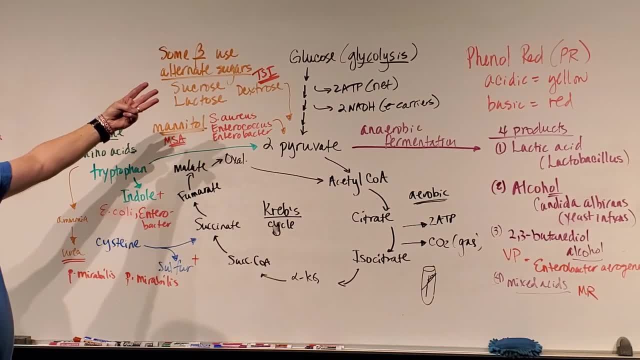 phenol red with lactose. we have the TSI test, we have the indole test, we have the urea test, we have the MR test and the VP test and I believe that's all the tests that we run in class. 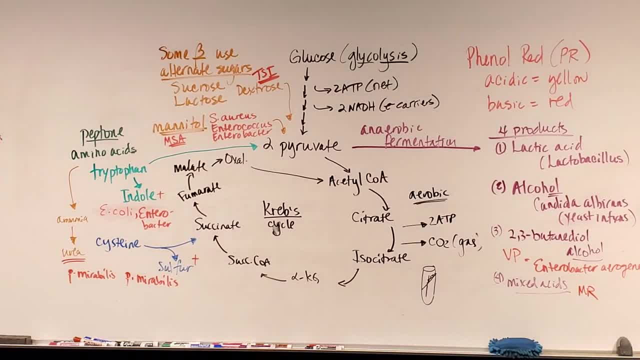 Let me take one look at my notes. Let's see we got PRG, PRL, TSI. MR VP, the SIMS test- Oh, I forgot the SIMS test. The SIMS, the sulfur indole motility. 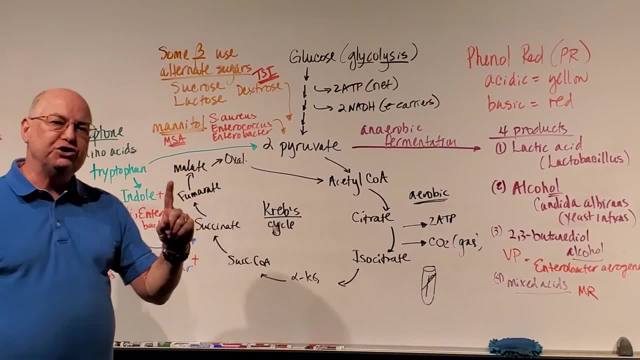 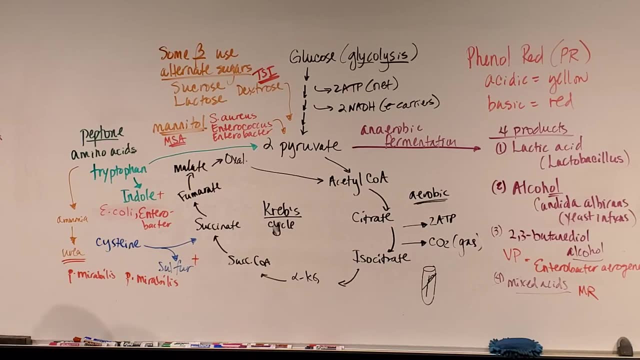 We covered that one. Oh, I know which one I'm missing: The citrate test, citric acid. okay, So in the citrate test, also called the Simmons citrate test, we're looking to see. we're looking to see which bacterium can simply break down: citric acid or citrate. 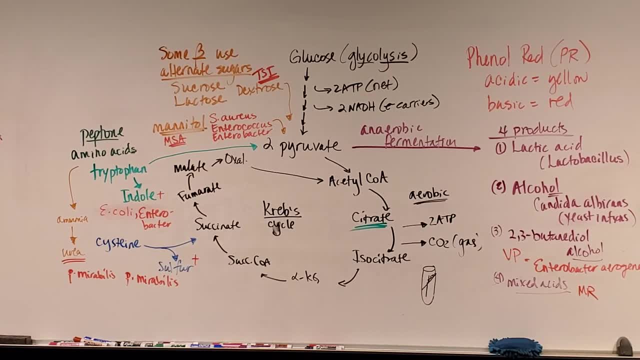 Now, only a couple of bacteria can use citrate as their sole carbon source, And what happens is, as they produce carbon dioxide in this process, that carbon dioxide can interact with other compounds and produce a base. okay, And that basic. 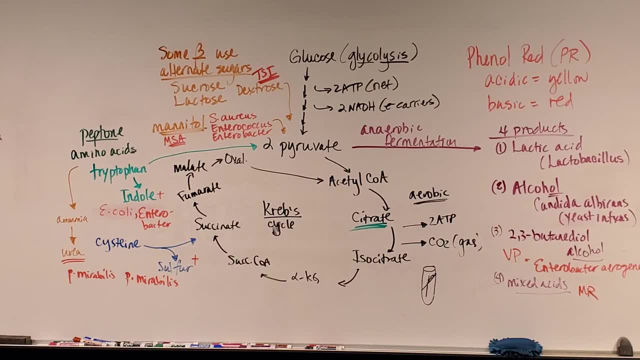 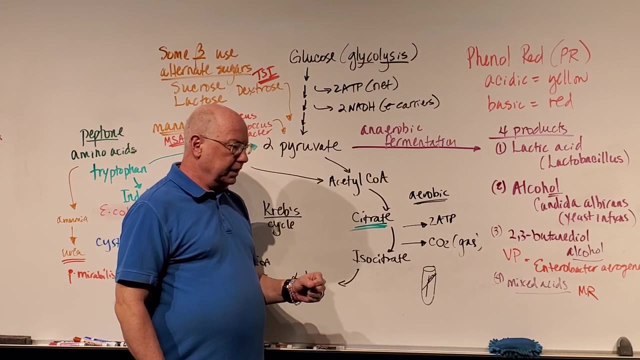 uh compound will turn the pH indicator um, which is called bromothymol blue, from green to a royal blue color. So the last thing, what we did, was the citrate test. We have a slant there and um. 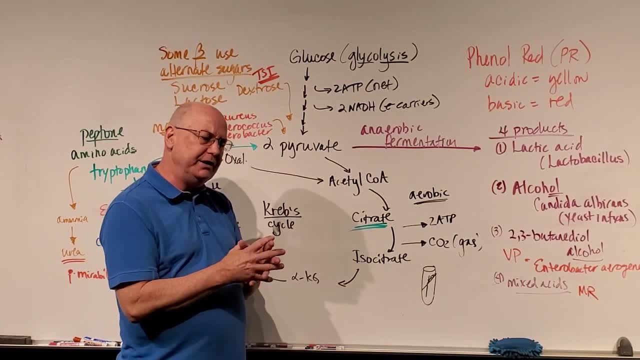 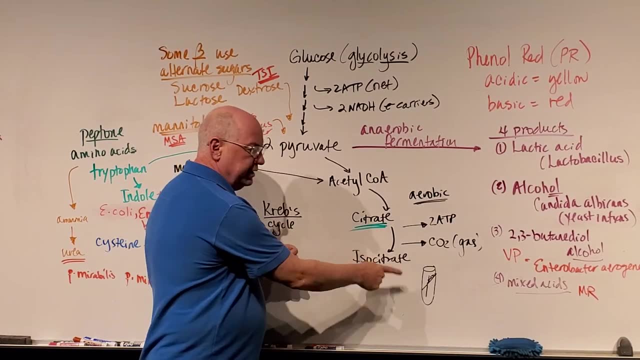 the slant had a greenish color, sort of a blue green color to it, um, like a sea green color. And that auger. if the bacterium can break down the citrate in that auger, it will turn the auger from. 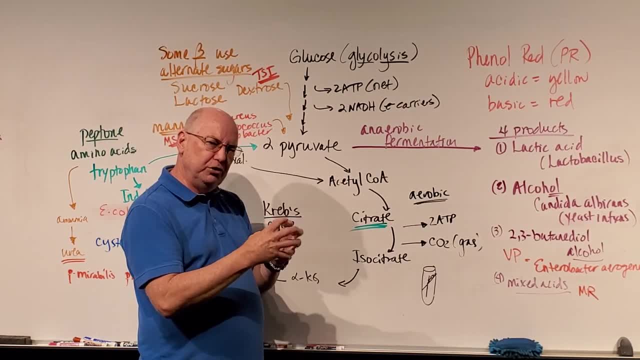 from the sort of bluish green to a very, very beautiful, bright blue color. And so then we know that citrate was broken down And, um, one of the things to note about that is in the citrate test, if you do get a positive result. 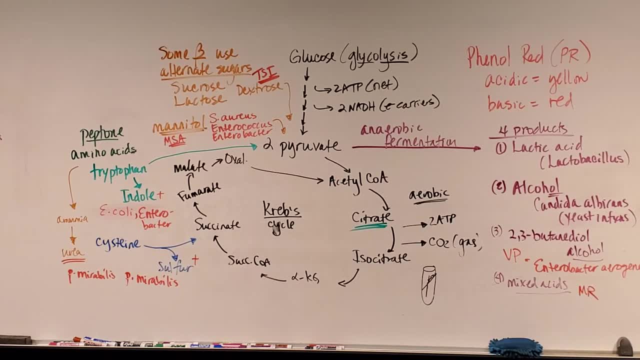 um, then you know that you have Parotius mirabilis or Klebsiella pneumoniae. So Parotius mirabilis can also break down, citrate and, and, and, and, and, and, and. 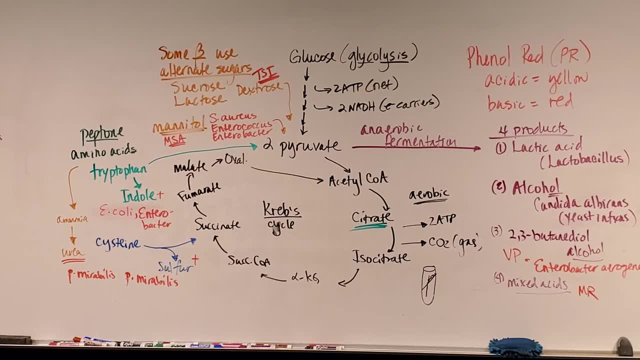 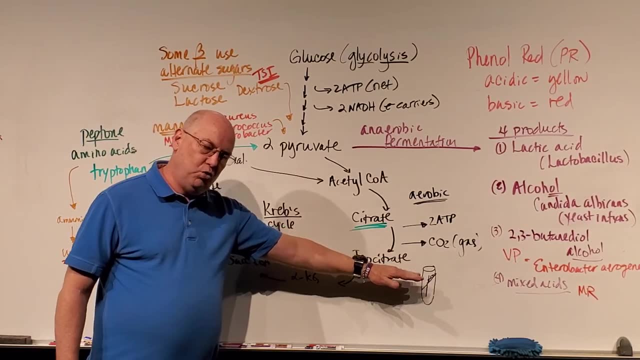 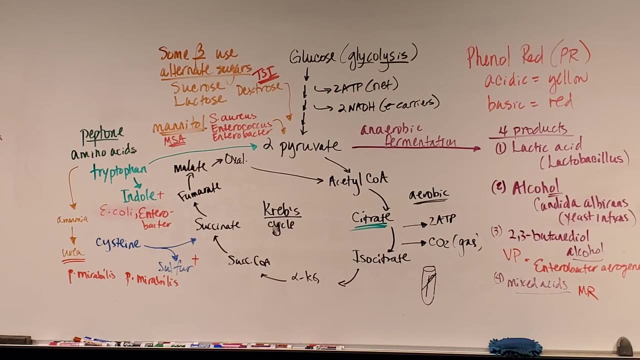 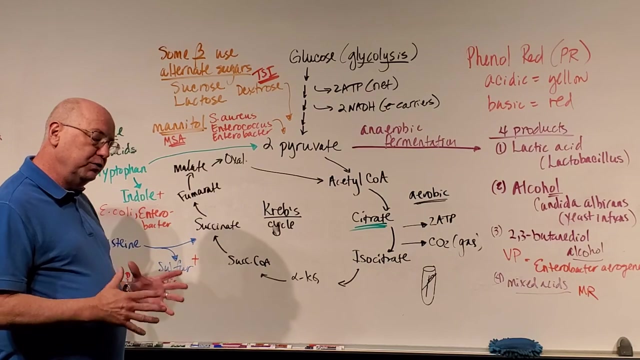 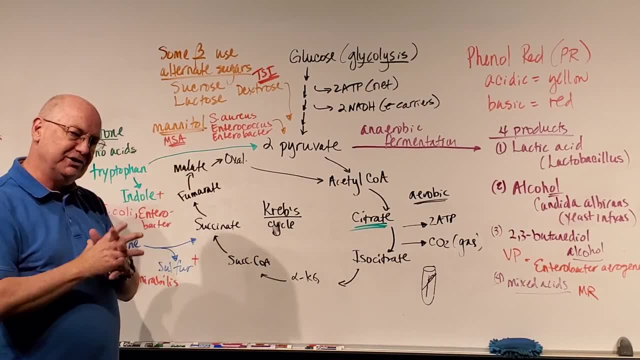 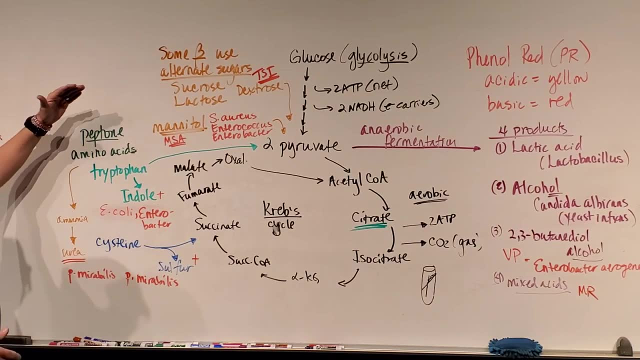 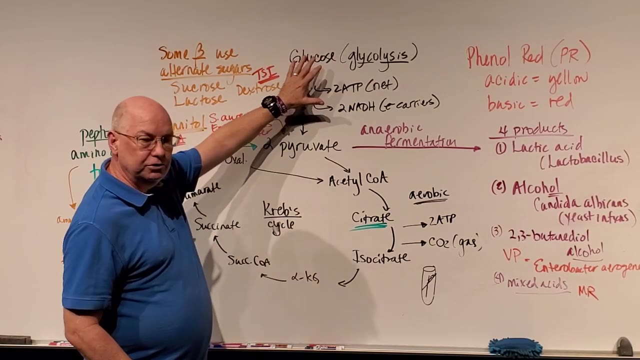 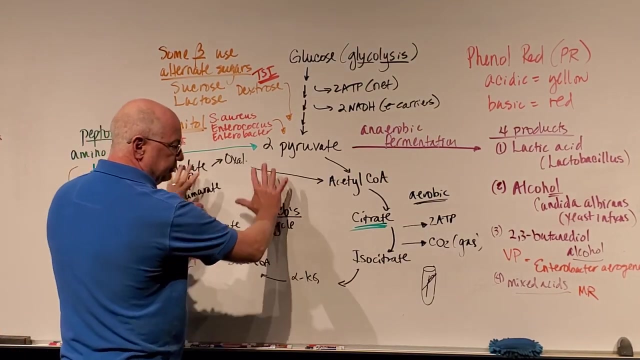 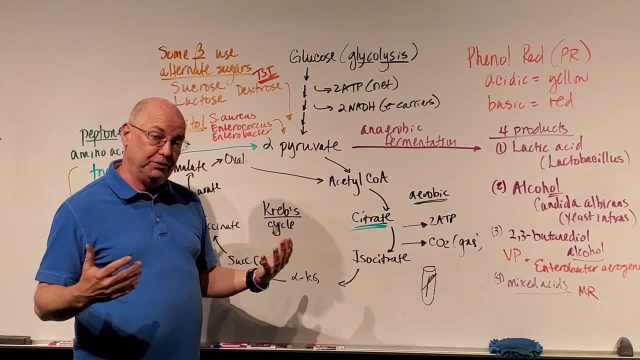 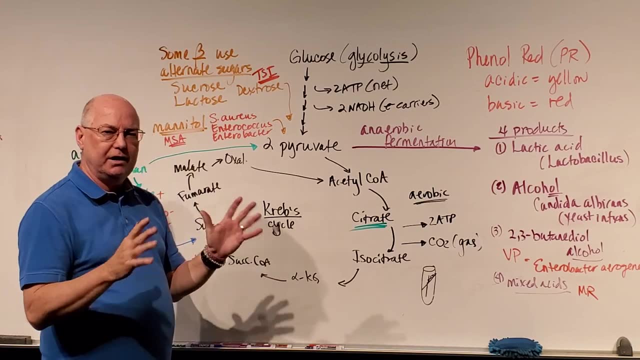 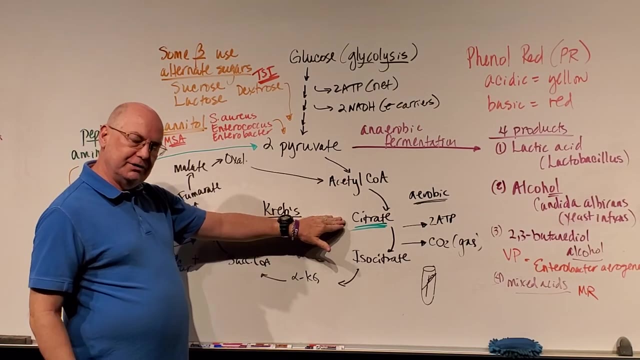 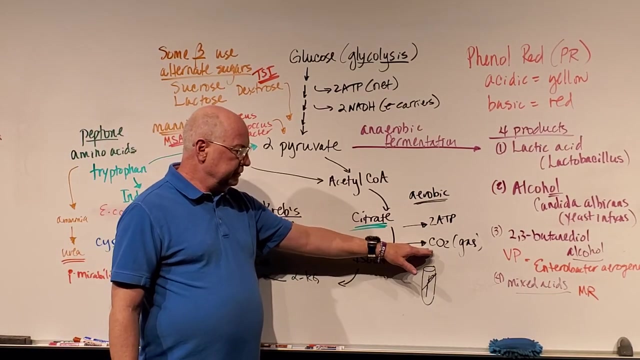 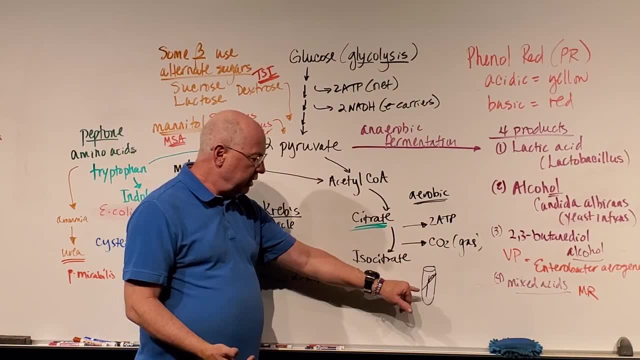 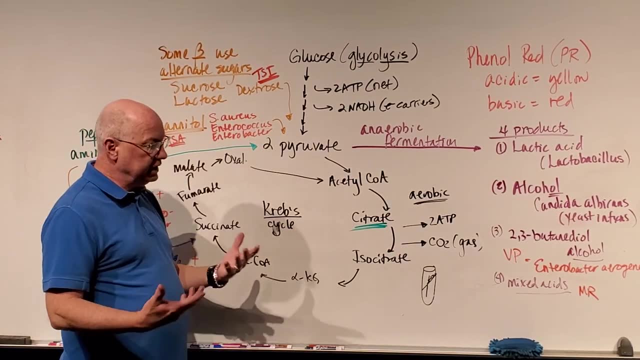 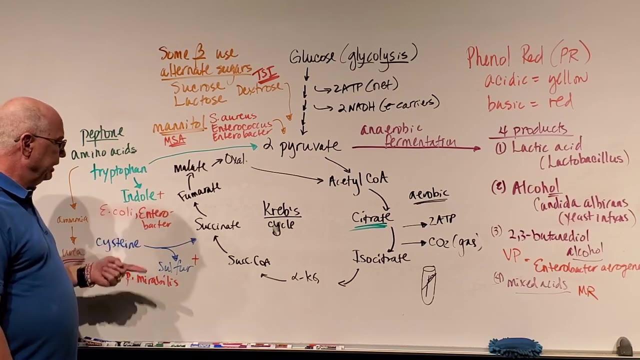 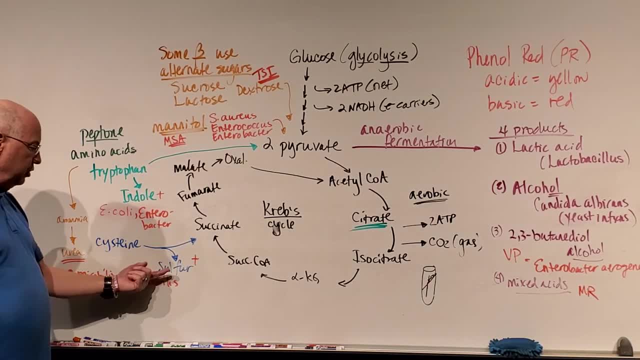 If it turns urea, we get a positive urea test. or positive sulfur test, we get proteus mirabilis, like in the sulfur endo-motility test, the SIM test. okay, And of course we have our PRT. 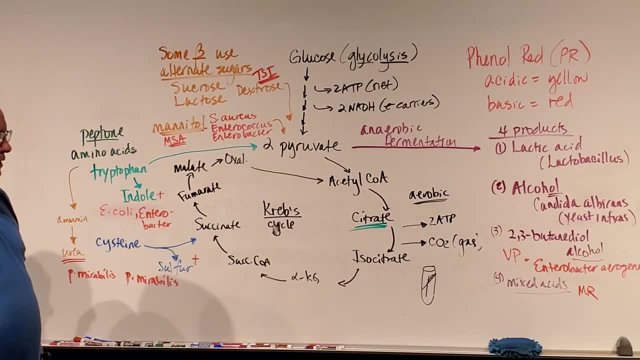 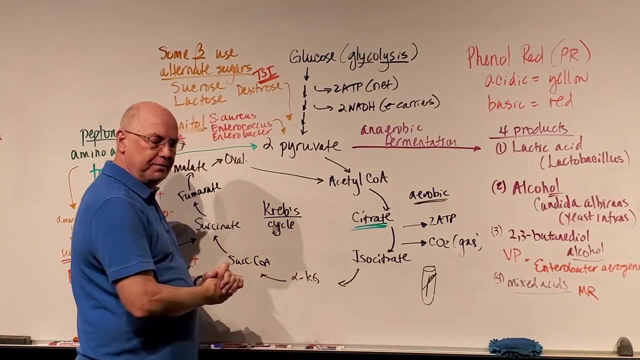 PRL and again. I could go through all the tests over and over and over again, but hopefully this ties what we do in lab with these tests into what we know about bacteria and how we can identify which bacterium is creating an infection. And these are a lot. 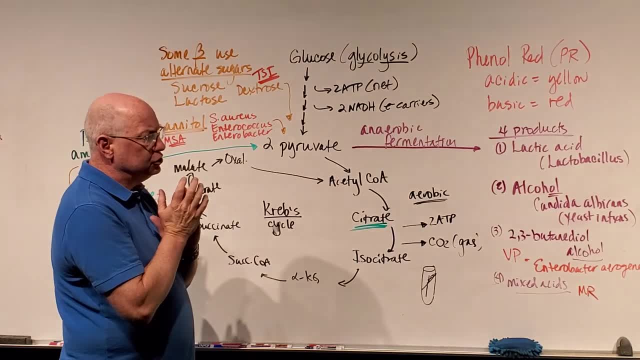 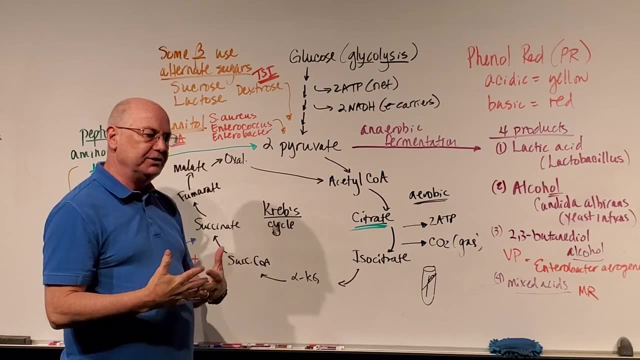 of enterobacter for the most part. so a lot of these tests will tell us a whole lot about which enterobacteria or enteric bacteria are present. a lot of gut bacteria like E coli, the enterococcus enterobacterium. 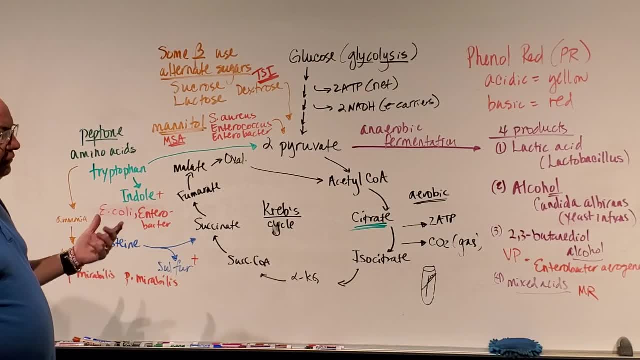 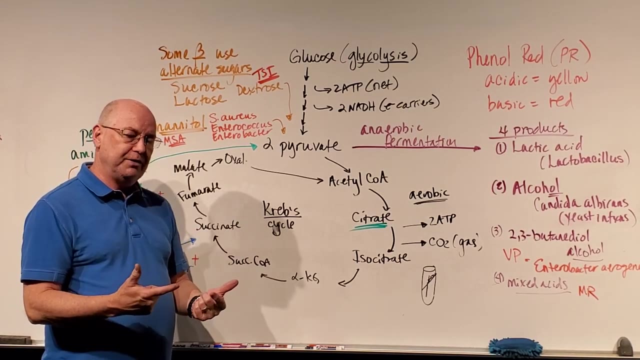 Enterobacter proteus mirabilis and a few others, so shigella salmonella. So anyway, I hope this was informative, or at least I hope I didn't make it worse on you. Maybe I did. You need to go back and watch the video, probably two or three times, and you can see.